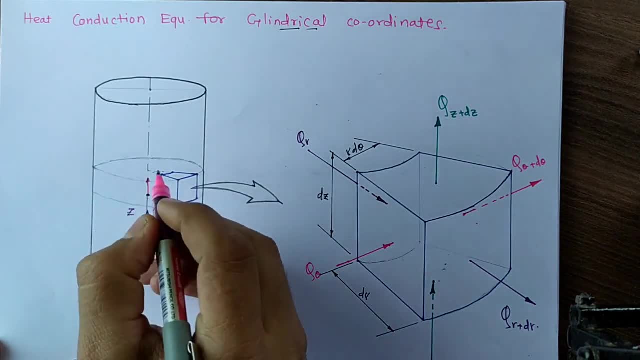 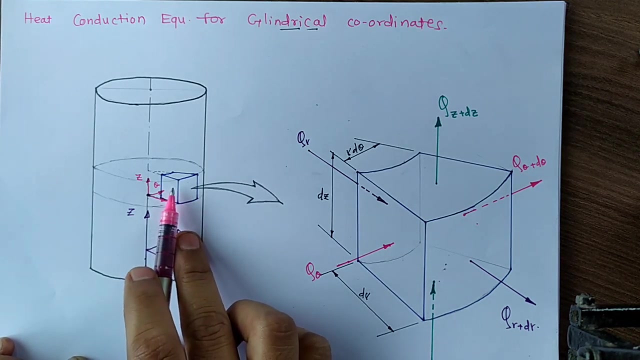 over here. if I draw over, this particular elements is called as a z direction. along the radius, we are having one direction, that is r, and then along this particular curve means like this, we are having theta. so these are three directions we have considered and we have considered small element. this small element, i have made it bigger. 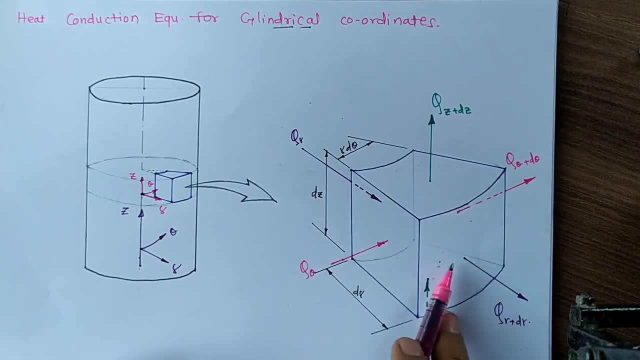 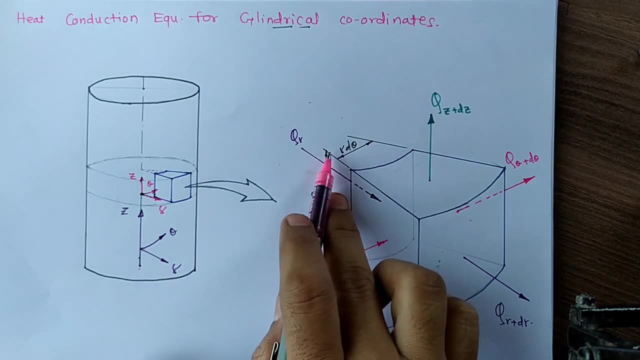 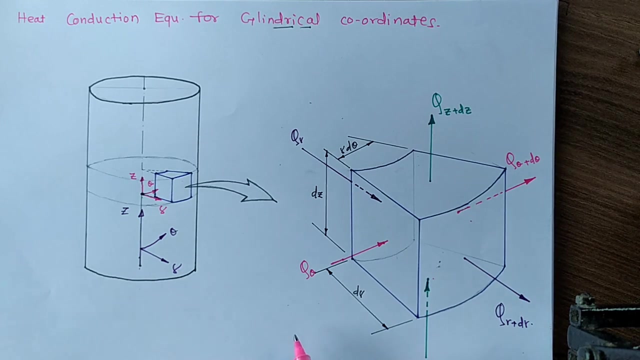 one for your understanding, and we have drawn many elements over here. so if i have to consider these three direction over here, the vertical direction, vertical direction is considered to be z, along the radius. along the radius direction is r and along the curved path it is theta. now you can see. 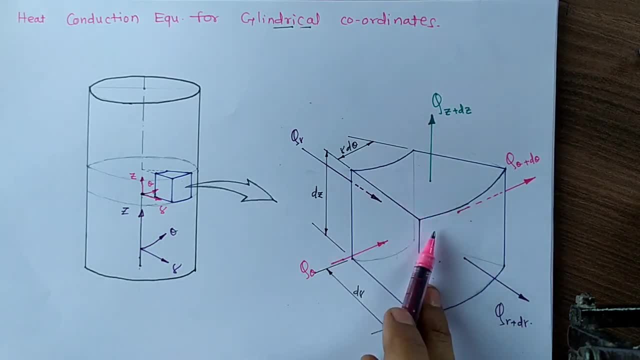 here that this small element, this small element, its dimensions are like this: the vertical dimension, if you consider that is dz, you can see here the vertical dimension is dz along the radius dimension is what dr. so here is dr, we have written it- and this dimension, so it's like a cubical part. 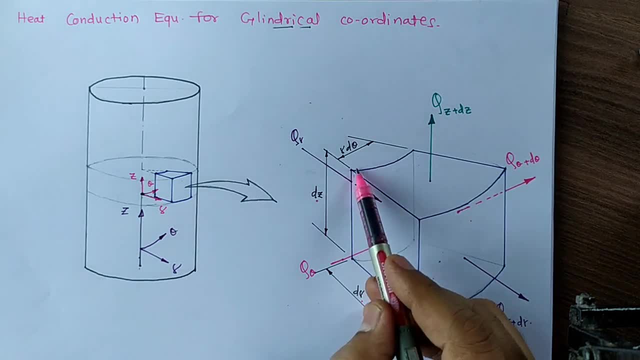 so vertical dimension dz: along the radius it is dr, and this particular curve length is rd theta. we are knowing that angle can be measured by the radius and you will get this particular length. so it is rd theta. so three dimension dz- dr, rd theta. these are the 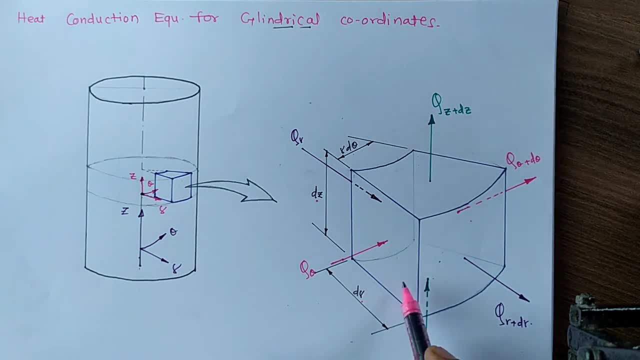 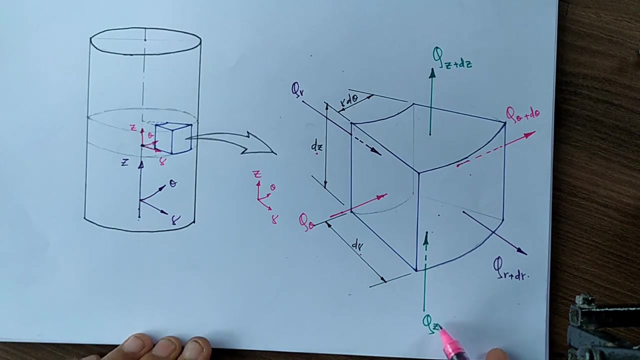 three dimension of this particular cube. now, this element has heat entry and heat exit along the z direction. so z direction, as i told you, z direction is vertical direction. this direction is vertical dimension, along the radius is r and along this is what theta. so along the vertical direction, if you see in the vertical direction the heat entry, heat entry is qz heat. 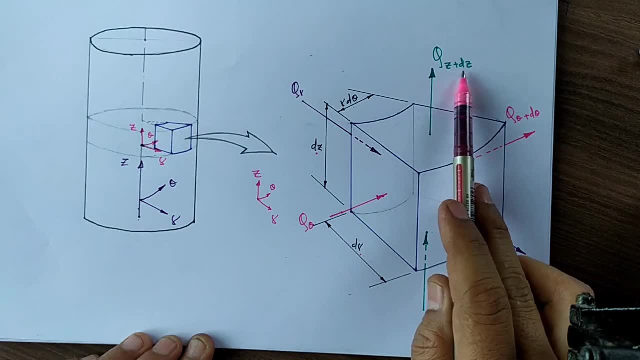 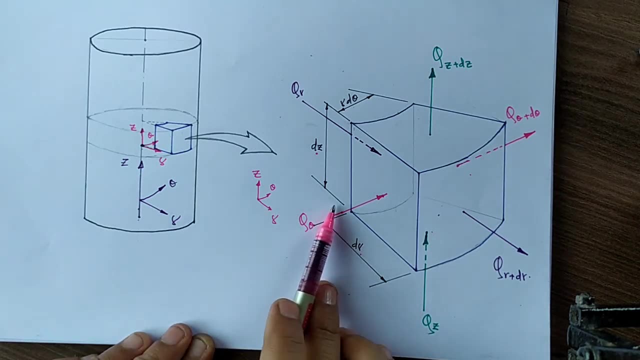 entry is qz and heat exit is what qz plus dz. so this is the entry in z direction, this is exit in z direction along the radius, if you check radial direction, along this radial direction the heat entry is what qr, heat entry is what qr and heat exit is what qr plus dr. okay, so qr is entry and qr. 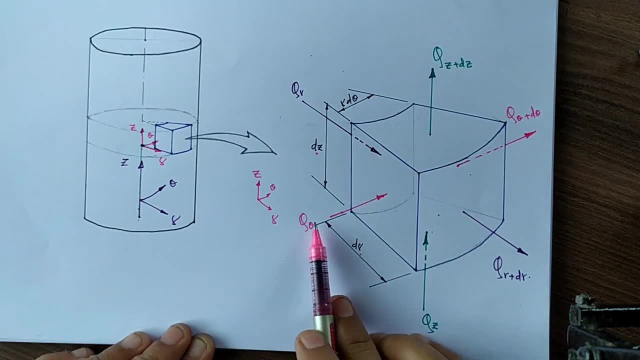 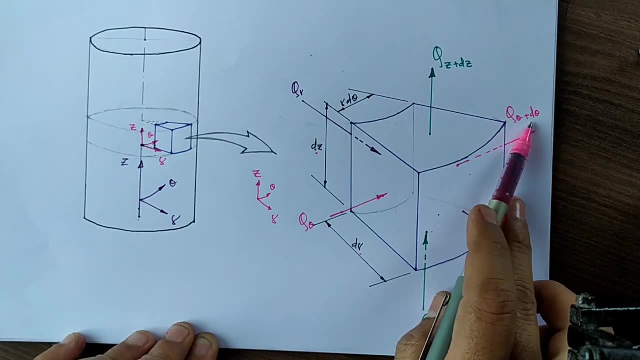 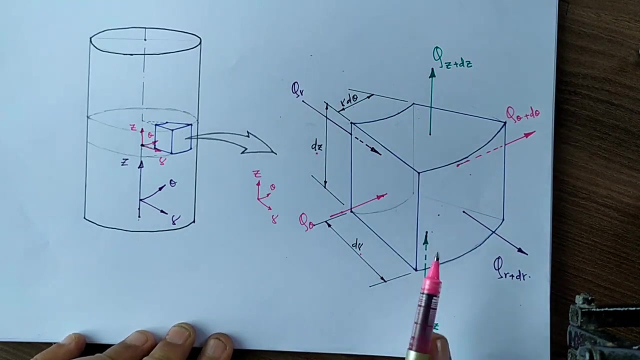 plus dr is exit along the theta direction. theta direction means what? in this direction heat entry is q theta and heat exit is what, q, theta plus d theta. so at the entry it is one like qr and at the exit it is qr plus dr. at the entry qz. exit is qz plus dz. at along the z, along the theta. 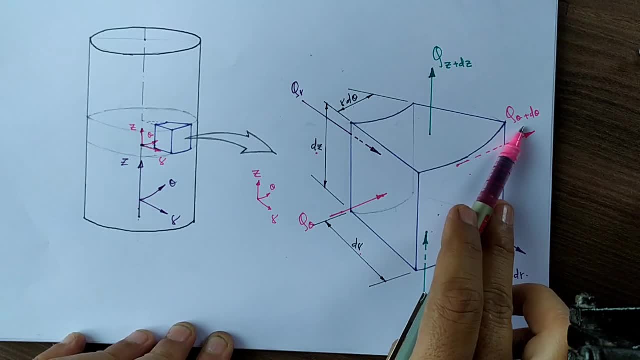 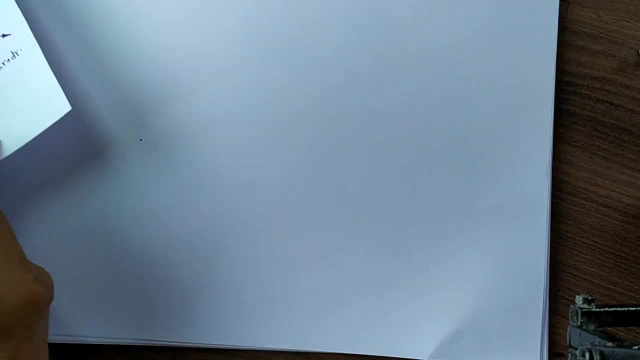 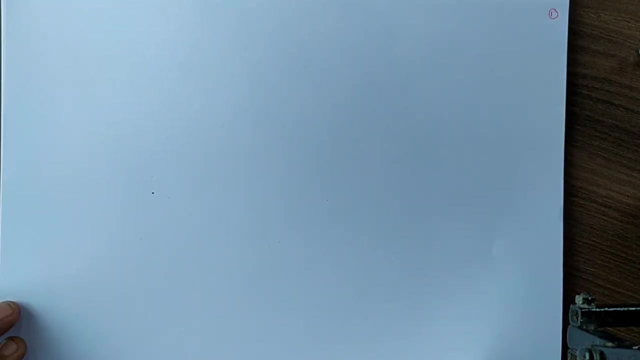 direction. it is q theta and exit is what q theta plus d theta. now for this particular element. let's go first of all by the energy balance equation. i hope you are knowing what is meant by energy balance equation. so we are going to start with energy balance equation. let's write: 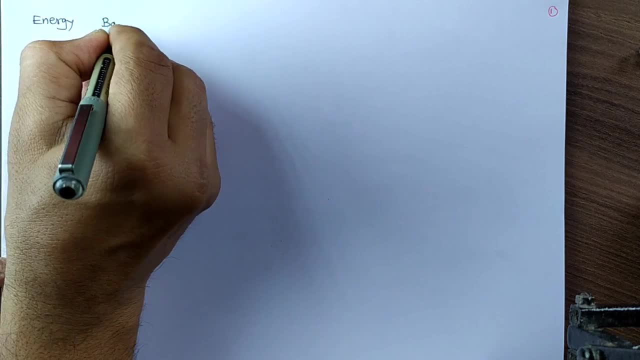 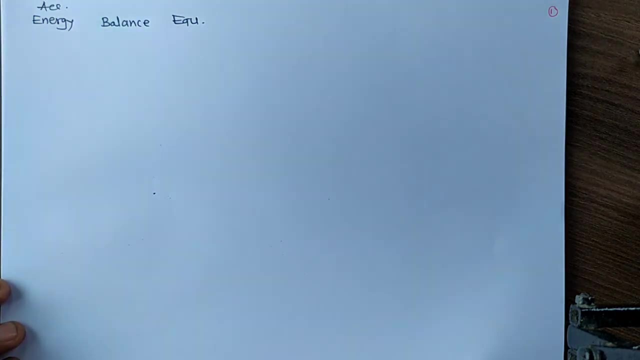 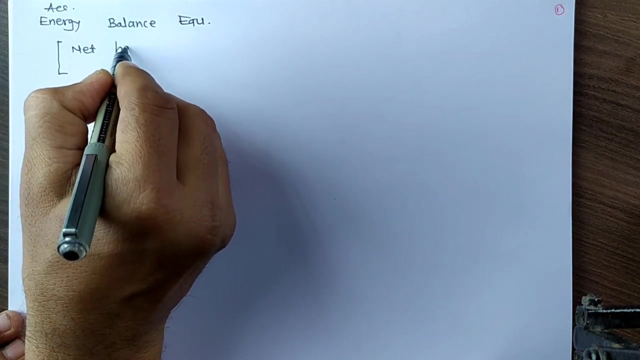 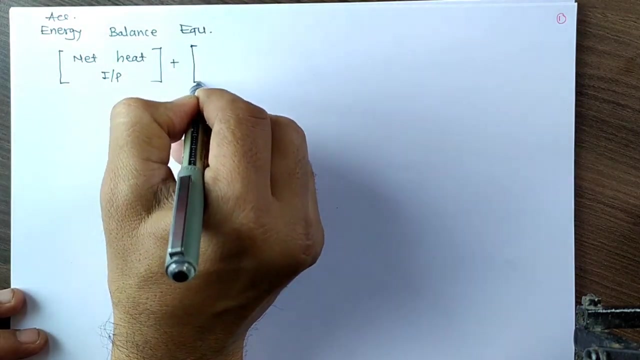 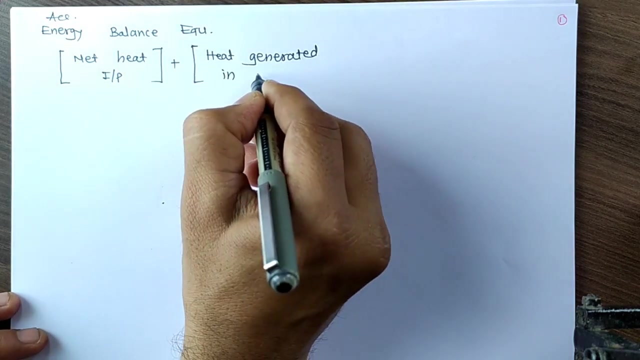 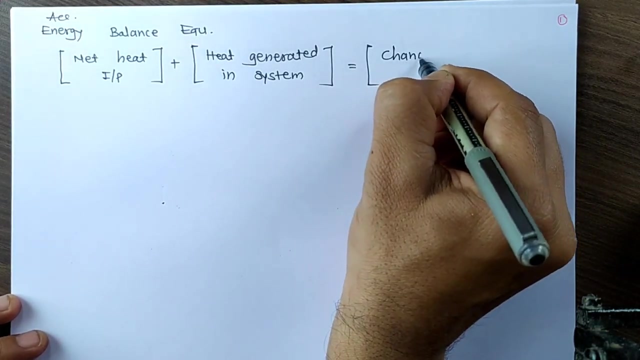 energy balance equation. so according to energy balance equation, according to energy balance equation, we can write as net heat input in the element. let me write net heat input: heat input in the element plus heat generated in the element. heat generated in element, or i can cite, in system is equal to change in internal energy: change in internal. 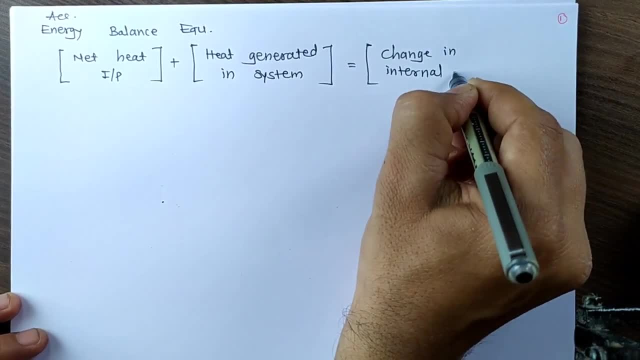 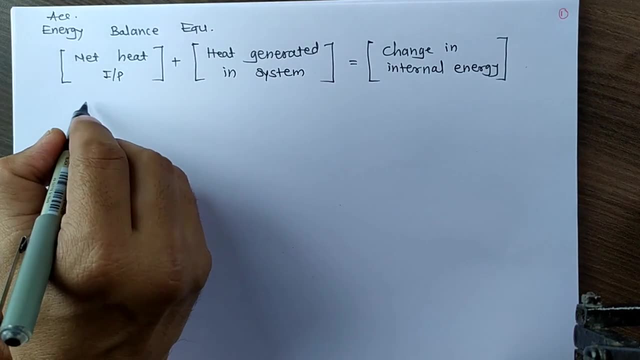 energy. okay, so this is what. this is what the action here is: the change in the equivalence of the energy to energy balance equation. this, this particular first part, that net heat input. i will consider it as a part number one. this is part number one. i am going to consider this as a part number two. 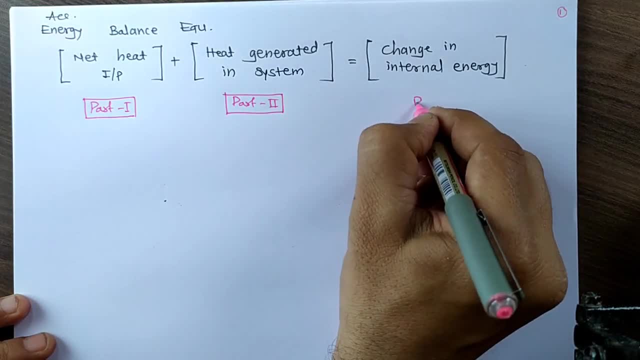 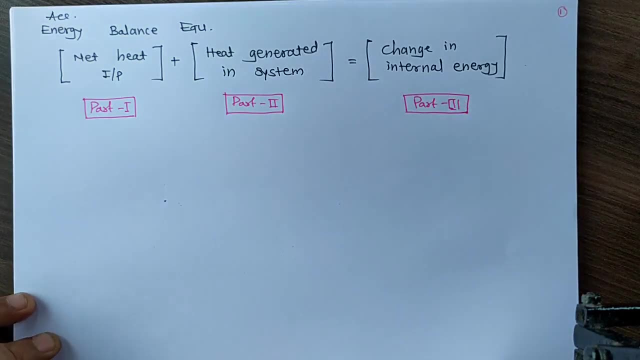 this is part number two, then this is what part number three. so i have made it three part of this particular equation. what i have to do is i have to derive equation for each. so let's consider this is equation number one. let's consider this equation number one. in the equation number one, we 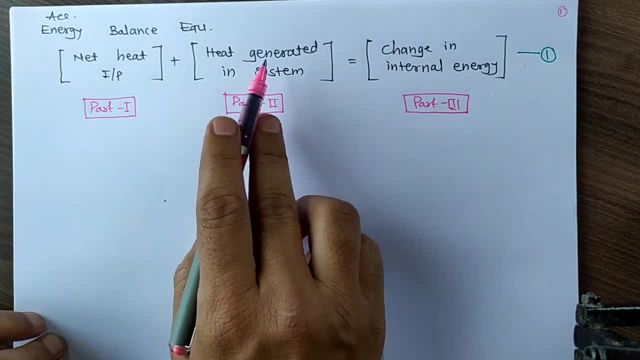 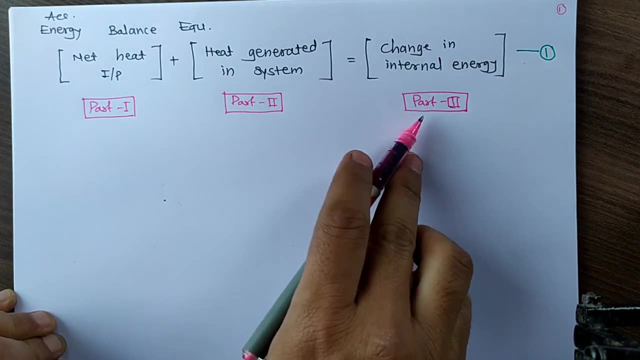 are having three part. part number one is net heat input. part number two is heat generated. part number three is generating internal energy. so what i have to do is i have to derive equation for part one, part two, part three, and then i have to put in the equation number one. so let's proceed for part. 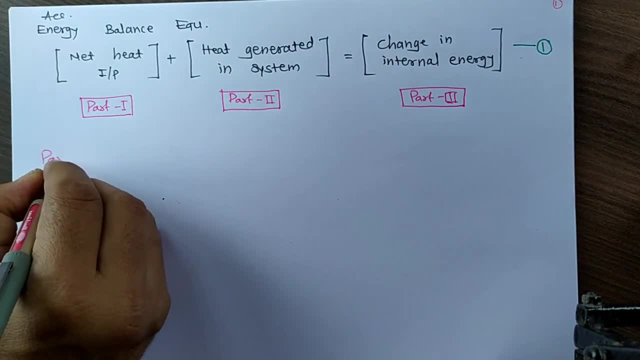 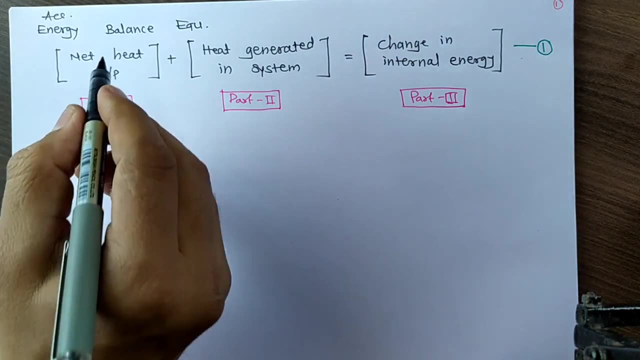 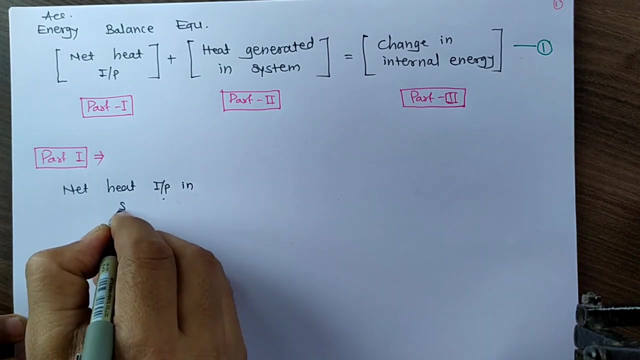 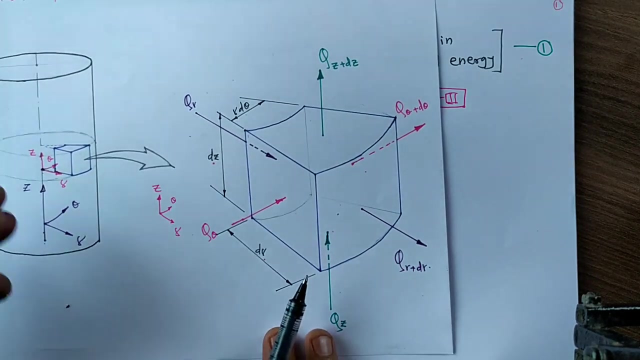 number one. so i am going to derive equation for first of all part number one. so let's go for part number one in detail. what says part number one? net hit input in the element net hit input in system. let's say: okay, so now what is net hit input? if i refer this figure, what is net hit input? you can consider. 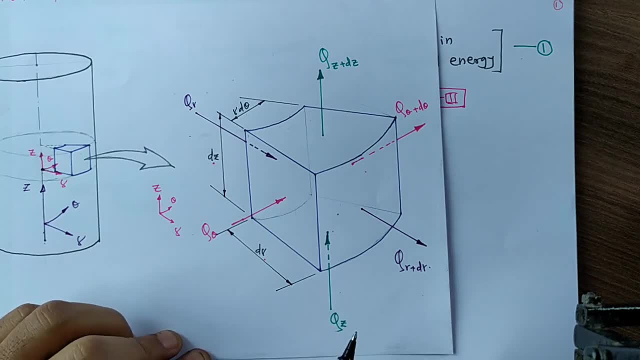 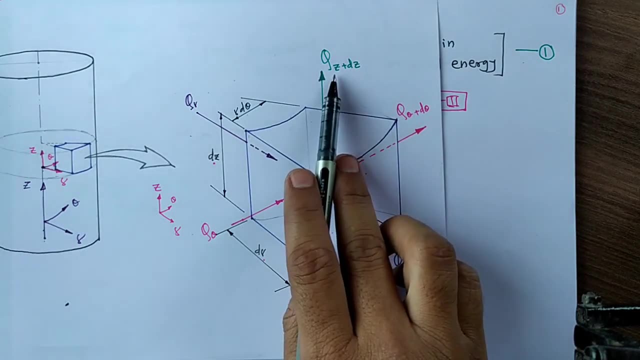 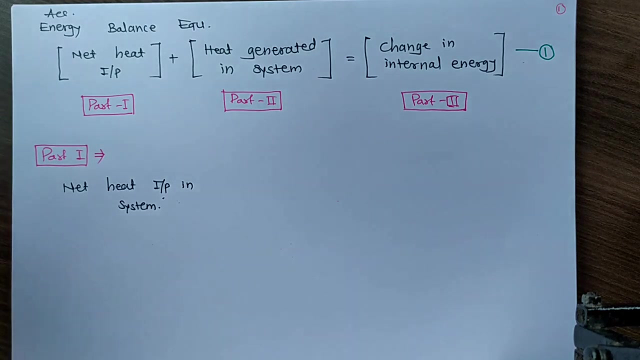 that let's consider a z direction. in z direction, what is net hit input? that is qz minus d, qz plus dz. okay, so that we have to, that we have to know that. if i consider- let me show you one example by which you can understand it in easily- that let's 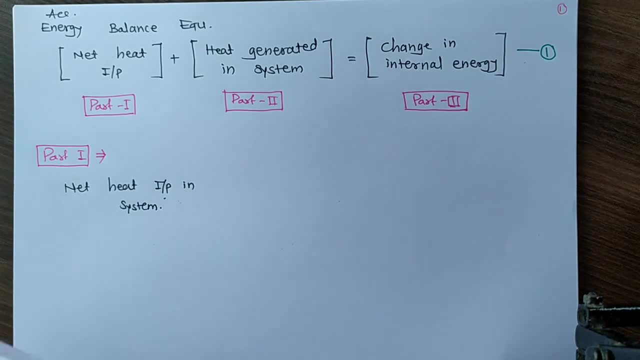 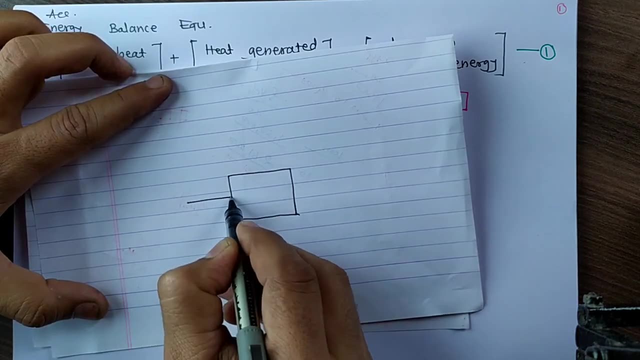 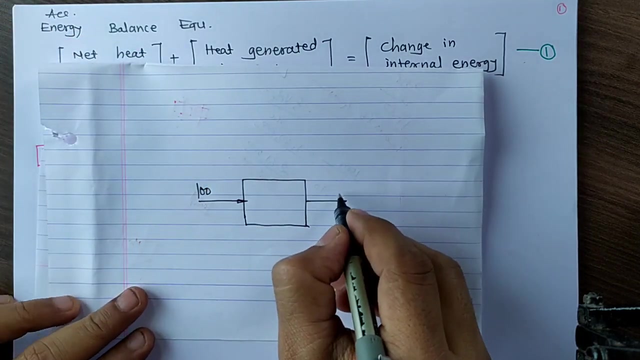 let's consider a system, if i am having this as a system. now to this particular system, if i consider there is some heat input and there is some heat output. let's consider 100 unit of heat is input. 100 unit of heat is input you and going outside is 80. So input is what 100.. Going outside is 80. So what is net heat input? 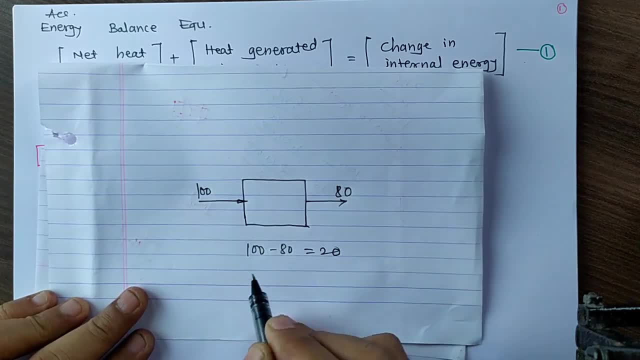 You can say 100 minus 80.. 100 minus 80 is 20, is the heat input. Similarly, if I consider this is qz and if I consider qz plus dz, So what is net heat input? in z direction It will become qz minus. 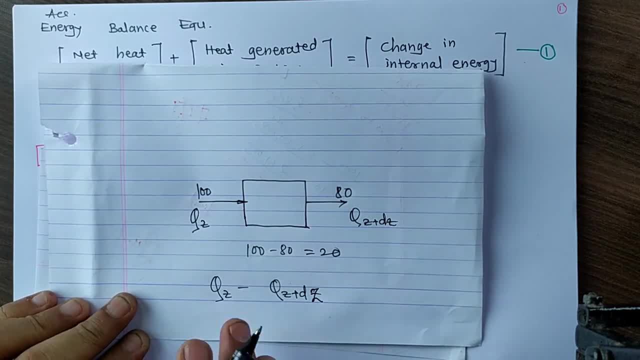 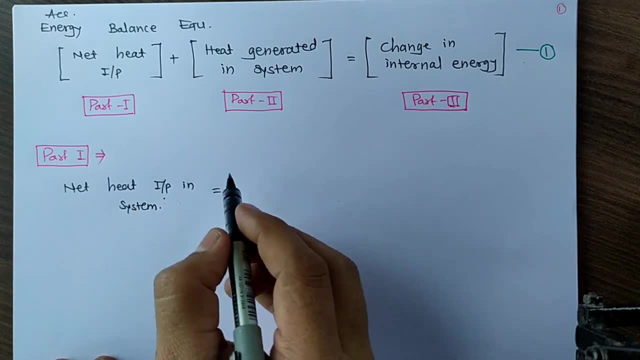 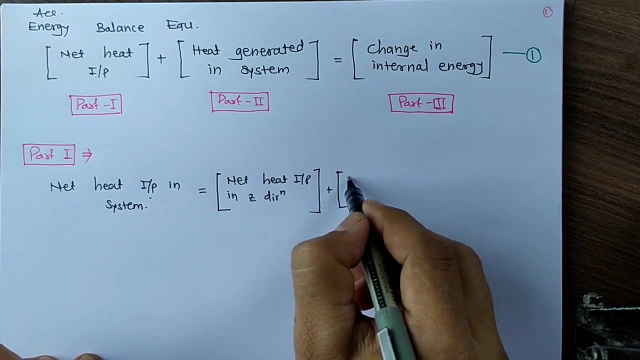 qz plus dz, That is in z direction. So applying this principle over here we can write net heat input in all direction. Okay, we have to consider all direction. So first of all I will write it: net heat input: net heat input in z direction plus net heat input. 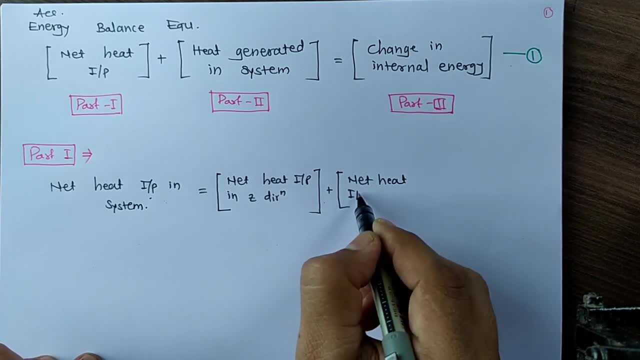 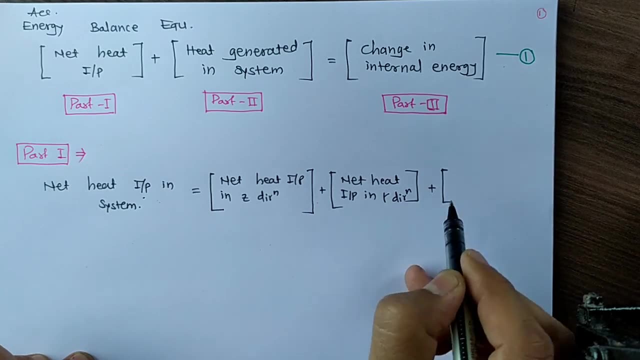 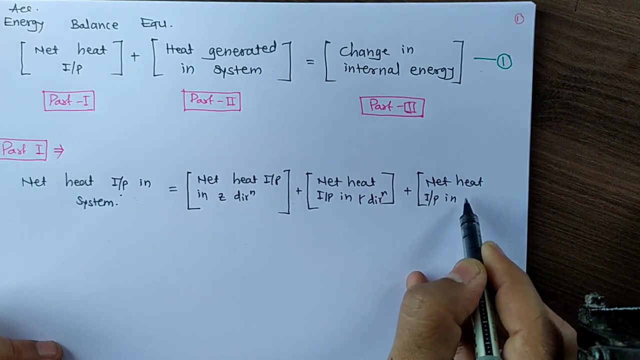 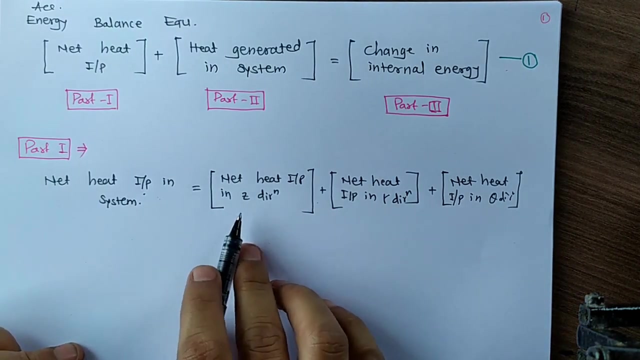 input in r direction. This is in r direction plus net heat input in net heat input in theta direction, So that we are knowing that three directions already we have discussed. For the cylindrical there are three directions: Z direction, r direction, theta. 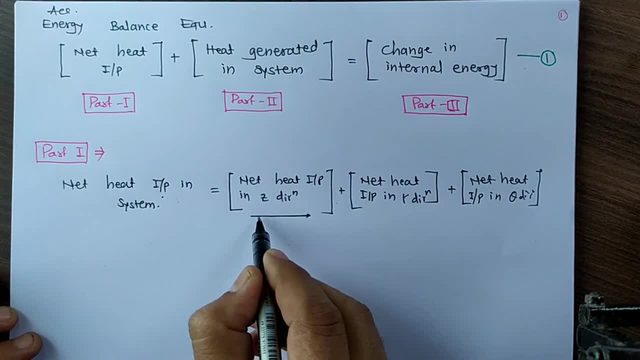 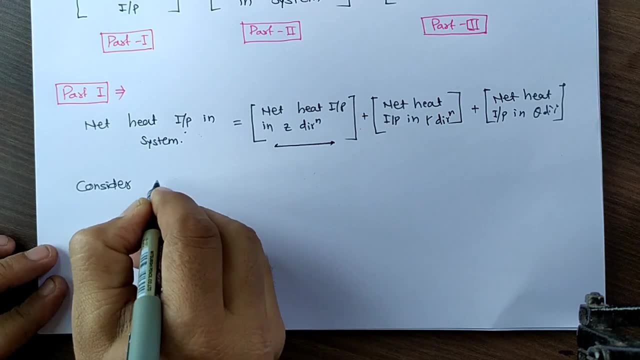 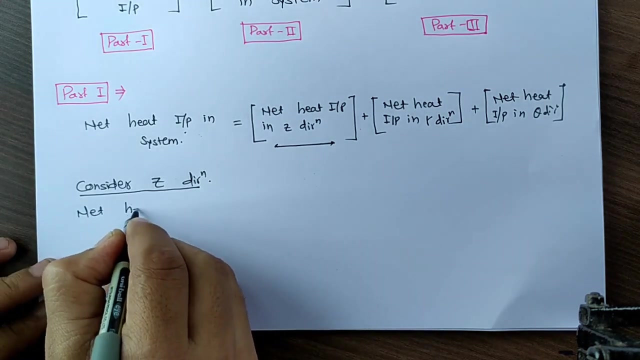 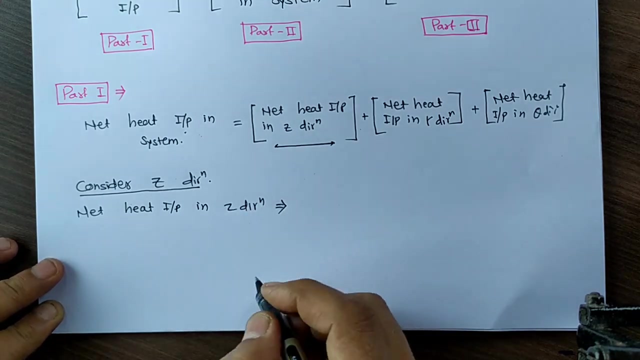 direction. Now let us go first of all for the z direction. I am going to derive equation for z direction. Let me write that. consider z direction. So in a z direction, heat input in z direction. So one by one I am going for all the directions. So first of all, 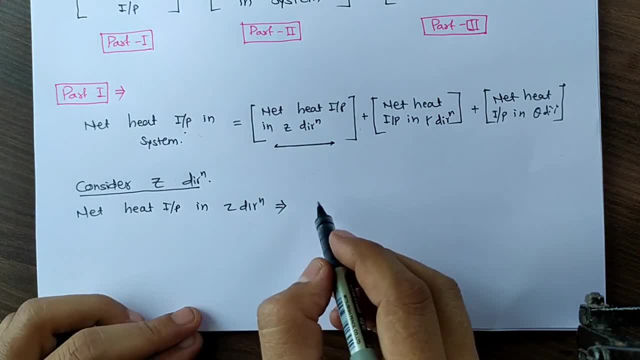 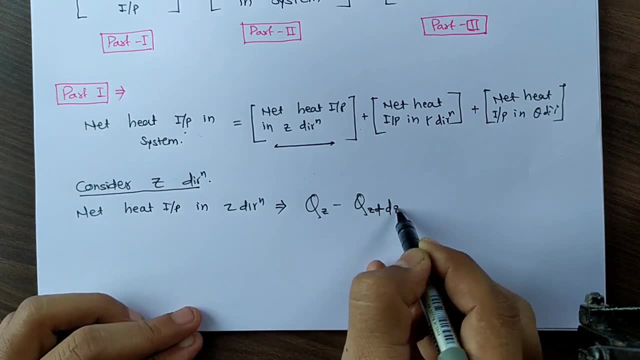 I have considered z direction In z direction, what is the net input? Net heat input is, as I told you example, qz minus qz plus dz. That is the net heat input. in z direction. This is the heat input. qz is. 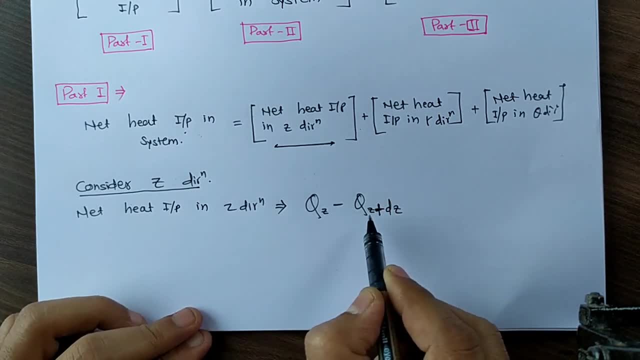 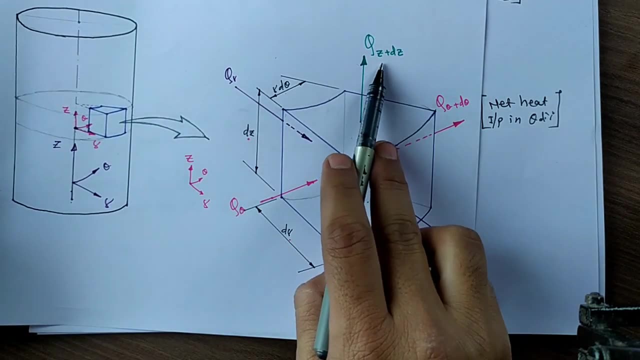 heat input and qz plus dz is heat output in z direction. Okay, so you can see this particular figure now that what is net heat input in z direction, That is qz minus qz plus dz, So this is qz. What is output in z direction is qz plus dz, So this minus this will be in z direction This. 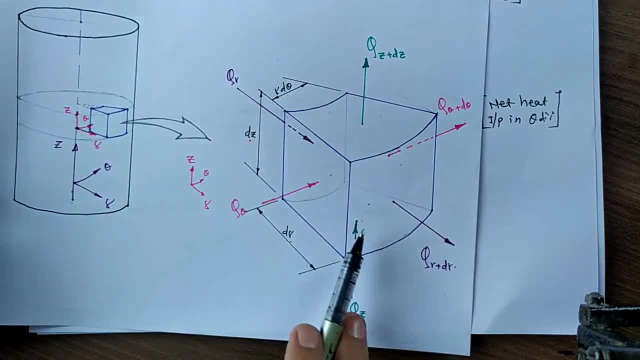 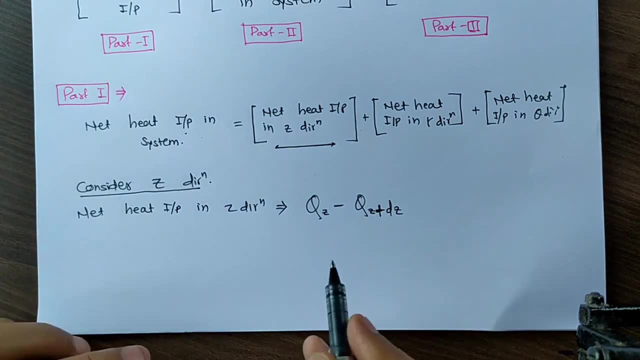 minus, this will be in theta direction, and qr minus, qr plus dr is in r direction. Okay, so I am in z direction now. Now, when we write in z direction, we have got qz minus, qz plus dz. Now let us. 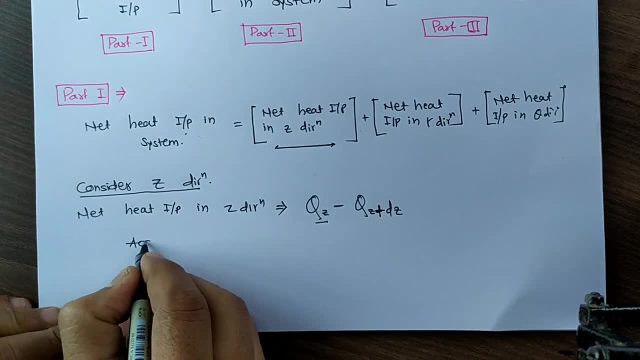 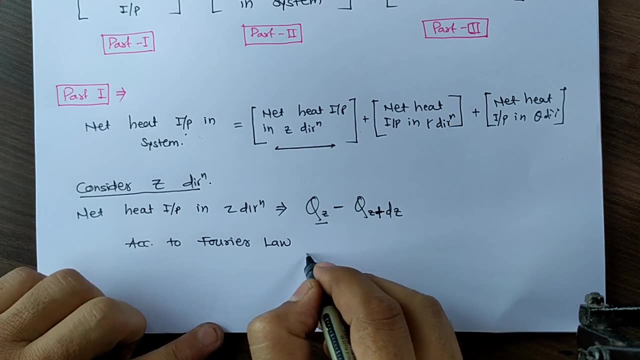 consider qz. I want to write equation for qz. So according to Fourier law that we are knowing What is Fourier law, According to Fourier law, I can write as qz: What is Fourier law we are knowing? The Fourier law is: 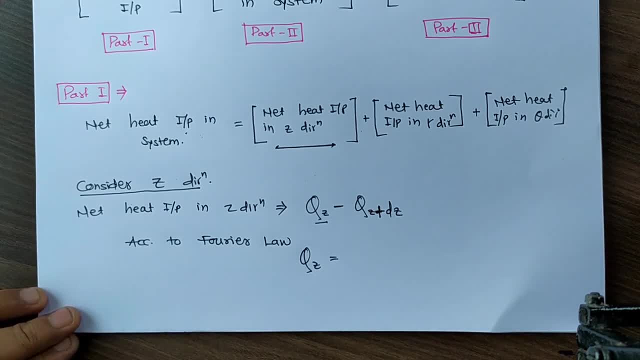 minus. I will write over here that Fourier law. The Fourier law is what q is equal to minus ka, dt by dx, if it is in x direction. If it is in x direction, Now we are in a z direction. So 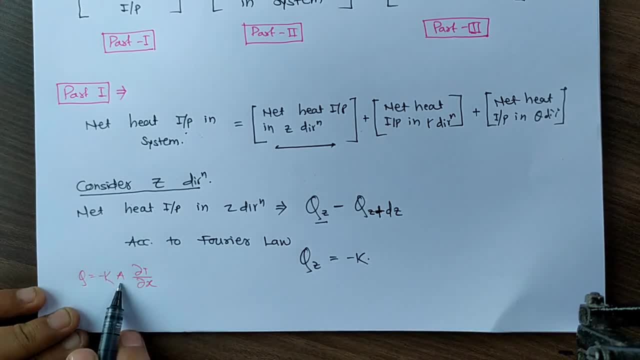 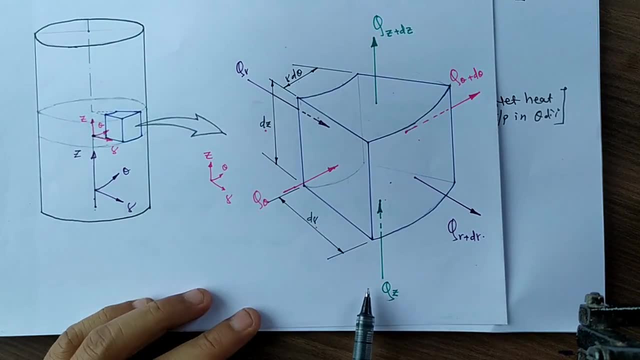 for z direction. it will become minus k into a. is what Perpendicular area? Perpendicular area in z direction? So if you check this particular figure, you can see that it is in z direction. What is the perpendicular area in z direction? So, if it is moving in this direction? so this: 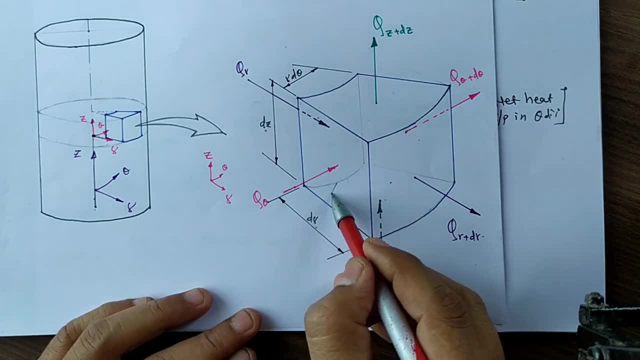 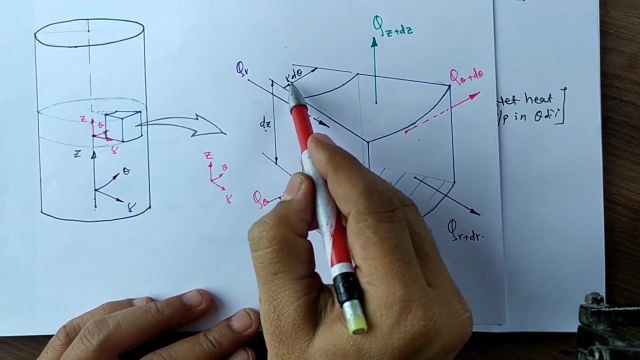 downside area. this particular down area is the perpendicular area for z direction. What is its dimension or what is its area? Area will become dr into this curve. What is this curve? This curve is rd theta, So dr, rd theta or rd theta dr. That will be what. That will be the perpendicular area. 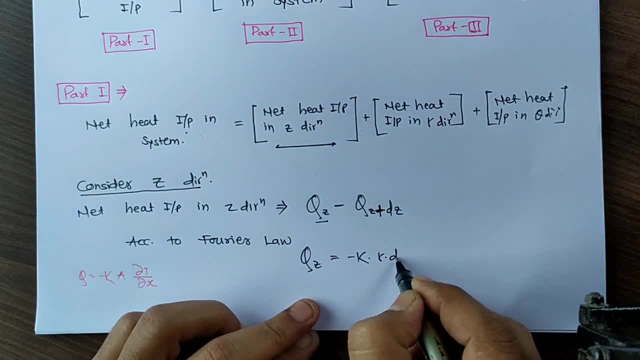 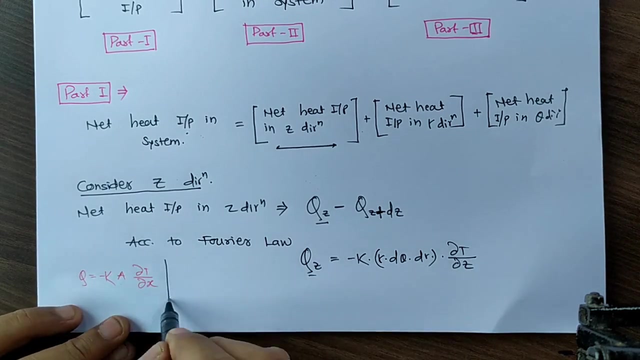 in z direction. So let me write rd theta into dr, That is the perpendicular area into change in temperature with respect to z direction. So that is dou t by dou z. That is the equation. for what? Equation for, Equation for. 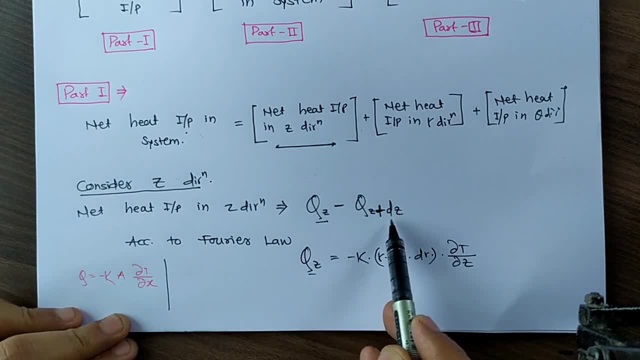 qz. Now I have to write equation for qz plus dz. So for that purpose we have to refer the Taylor series. according to Taylor series that you might be studied in the mathematics somewhere in the M2 or M3. So 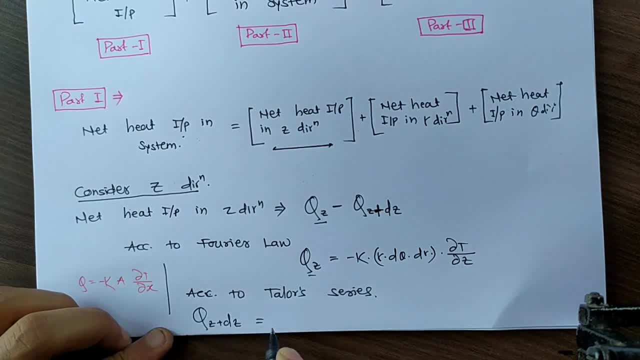 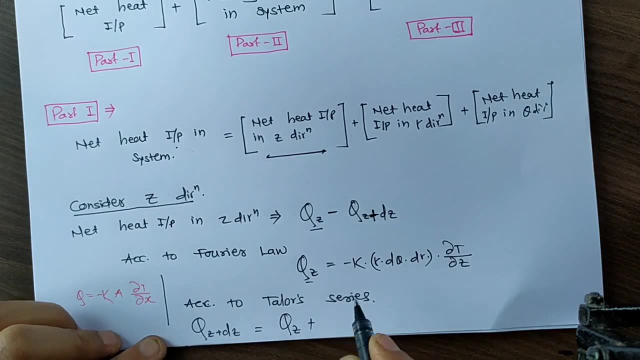 there I can write that qz plus dz is equal to qz plus dz is equal to what. This can be expanded, that qz plus daba of daba z, qz dz. one factorial, That is first term Plus second term, is daba square. 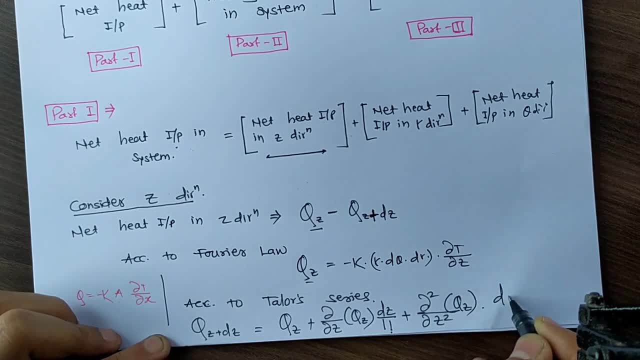 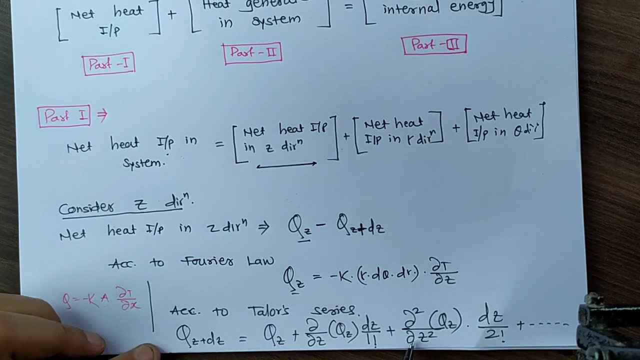 daba, z-square, qz, dz, two factorial and it will to go on. So, generally, what is done here? This dz element or dz dimension, is very, very small. It is square, It will become more small And here it will become 2 factorial. So this onward term, This onward term is generally. 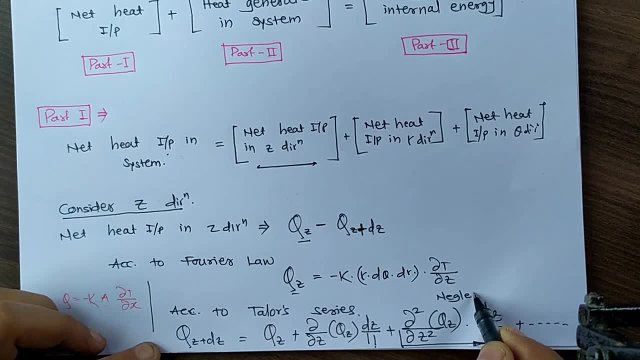 neglected. This onward term is generally neglected. So if you neglect it, then what will become an equation? Let me show you. I am going to give a zero answer. I am going to determine a negative value, So I am going to have a negative equation. Say here: negative 0.5 to. 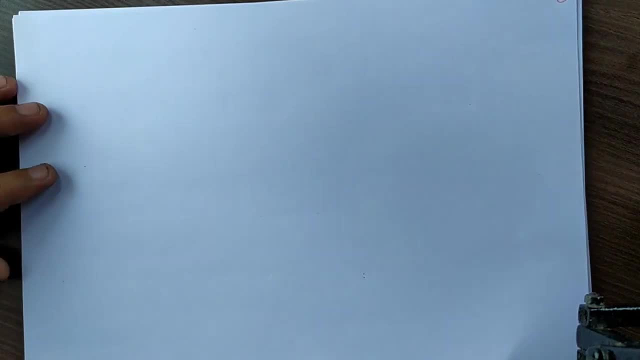 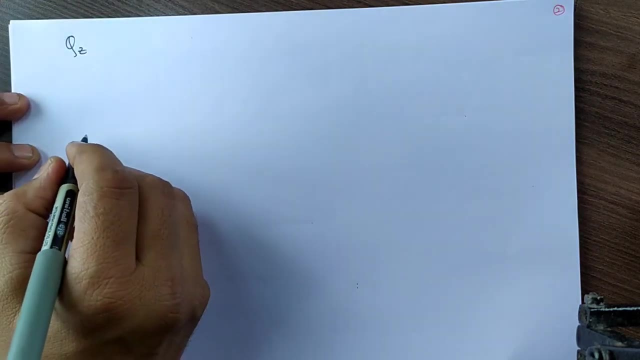 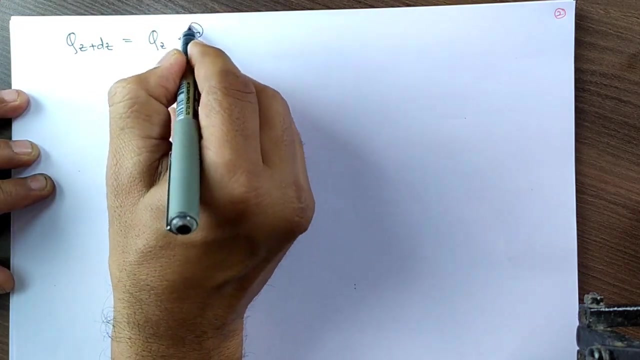 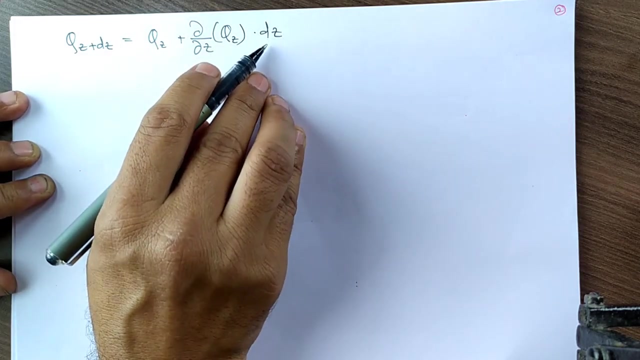 you the equation for this. after taylor series expansion, the equation for the equation for z direction will become as like this: qz qz plus dz is equal to is equal to qz plus daba of daba z, qz dz- further term we have neglected- divided by one factorial. one factorial is one that we are: 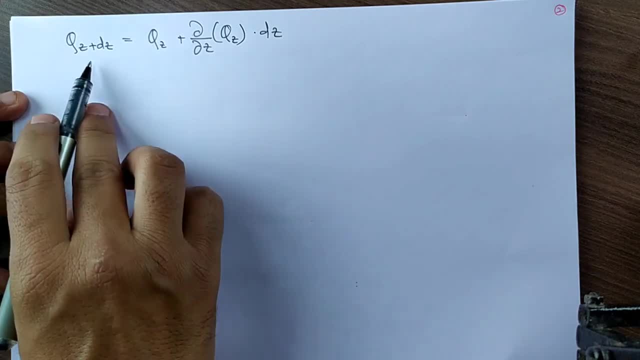 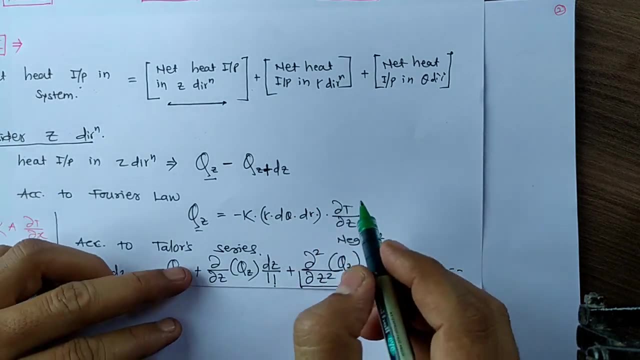 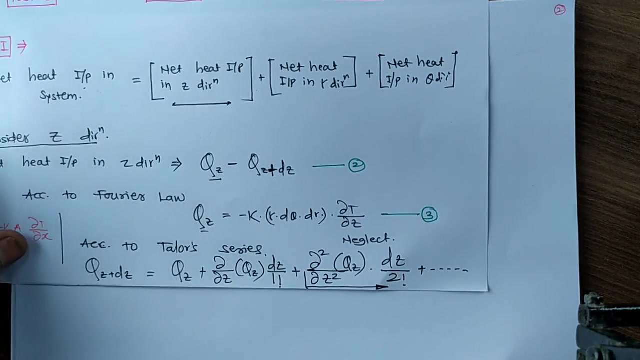 knowing it. now we are knowing the equation for qz and qz plus dz. these are two equation. we are knowing it. okay, so here what i will give. i will give this as equation number two, this as equation number three, because we have to take a reference of this, and then i will put this as equation number. 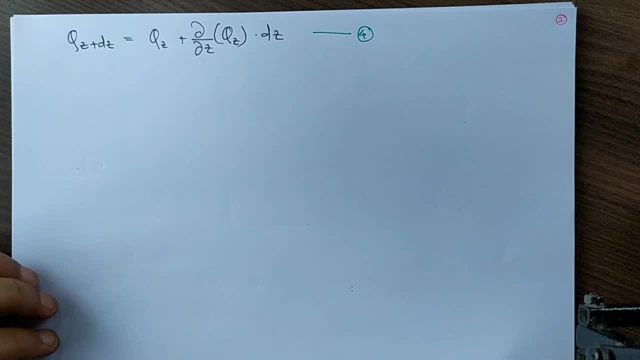 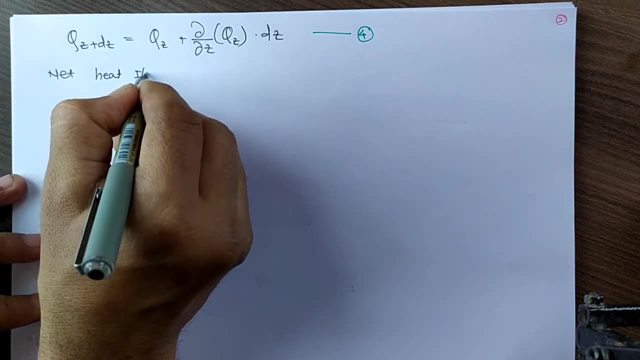 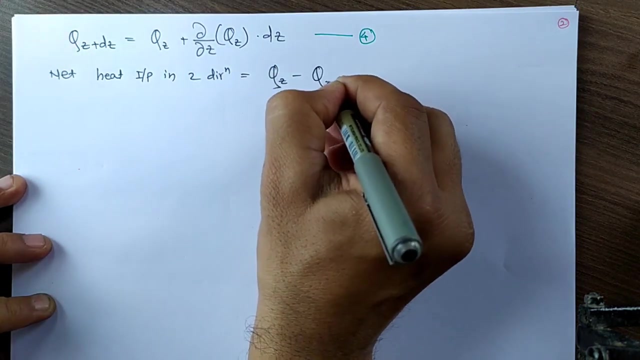 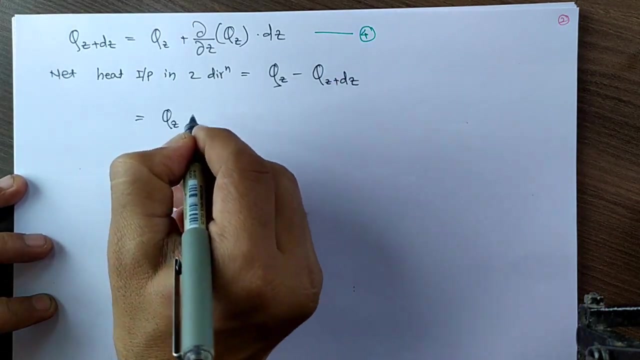 four. this is equation number four. now finally, finally, what will become net heat input in z direction? net heat input in z direction will become what? qz minus qz plus dz. this equation already we have, knowing it. let's put this equation number four in this one, so it will become qz minus qz plus dz. is what this? 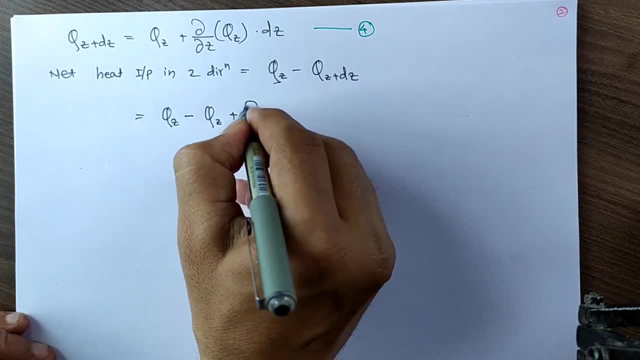 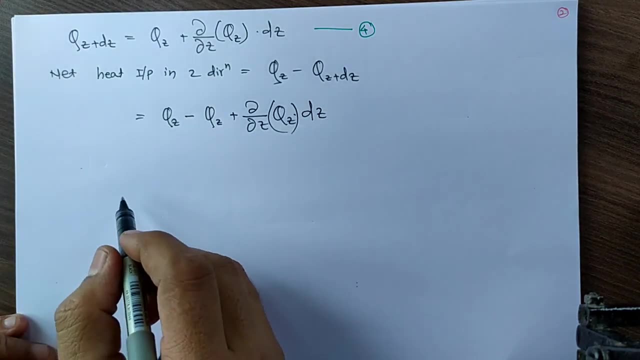 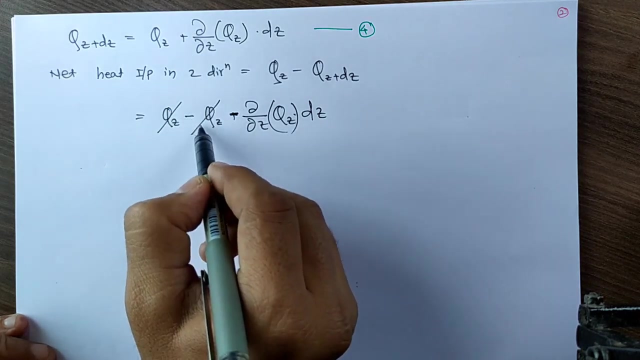 one, so it will become qz plus daba of daba z, qz dz. so if i simplify this, if i simplify this, this qz and qz will get cancelled. and when it is minus sign, so this will also become minus, because this minus into bracket, if i put it, we have removed the bracket. that's why it will become minus sign. 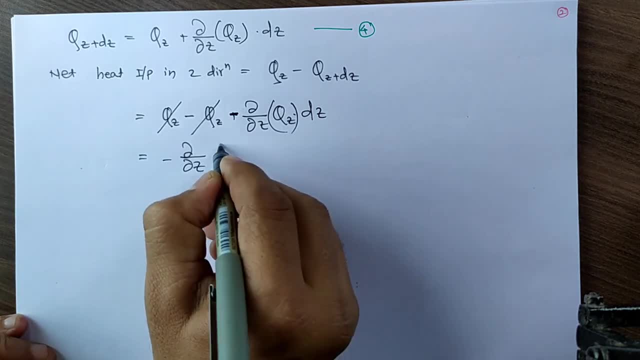 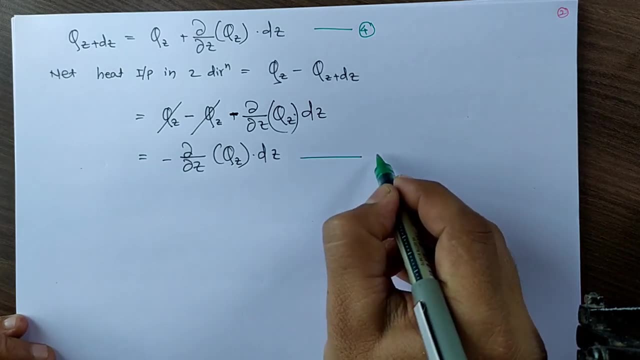 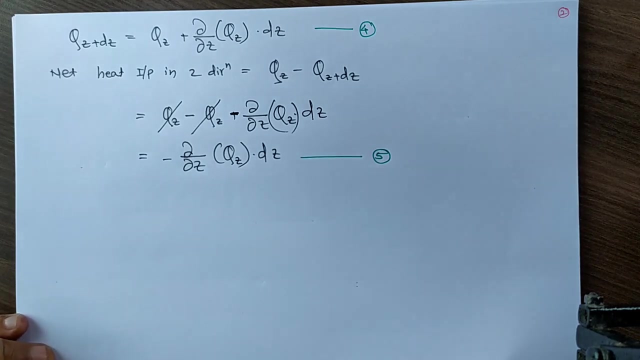 so what? we have got an equation minus daba of daba, z, qz, dz. that's the equation. that's the equation for net heat input in z direction. let me consider: this is equation number five. this is the equation number five we have got, that is heat inputting z direction. now heat input. 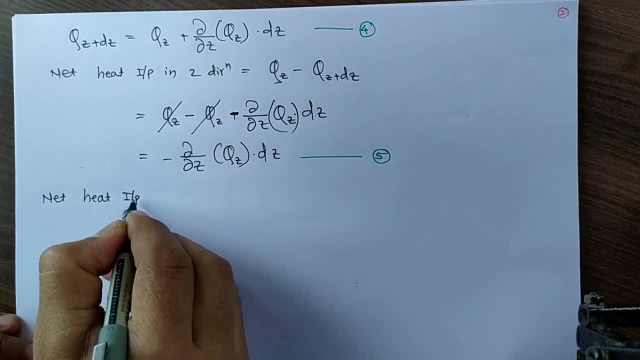 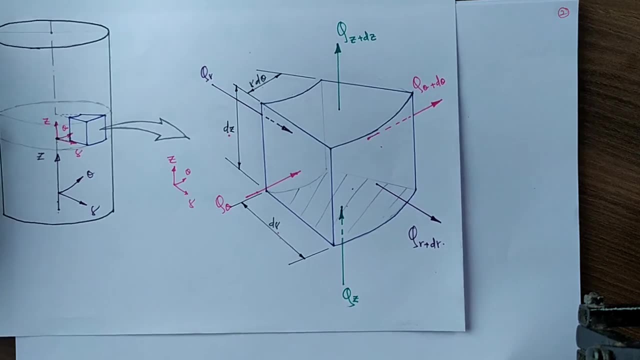 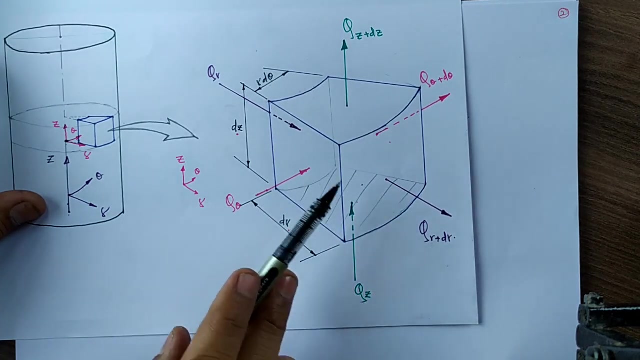 net heat input in r direction. we are going for one by one in r direction. what is in r direction? if you see this figure once again, all direction, in which one we have seen here: r direction. so in this direction heat input is qr, output is qr plus dr. so net heat input is qr minus qr plus dr. okay, that's. 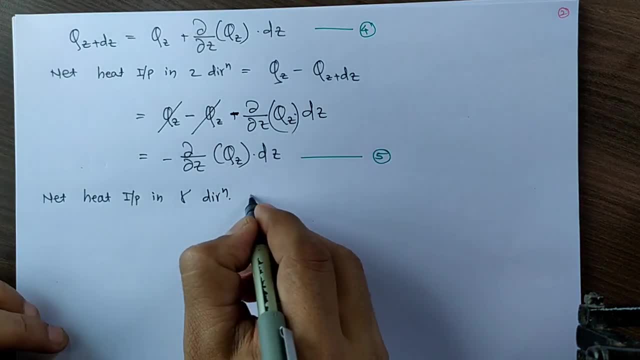 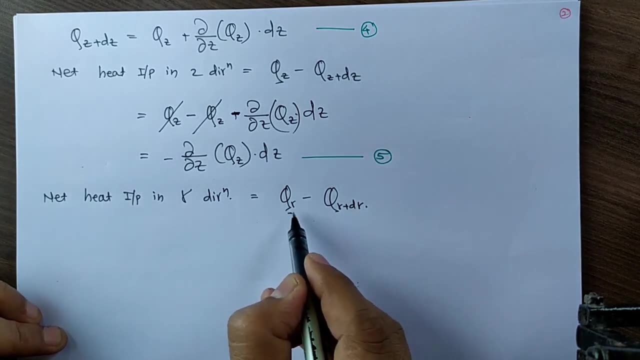 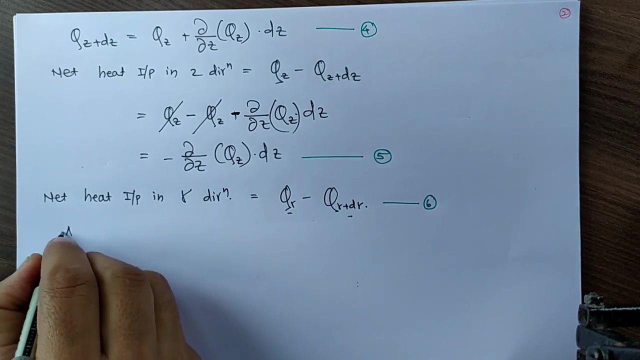 the net heat input. okay, so we have to write here: net heat input: r direction is qr minus qr plus dr. now, once again, we have to write equation for this and this: let me consider this as equation number six. this is equation number six, so according to same, what we have done for previous, according to: 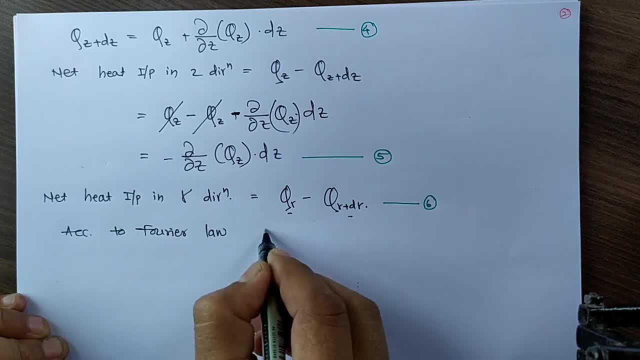 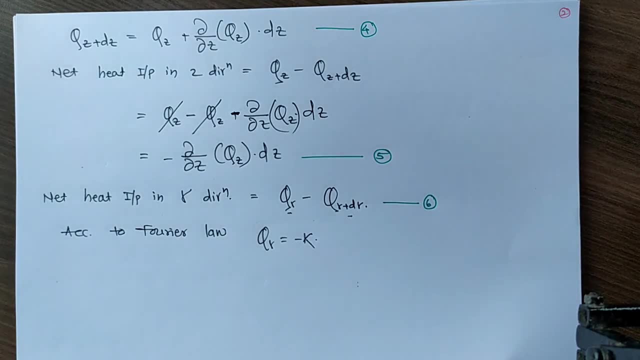 fourier law. according to fourier law, we can write a qr. qr is minus k a. dt by dr will become so it's minus k. a is a perpendicular area in r direction. now let's check what is perpendicular in r direction. what is our direction? that we have seen is: this is our direction. 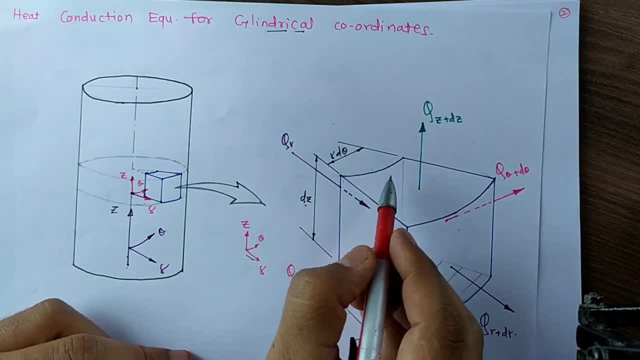 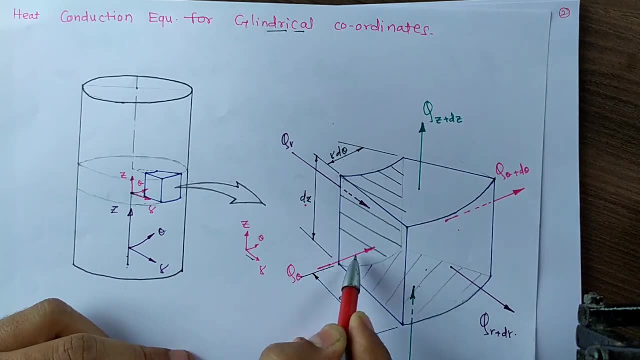 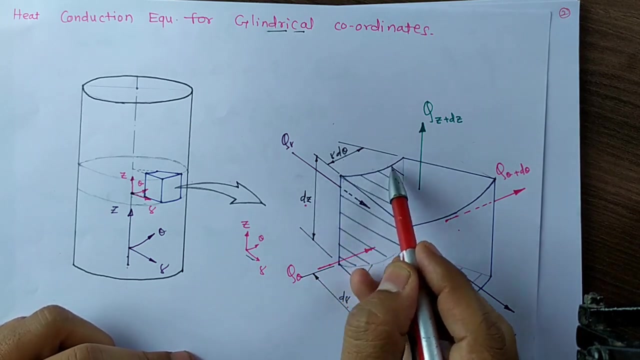 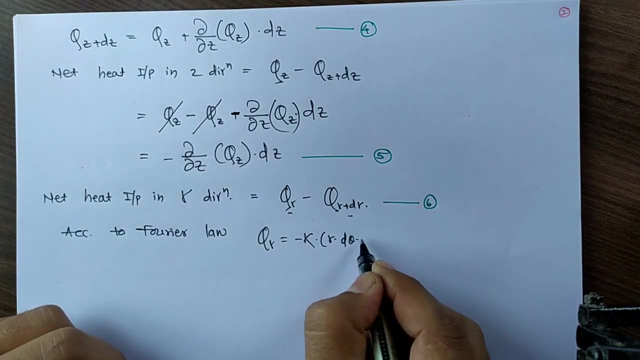 in our direction. what is perpendicular area? now, the perpendicular area is this one, check, this is the perpendicular area in r direction. okay, this is perpendicular. now what is its dimension? vertical dimension is dz, and this dimension is what r d theta? so area will become r d theta into d z. okay, so it will become r d theta into dz. is perpendicular area. 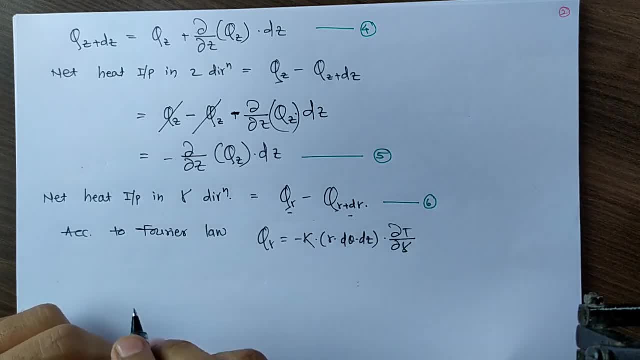 change in temperature with respect to r direction. so it will become d, it will become dr. so that's the, that's the what: heat conduction in r direction. now let's expand qr plus dr. qr plus dr according to taylor series. according to taylor series. now i will not write. 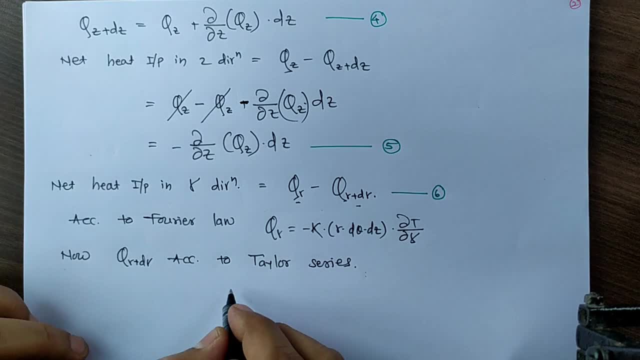 complete taylor series. i will write in short, after neglecting the terms: qr plus dr, we'll get qr plus d of d, r, qr, dr. that's the taylor series. okay, so now we have got this equation. this equation let's consider. this equation is equation number seven. 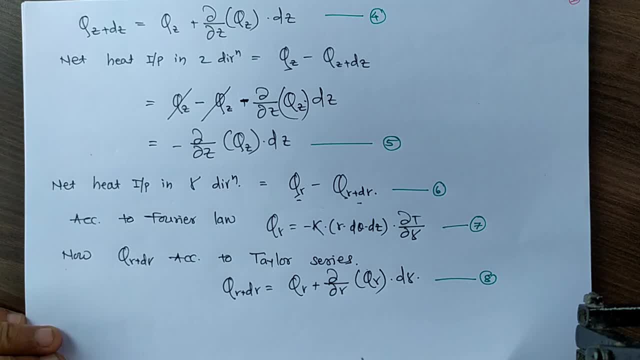 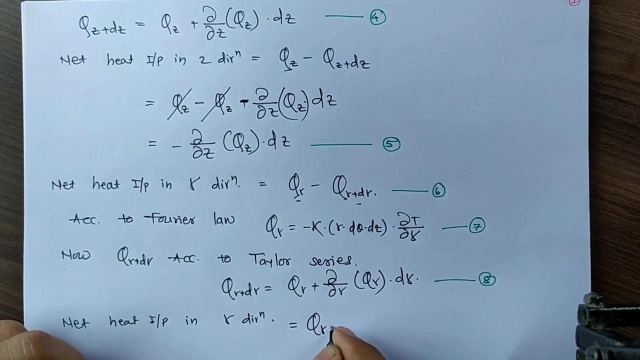 this equation is equation number eight. we have got it. now let me write: net heat input in our direction. this equation, this equation number six: net heat input in r direction. so So what we get in R direction, which is QR minus, QR plus DR. What is QR plus DR? 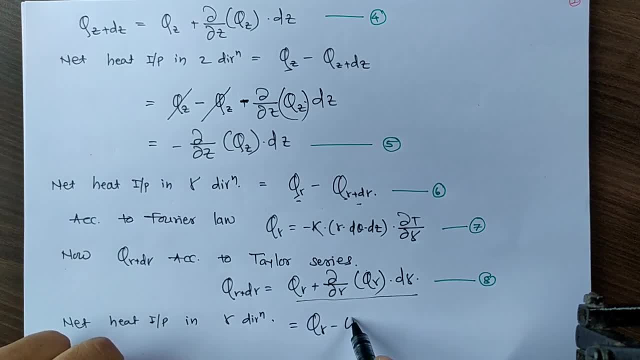 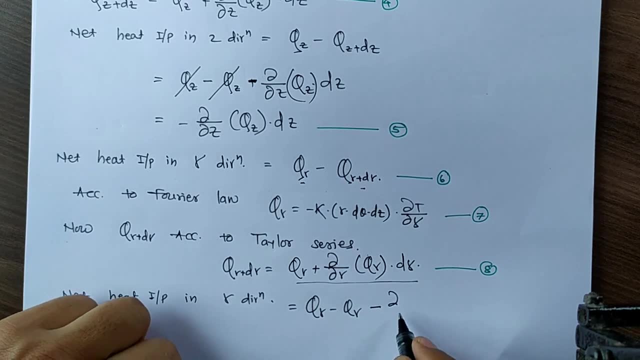 QR plus DR. is this Taylor series right, So minus QR, and when we multiply here minus, so this will also become minus Minus, minus daba by daba R QR DR, That's we get QR. QR will get cancelled. 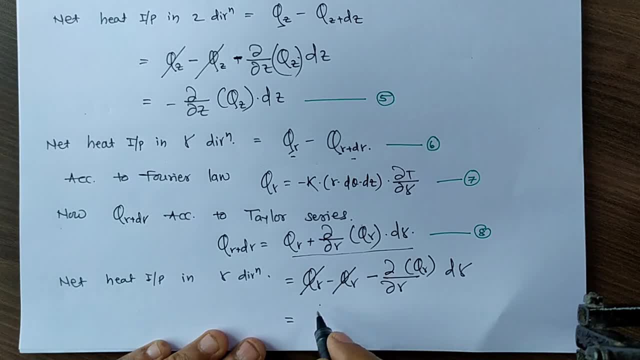 And what is remaining now? The remaining is minus daba by daba R QR DR. So this is what we have got: net heat input or net heat input in R direction. Let me consider: this is equation number 9.. 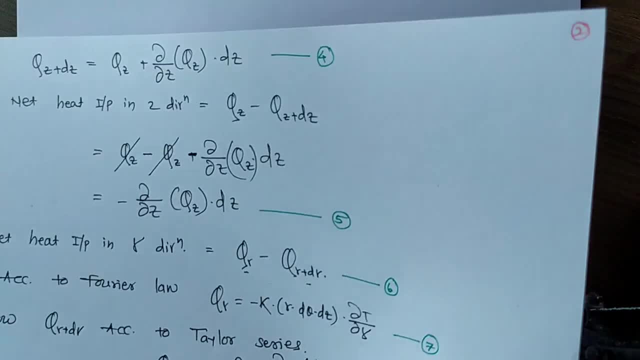 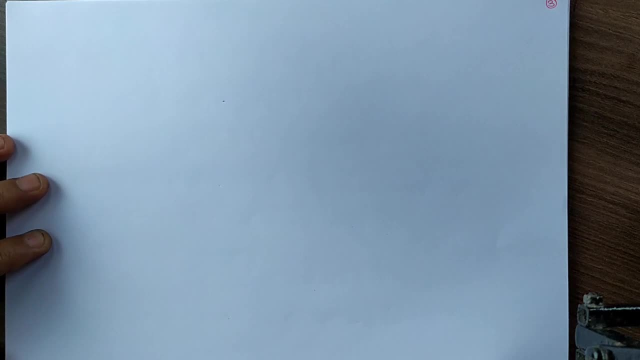 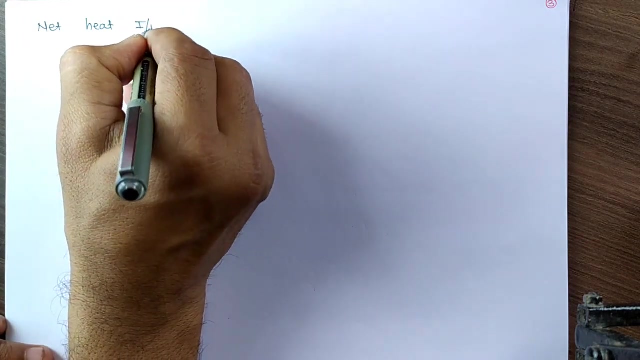 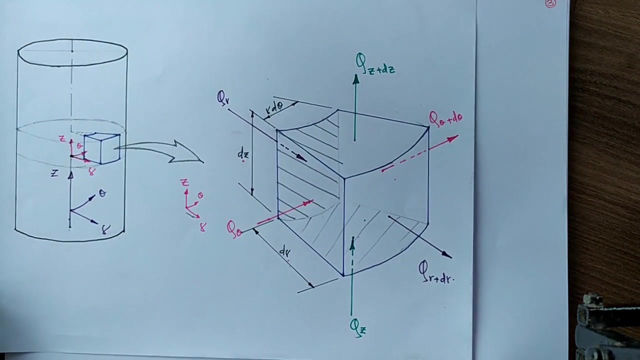 Equation number 9.. Similarly, we have to go for now, the direction: theta. Net heat input in direction: theta. So net heat Input in theta direction, Theta direction. So what is theta direction? We have to refer this particular figure. 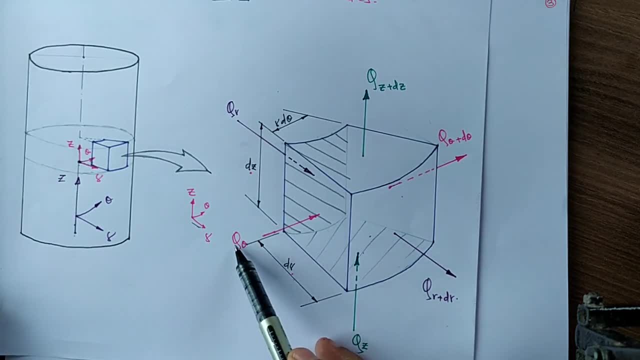 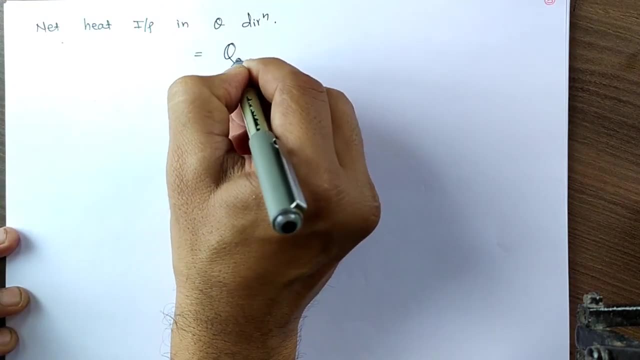 Theta direction is this one, Theta direction is this one. So in this direction, heat entry is Q theta, Heat exit is Q theta plus D theta. So we will get an equation as like this: Q theta minus Q theta plus D theta. 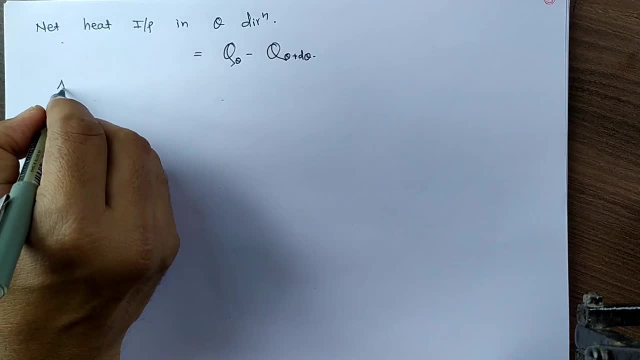 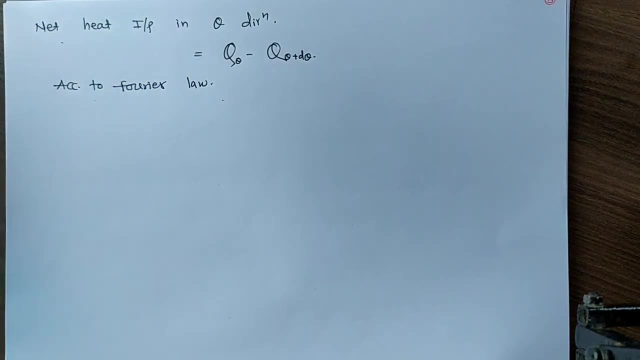 Okay, So we have to write Q theta according to Fourier law. So according to Fourier law, Fourier. Before this I will put an equation number for this one. This is equation number 10.. Previously we have came up to 9.. 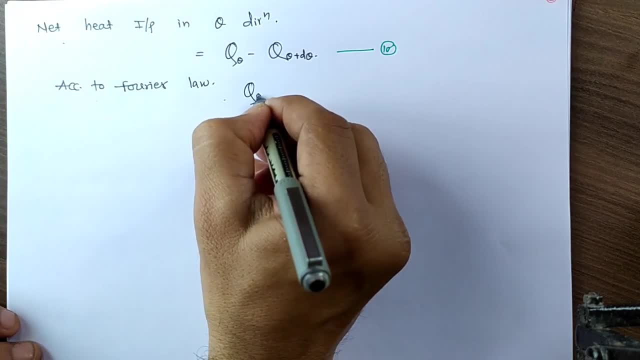 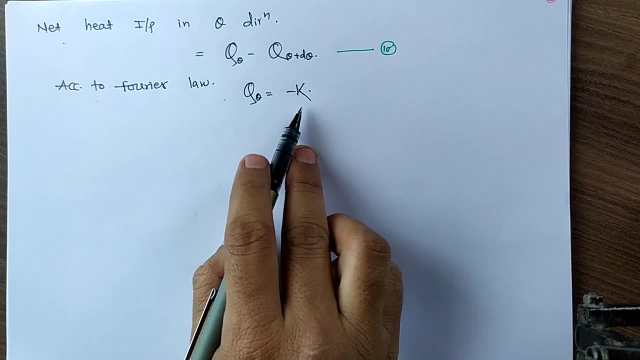 So this is equation number 10.. According to Fourier law, what is Q theta? Q theta is minus KA dt by D theta that we generally write. So area Area in theta direction, Perpendicular area in theta direction. So we are moving in this direction. 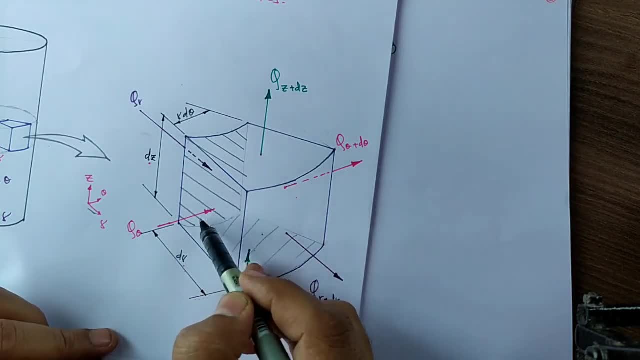 We are moving in this direction. What is the perpendicular area? Perpendicular area? is this plane now, This plane now. What is the dimension of this plane? That is DR And DZ. You can see here: DR and DZ. 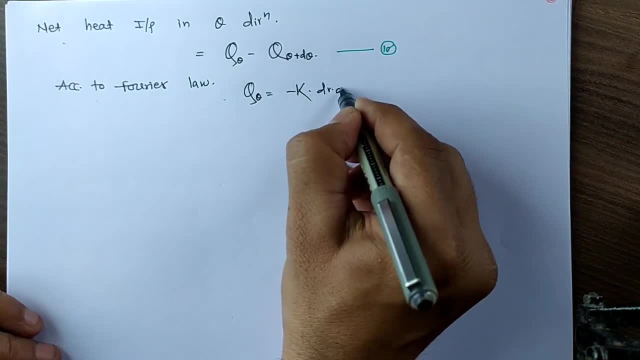 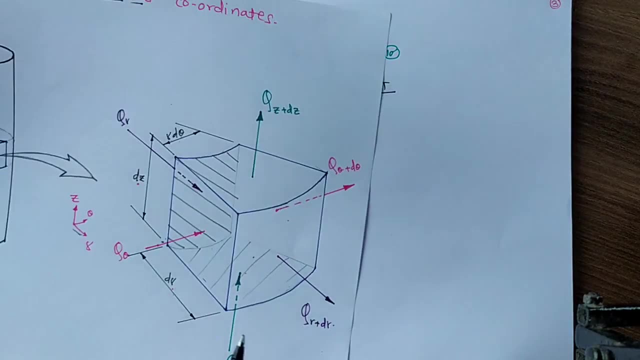 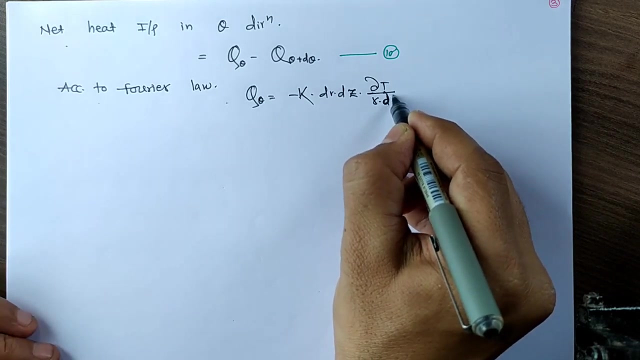 Okay, So I will put here area as DR DZ into change in temperature with respect to theta direction. So in the theta direction actual dimension is RD theta, So I have to put here RD theta. So whatever dimension is there that we have to put here RD theta. 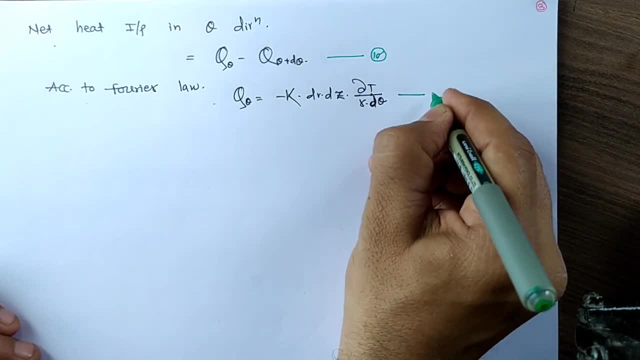 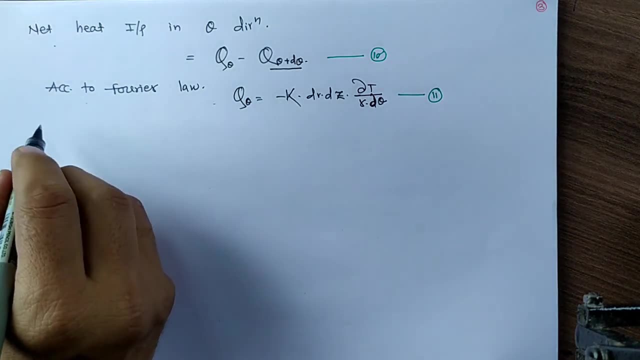 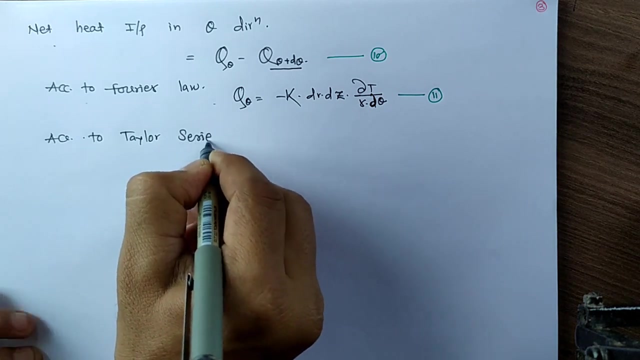 Okay, So that is the Fourier law applied in theta direction. That is the equation number. That is the equation number. Now I have to expand this according to Taylor series. Okay, So according to Taylor series, Taylor series, Q theta plus D theta will become Q theta plus. 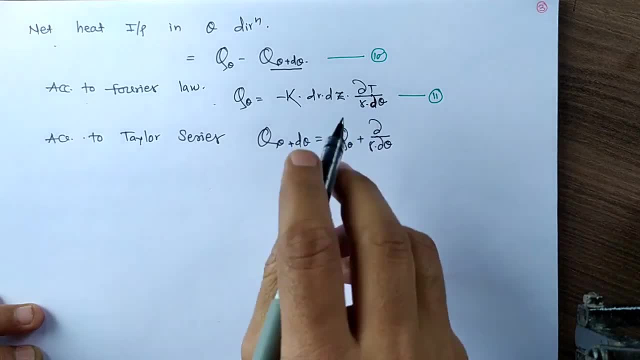 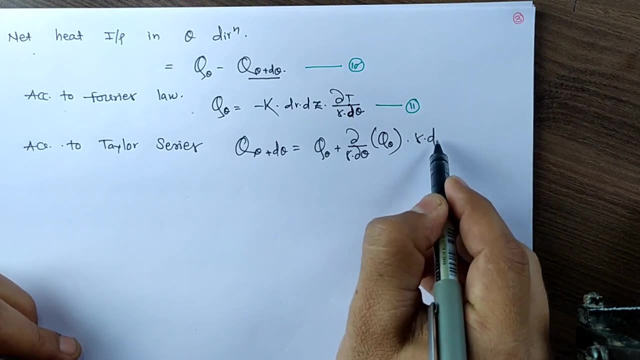 daba of RD daba theta, RD daba theta. Why? Because the dimension is RD daba theta, So I have to put here RD daba theta. Q theta Here becomes RD daba theta, RD theta, Okay. 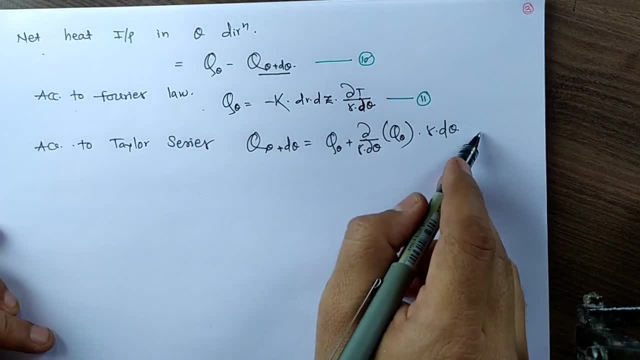 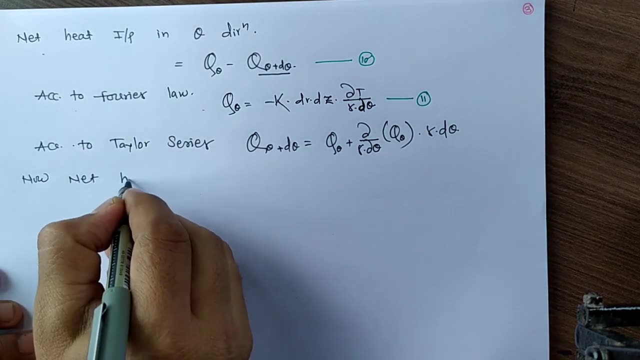 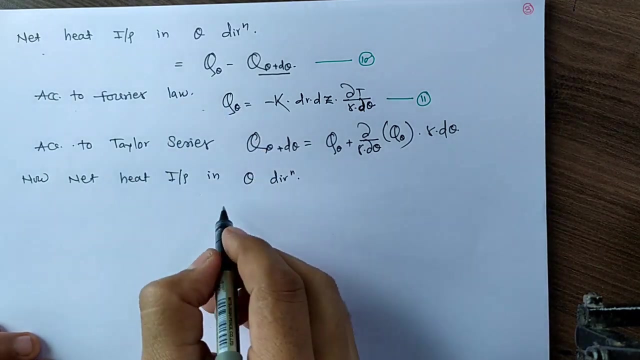 That is the Taylor series. That is the Taylor series. We have neglecting term. I have not written. Okay Now, net heat input in theta direction. Net heat input in theta direction, Theta direction. What we will get, We will get Q theta minus Q theta plus theta. 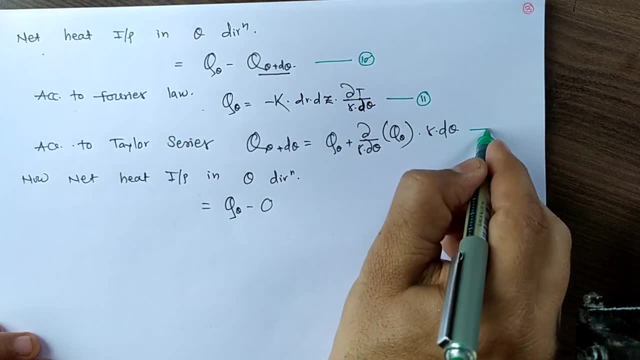 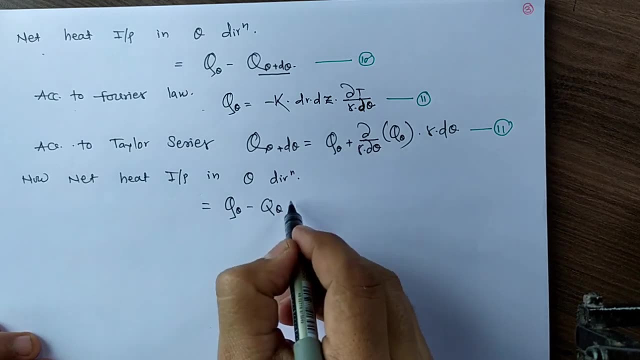 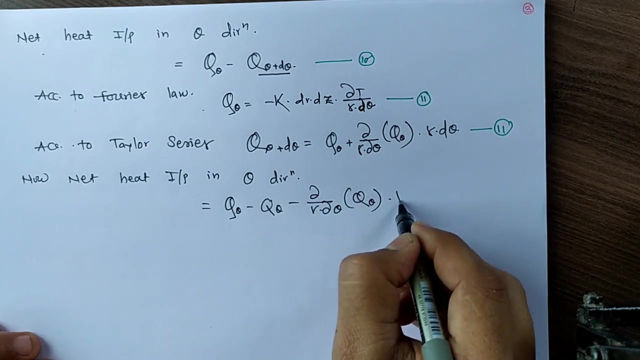 So what is Q theta, D theta? That is the equation number 11.. That is the equation number 11 according to Taylor series. we have written: So minus Q theta, minus Here, once again, minus daba upon RD daba theta. Q theta, RD theta. 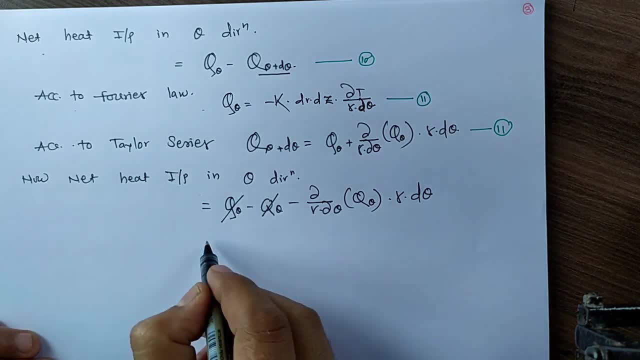 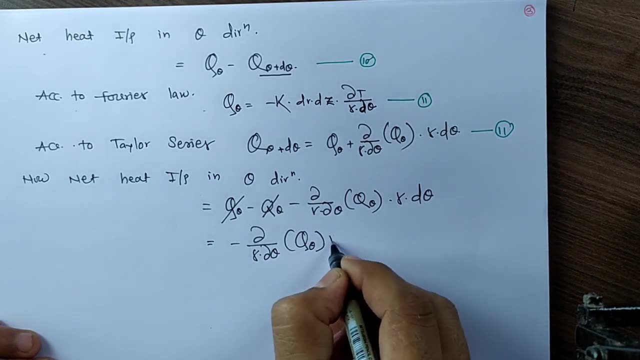 So simplifying this, Q theta and Q? theta will get cancelled. So what is remaining? Minus daba upon RD daba theta. Q theta, RD theta. That is what equation we have got: Net heat input in theta. So what we have done? 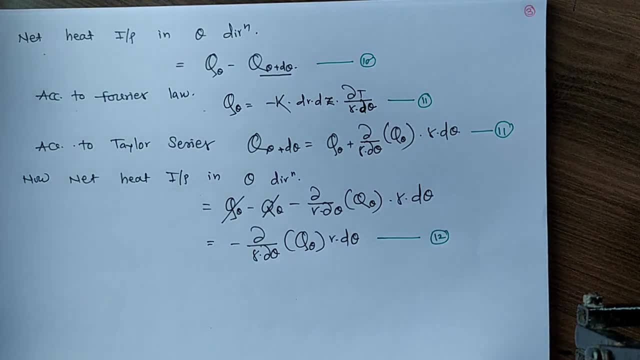 We have determined heat input in all three directions. First of all we have determined for Z direction, Then we have determined for R direction And then we have determined for theta direction. So let me show you In the Z direction what we have got. 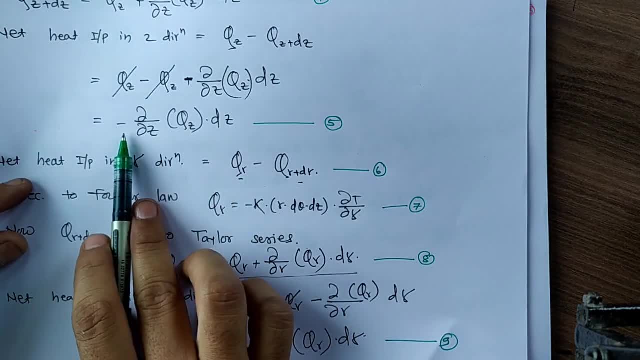 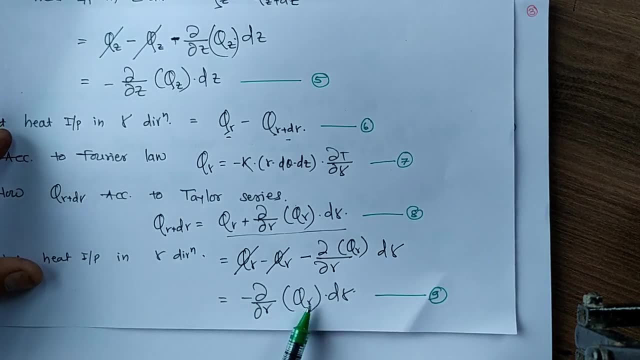 We have got this as equation: In Z direction: net heat input. in Z direction, minus daba upon daba Z QZ, DZ. Okay, In R direction, we have got minus daba upon daba R QR DR And in theta direction, we have got this one: 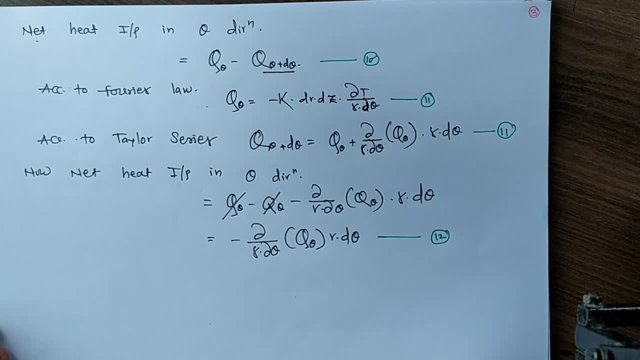 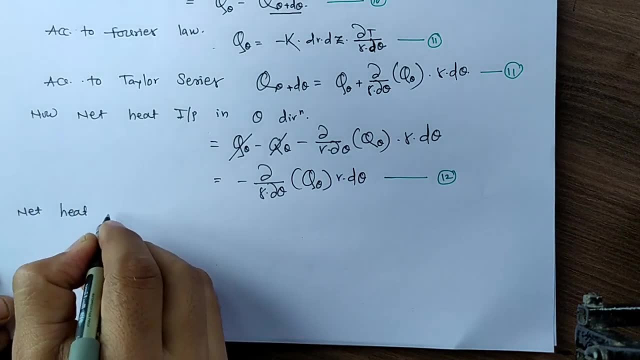 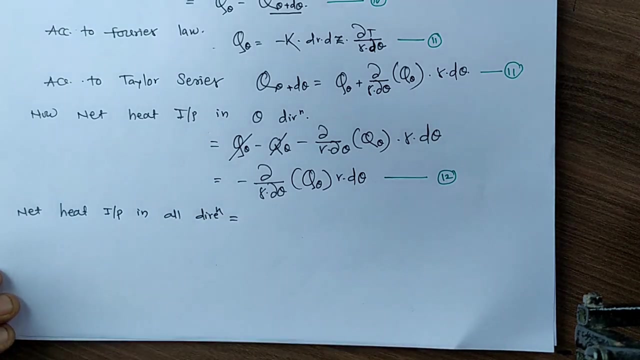 Okay, So all these things we have to combine together, That is net heat input in all direction, What is in all direction, That is the summation of all these three. Summation of all these three, whatever equation just now, we have shown it. 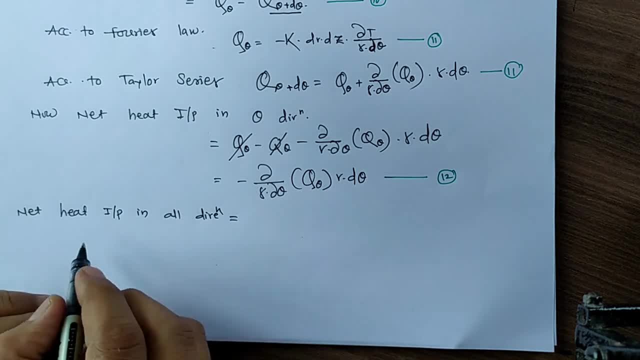 So first of all I will write net heat input in Z direction. So what is in Z direction? Z direction, it says Z direction. it says Minus daba R of daba Z, minus daba of daba Z. QZ, DZ. 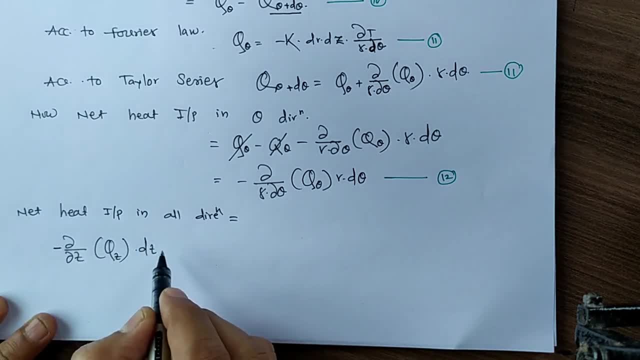 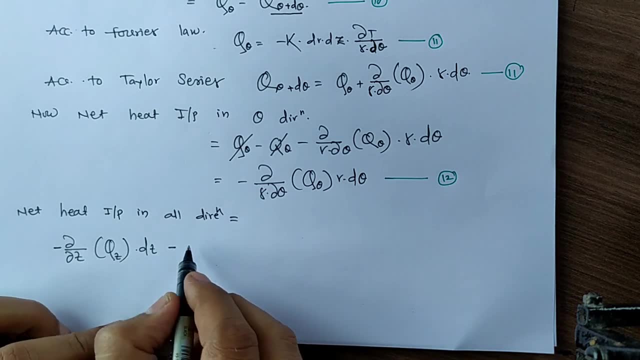 That is the first direction Plus, But this plus in the R direction. So in the R direction it is minus. So plus, minus, minus, It will become daba upon daba R QR DR, That is, in the R direction. 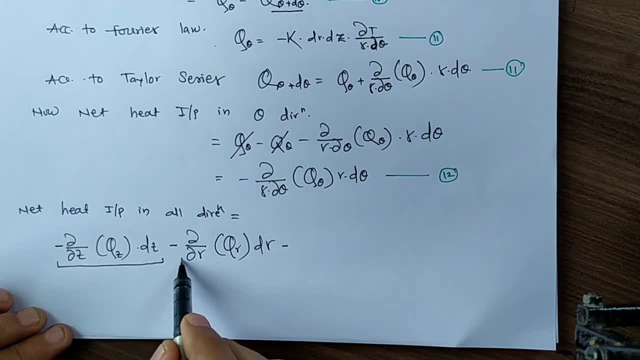 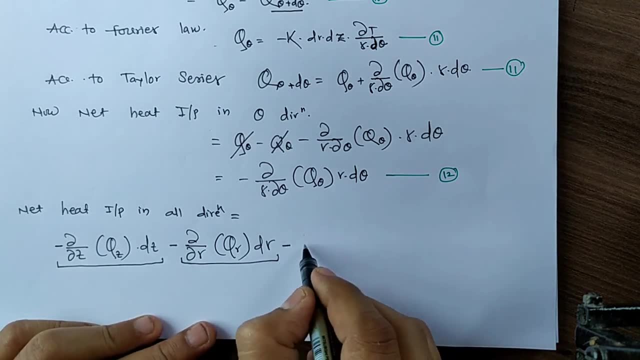 So this is in the Z direction: Plus, minus, it will become minus. That is in the R direction. Now I am going to write in the theta direction. So in theta direction once again: plus minus, it will become minus. 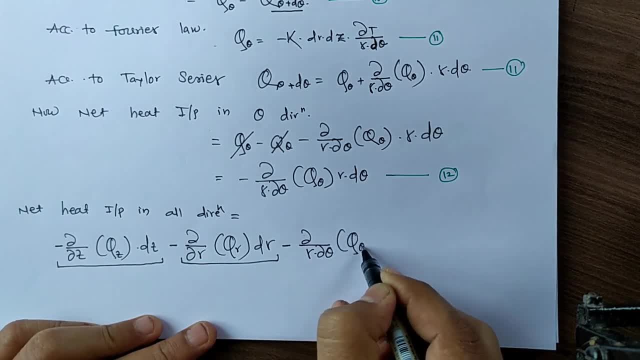 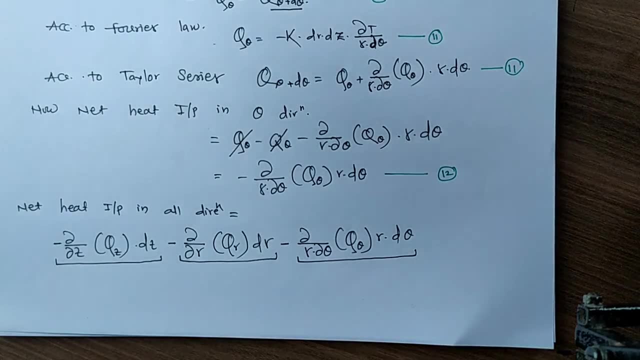 Daba upon R daba, theta, Q theta, R D theta. That is in the theta direction, That is in the theta direction. That is what we have got. That is what we have got, the what heat input in all this direction. So let me consider this as equation number 13.. 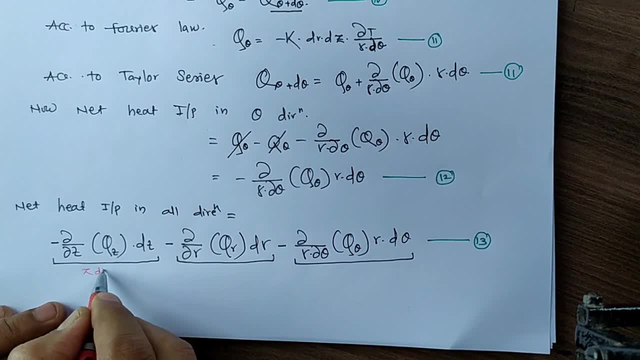 And here, this is in Z direction, This is in Z direction, This is in R direction And this is in theta direction, All three directions. we have written it, Okay. So we have got the first equation for the part number 1.. 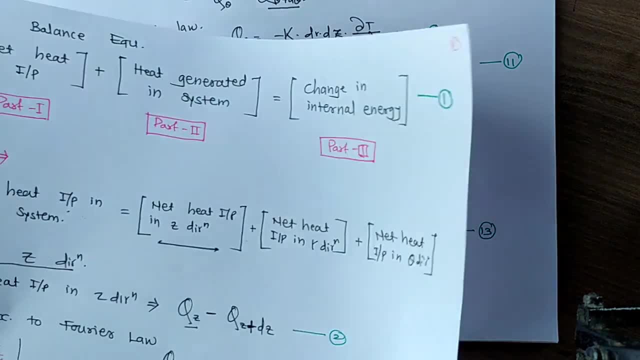 So this was the part number 1.. This was the part number 1.. Coming to the initial equation now, This was the part number 1.. Net heat input in all direction And net heat input in all direction. we have got equation number 13.. 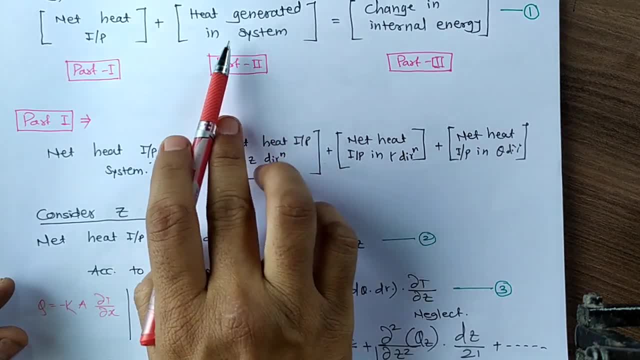 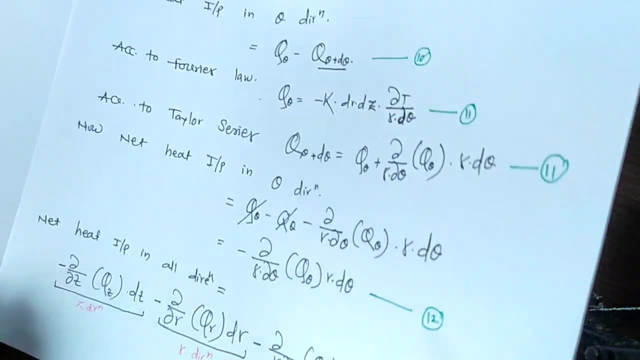 Now we have to go for part number 2.. What is part number 2? Heat generated in the system. Heat generated in the system. So what will be heat generated in the system? Let me take a new page, So it will become part number 2 now. 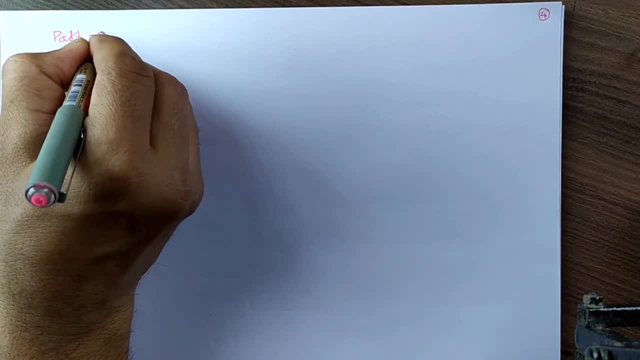 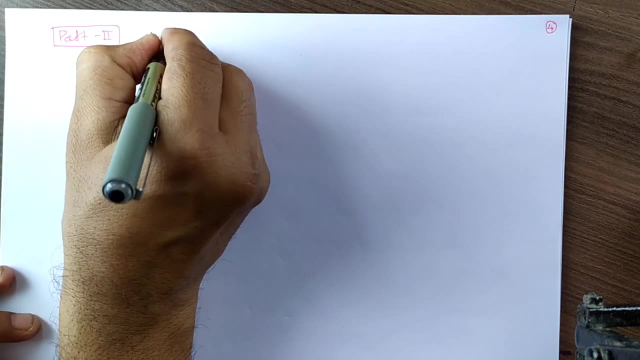 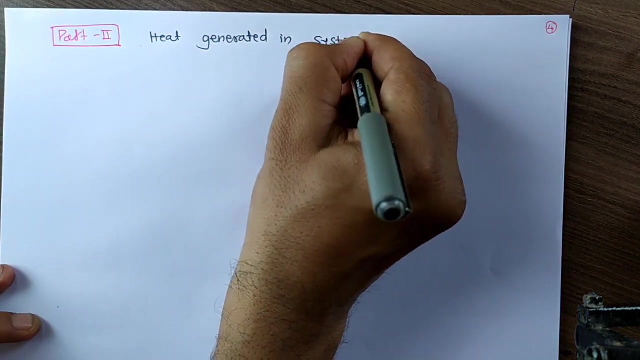 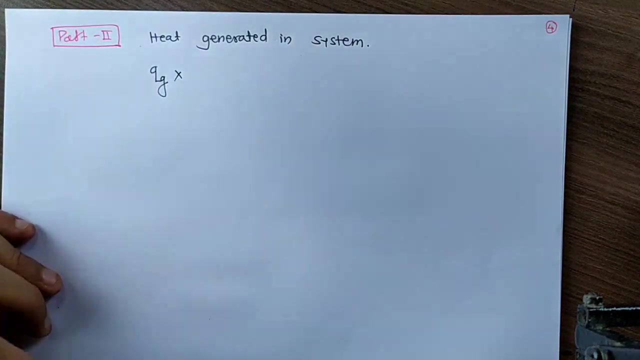 The part number 2.. Part number 2.. That is what. That is what Heat generated in the system, Heat generated in system, Heat generated in the system. So what is heat generated? Generally, QG. Generally, QG is the heat generated per unit volume. 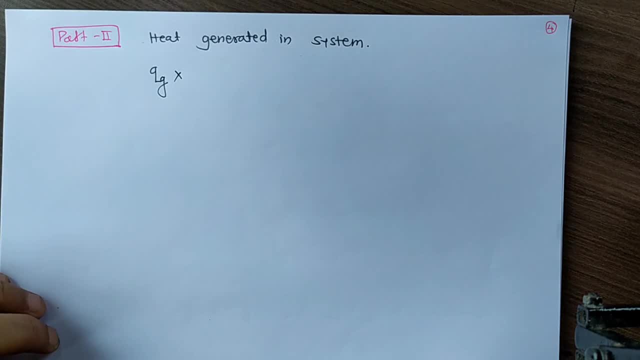 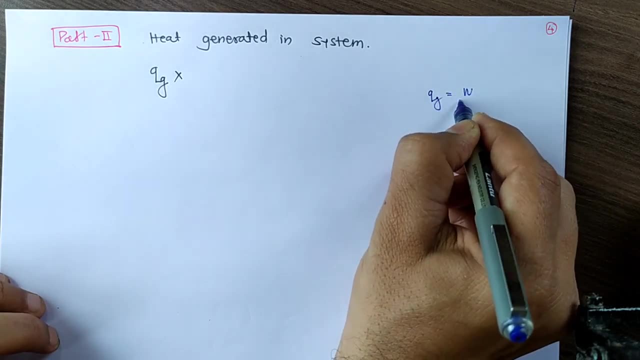 QG is what Heat generated per unit volume? It is unit Heat generated per unit volume. Its unit will be what? So if I write on this side, QG generally is in watt per meter cube, So that is heat generated per unit volume. 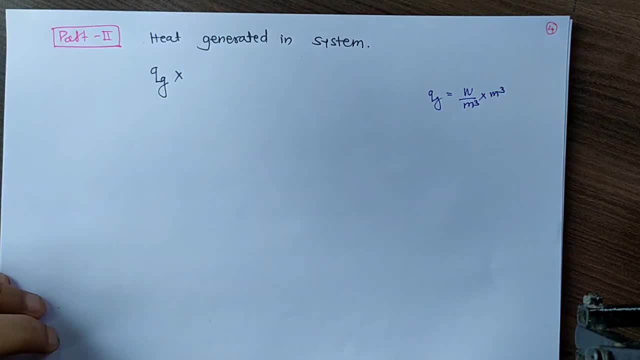 So if I multiply by meter cube then it will become a watt. Meter cube is what Volume? So what we have to do, We have to multiply by volume. We have to multiply by volume, So heat generated in the system. 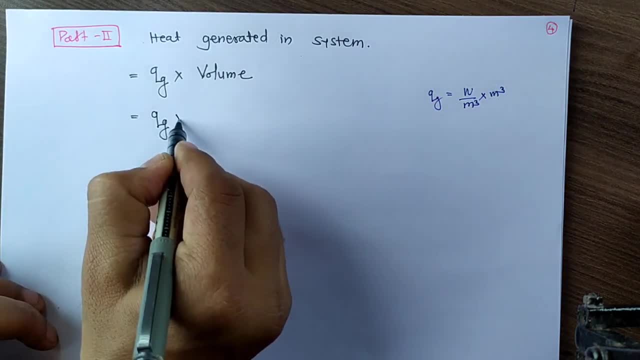 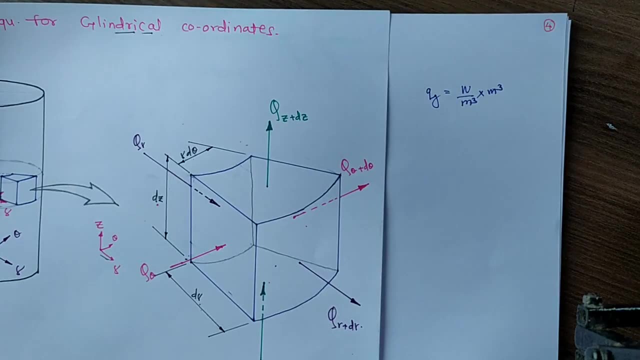 So we have to multiply by QG into volume. Now, what is the volume of element? What is the volume of element which we have considered? So if I consider this particular element, now Volume of this particular element is what You can consider, that all three dimensions. 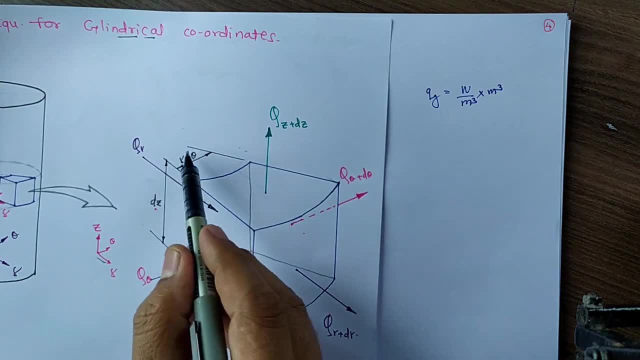 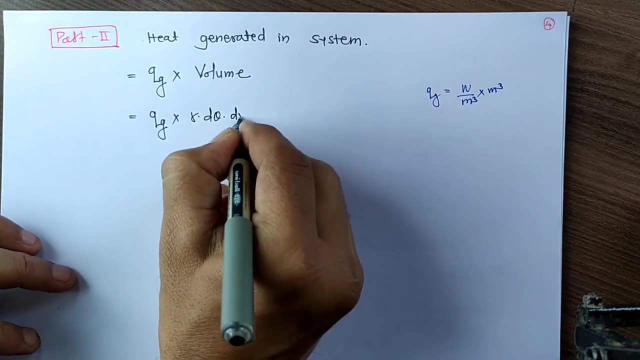 First is RD, theta, DZ and DR. So if I multiply these three, then we will get volume. So volume will become now here: R, D, theta, DR, DZ. That is the volume, And we have got part number 2.. 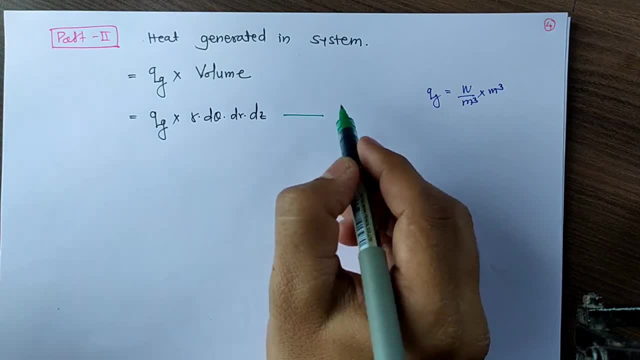 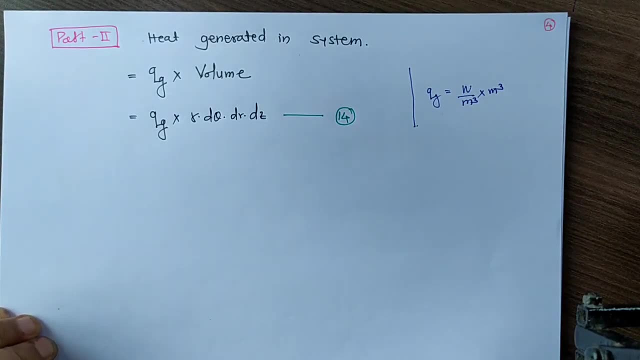 So part number 2.. Equation is quite easy. Part number 2 equation is quite easy And that is the equation number 14.. That is what equation number 14 we have got. Now we have to go for part number 3.. 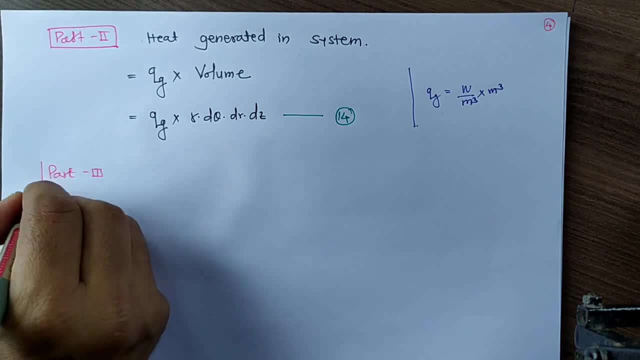 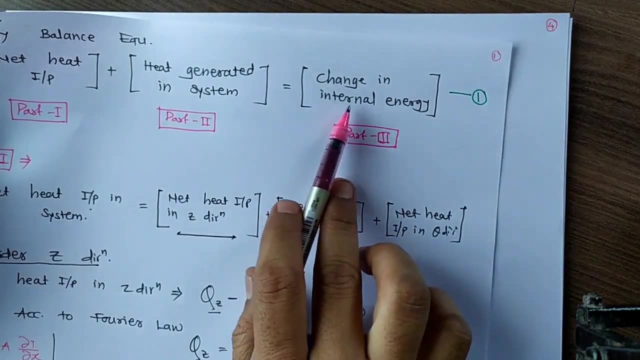 What is this part number 3?? The part number 3 is, if you go for initial equation once again In a part number 3, what we have seen is change in internal energy. You can see here Part number 3,, change in internal energy. 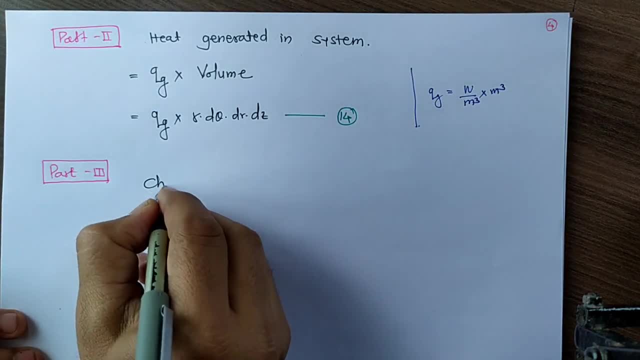 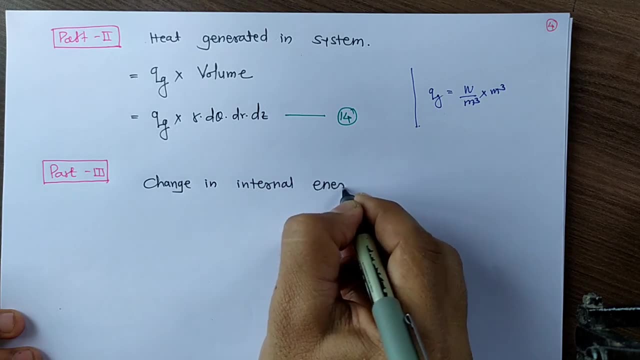 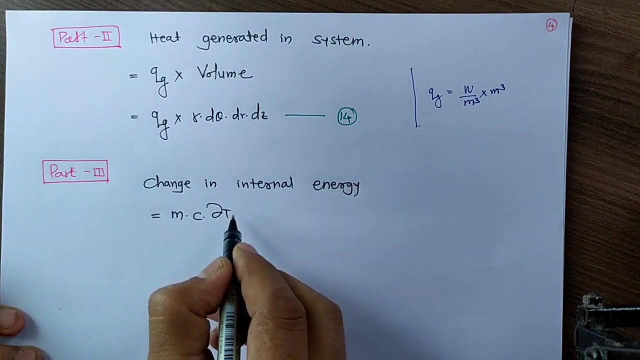 Okay, So what is change in internal energy? Let me write change In internal energy, of system. Change in internal energy we can write by simple equation: MCP, delta T, So MC, Change in temperature with respect to time. That is the equation we are going to use it. 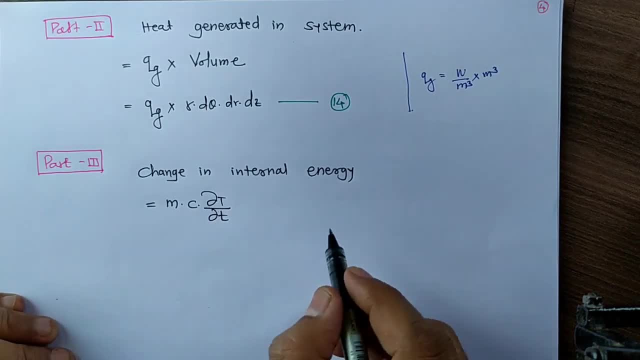 MC, diabetes by diabetes. In this equation, this mass, this particular mass, can be written as what? Let me write this mass can be written as Density into volume. that you must know, because mass is measured in kg. What is density unit? 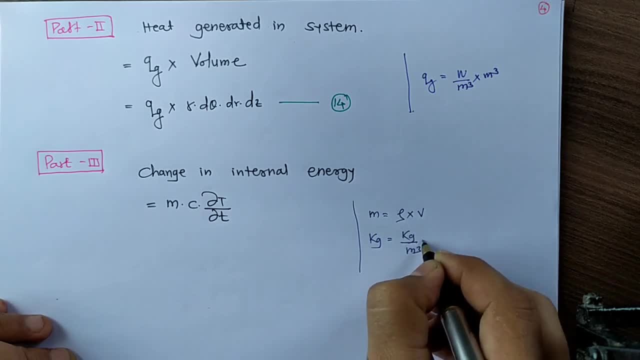 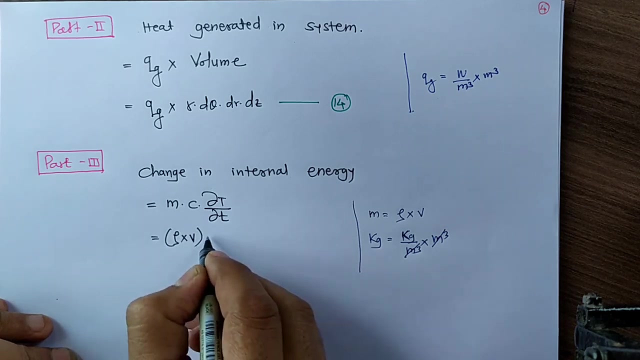 Density unit is kg per meter cube and volume unit is meter cube. So meter cube, meter cube get cancelled. Remaining is kg. So I can write: mass is equal to density into volume, right. So I can write: mass is nothing but rho into V, into C, dou T by dou T. 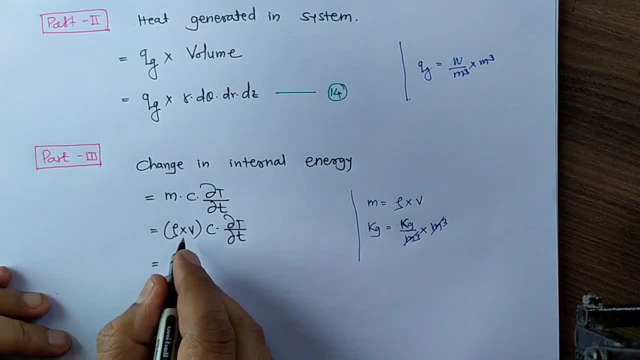 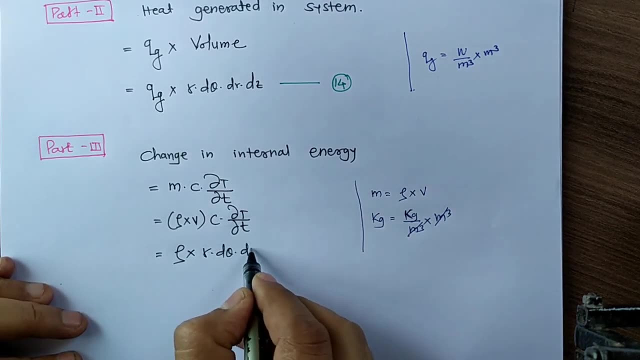 Okay, So what I have done- Mass is replaced by rho- into V. What is the volume? Volume that we have written R d theta dr dz. So let me write density into R d theta dr dz, that we have written it into C dou T by dou T. 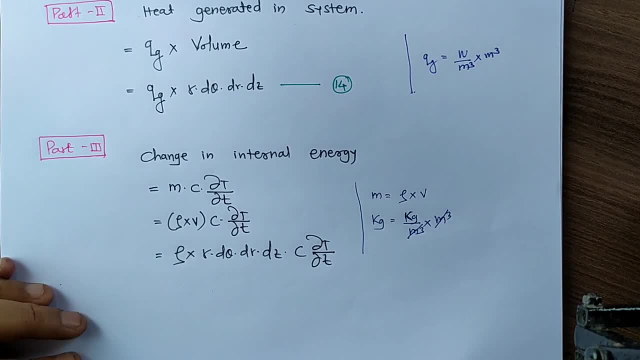 That is what we have got it, Okay, And this is the change in internal energy and that is the equation number 15.. That is the equation number 15.. Now we have got equation for all three. That is part number 1, part number 2, part number 3.. 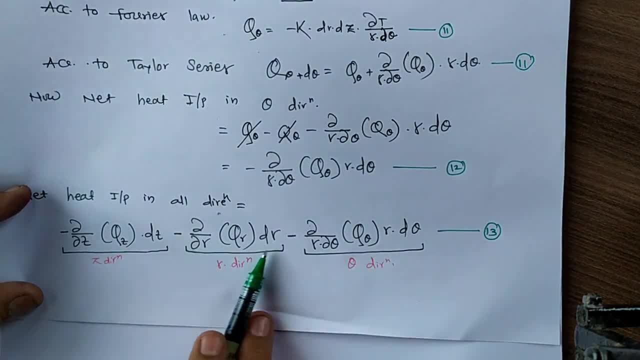 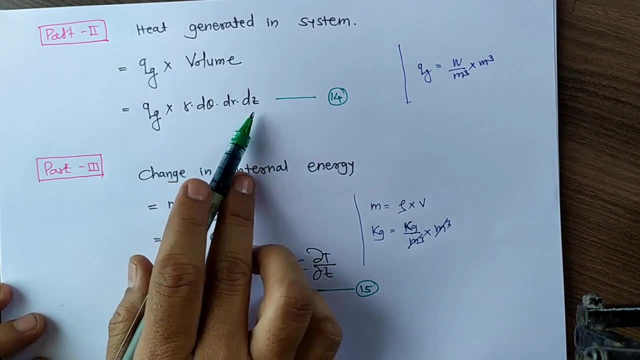 What is part number 1 equation? Part number 1 equation is equation number 13.. That net heat input All direction. Part number 2 equation. Part number 2 equation is heat generated in the system Qg, R, d, theta, dr, dz. 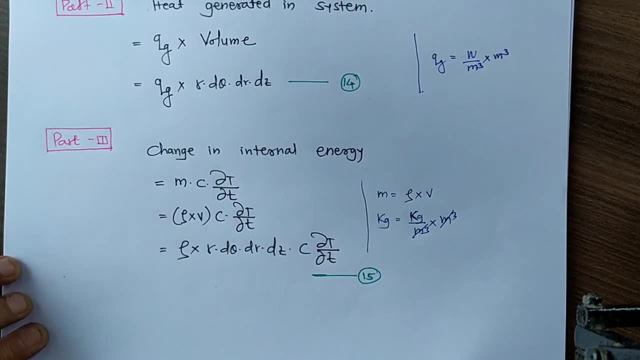 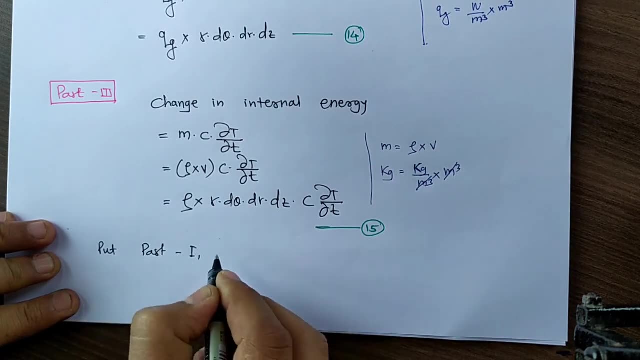 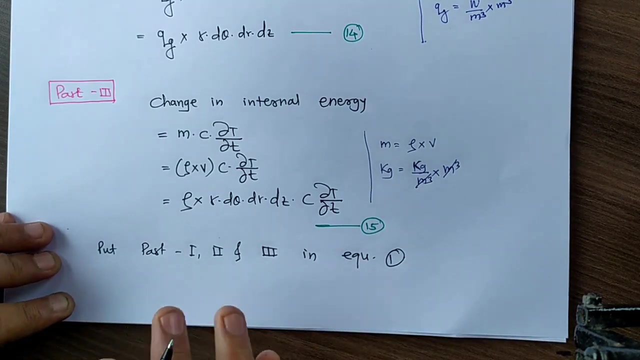 Part number 3 is this one. So put Now what I am going to do is I am going to put part 1, 2 and 3 in equation number 1.. That is the basic equation. So in the basic equation we are going to put all this part. 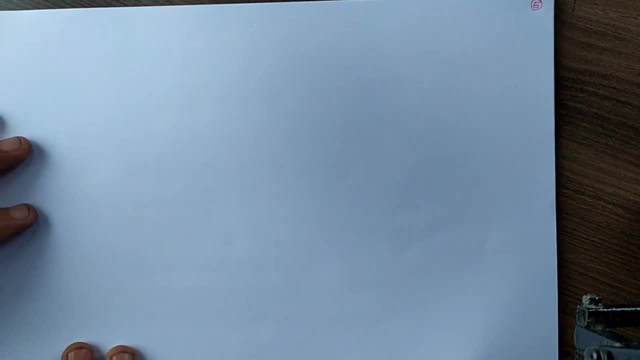 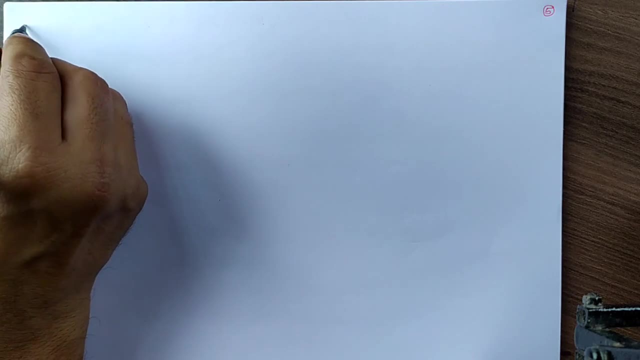 Okay, All this part. So let me write First of all for the net heat input, part number 1.. Part number 1 equation, That is the equation number 13 you can refer. So that says part number 1 equation. I will write as like this: 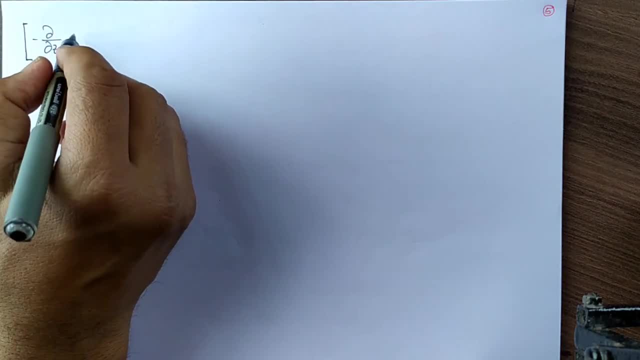 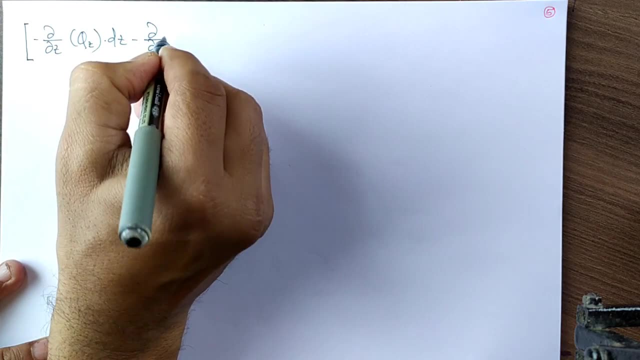 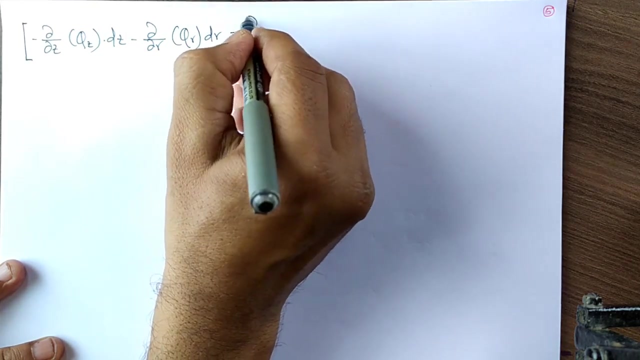 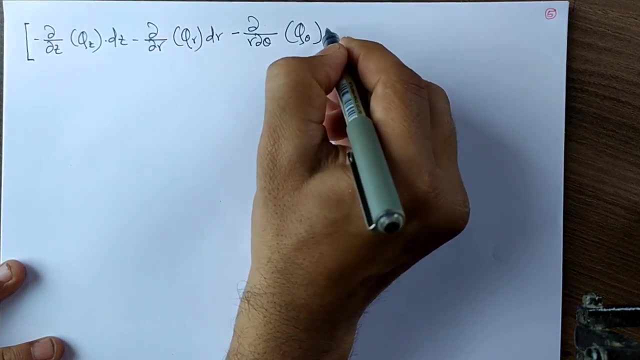 Minus daba by daba z, which we have already proved That. minus daba by daba z, Qz, dz. minus daba by daba R, qr, dr. That is the equation number 13. we are writing: Okay, Minus daba by R daba, theta, q, theta, R, d, theta. 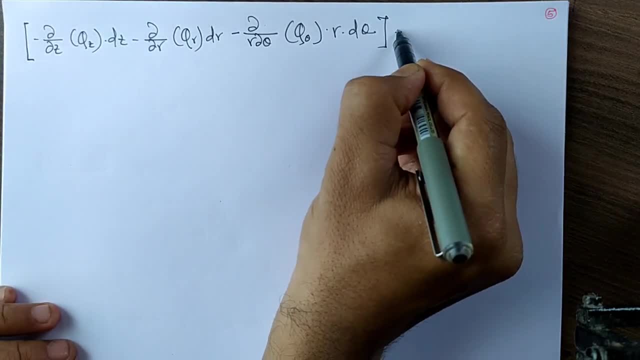 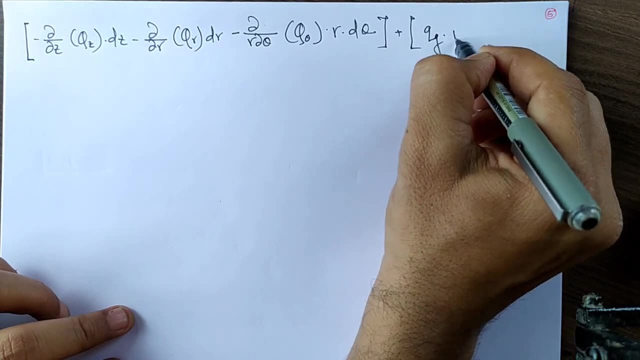 Okay, So that is what we have written, Part number 1.. What is part number 2 plus part number 2?? Part number 2 is equation number 14. And that is Qg into volume, That is R d theta, dr dz. 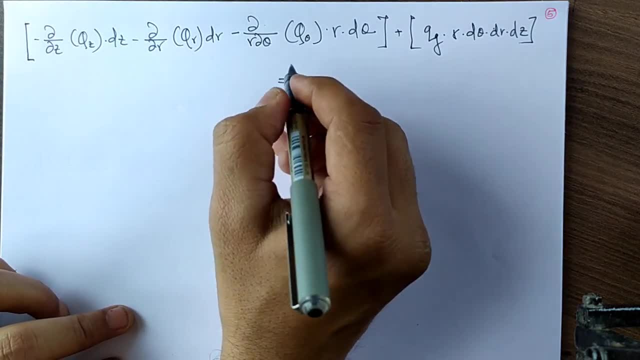 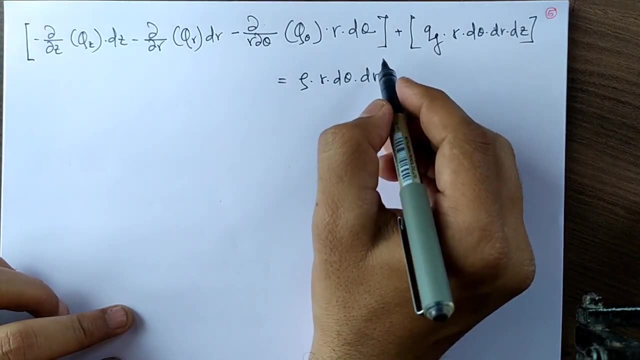 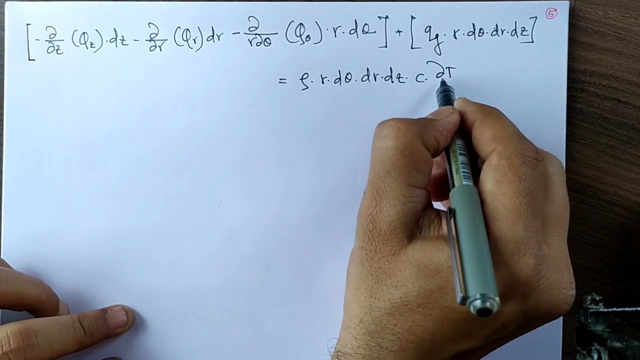 That is what we have written- Is equal to change in internal energy. That is the equation number 15.. That is rho R d theta dr dz into c, into dou t by dou t. So that is the part number 1, part number 2 and part number 3.. 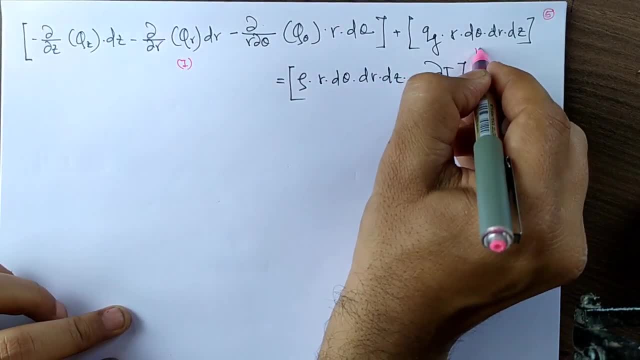 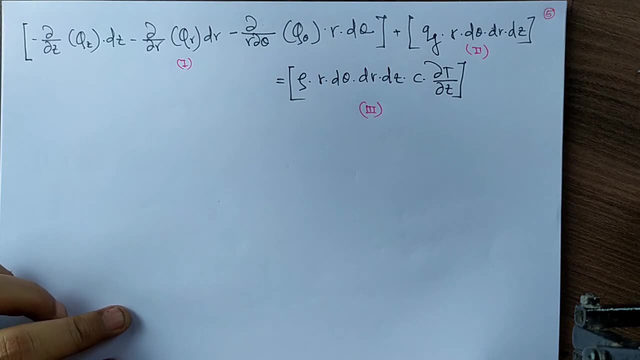 We have taken from different equations. That is the part number 1.. That is the part number 2. And that is the part number 3.. So we have to simplify this. We have to simplify this. Let us go for simplification. 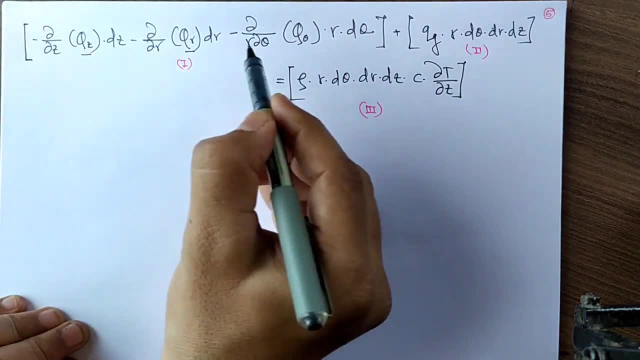 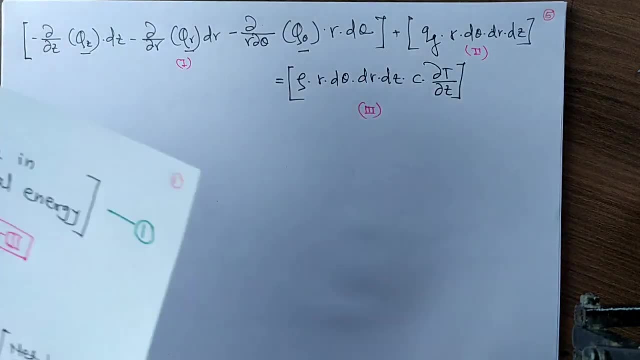 Let us go for simplification. In this particular equation there is a Qz, Qr and Q, theta That already we have derived according to Fourier law, That already we have derived according to Fourier law. So, for example Qz, already we have derived equation number 3.. 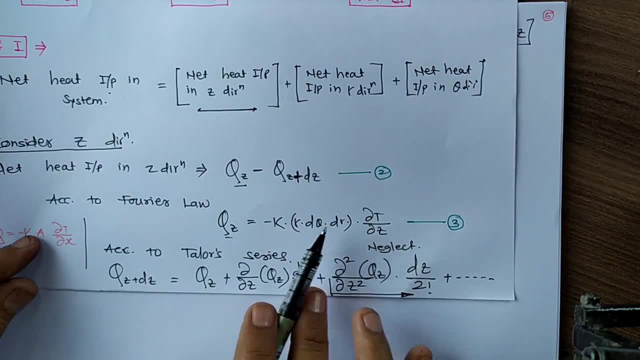 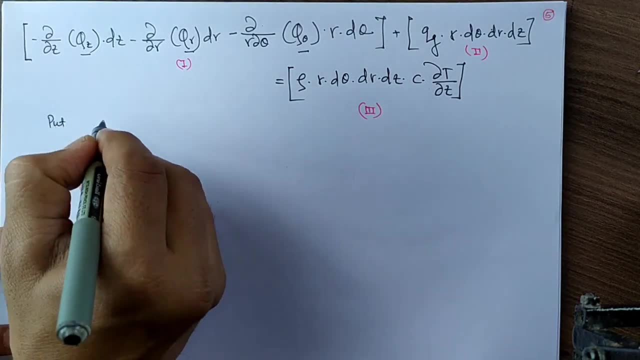 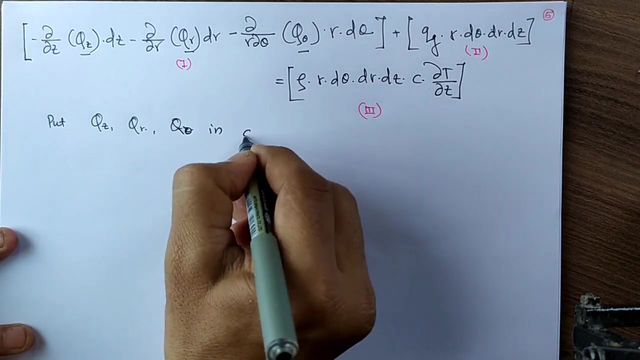 That is Qz minus kr, d theta, dr. Similarly Qr and Q theta. these equations are available above. Okay, So put Qz, Qr, Q theta In above equation. So what we will get if we put this one. 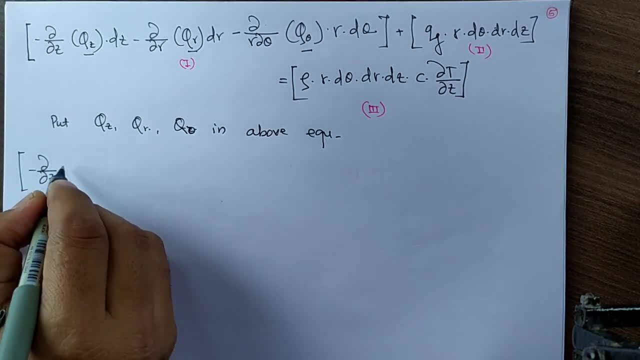 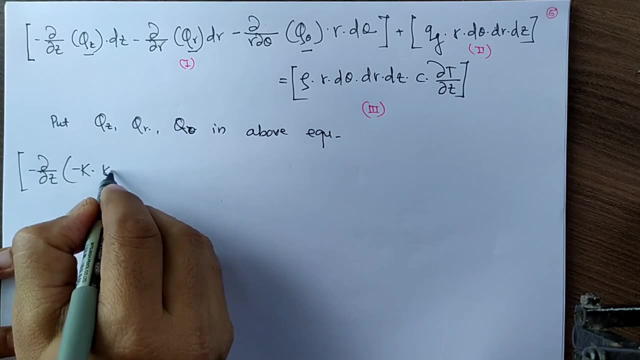 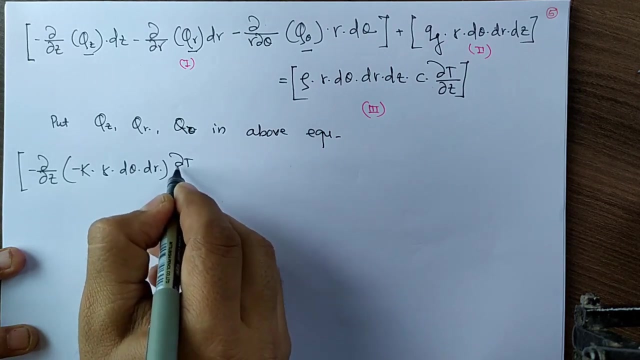 So let me write once again: minus daba upon daba z, Qz Instead of Qz. let me refer the equation of Qz So it will be minus kr d theta dr. Okay, Daba t by daba z. 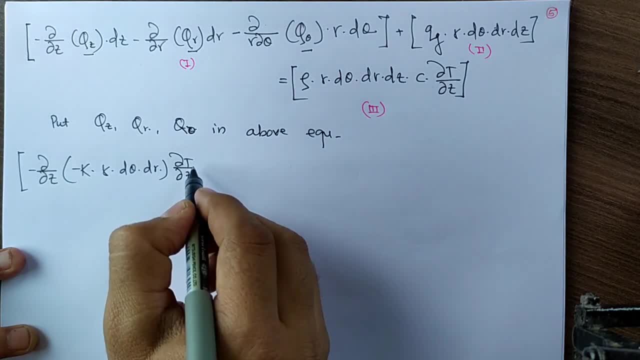 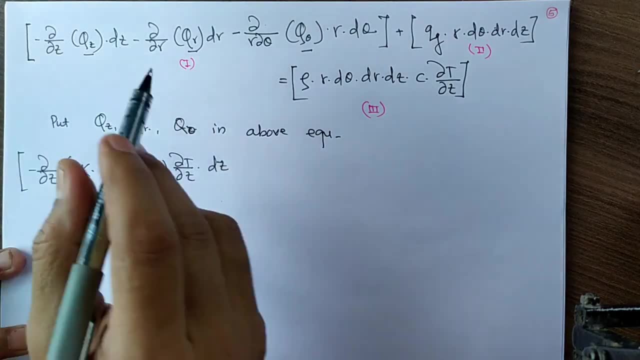 That is the equation. for what Equation for This particular? according to Fourier's law, Qz into dz is also present. Into dz, this dz is present. Minus daba upon daba r Qr I have to put. 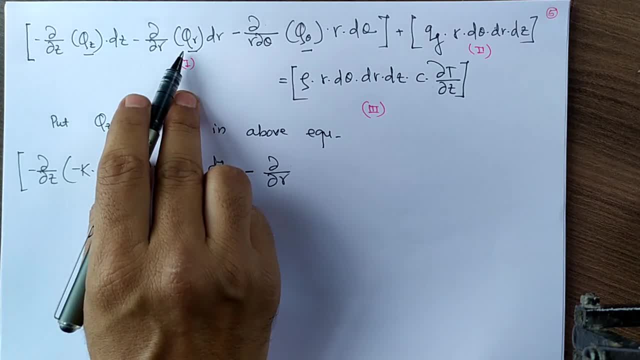 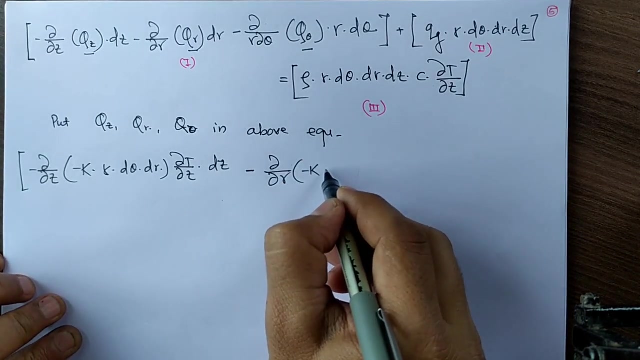 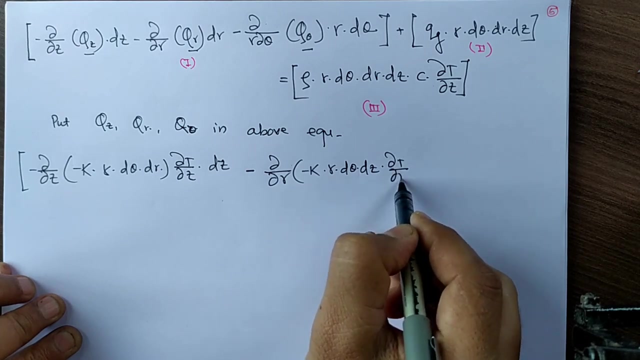 Let me refer the equation for Qr, what we have derived already. So Qr comes to be Just a minute. I will refer the Qr. Qr is according to Fourier's law. It says minus k, Minus k, into r d theta dz, into daba t by daba r into into dr, into dr. 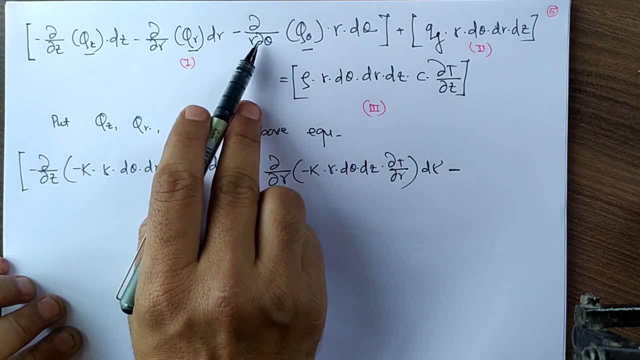 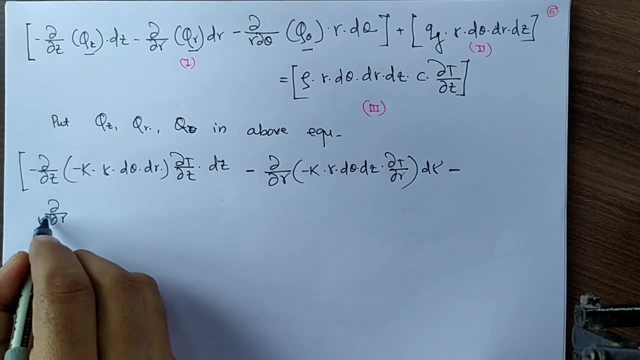 That is what we have done. it Minus, Minus. Now, what we have to put, We have to put Q theta. So what is Q theta? minus daba upon daba r. This is actually daba upon daba theta. 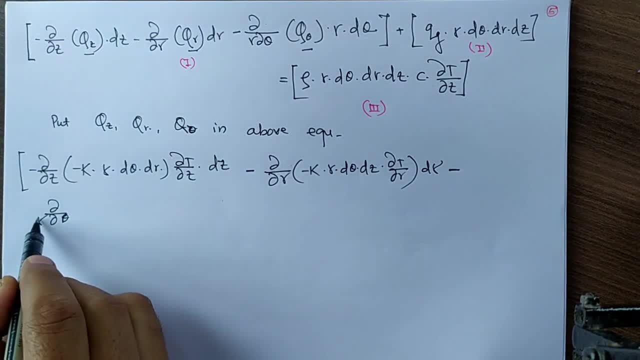 Daba upon daba theta. Here we have taken it. So my here Minus Daba upon r daba theta, Q theta. What is the Q theta, Q theta? you can refer from the equation number, Equation number 11.. 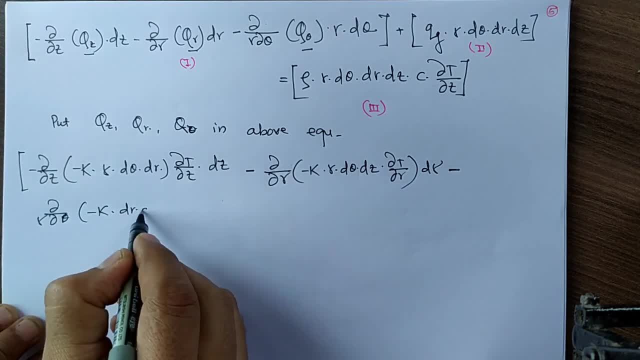 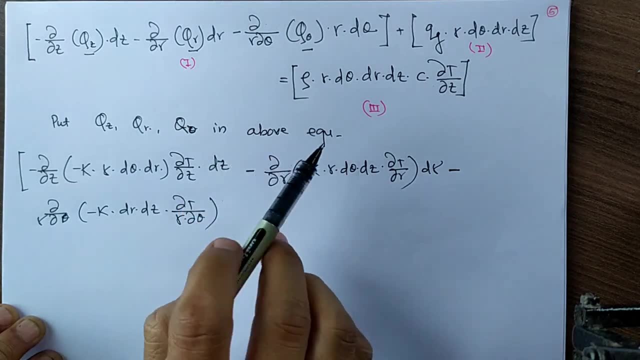 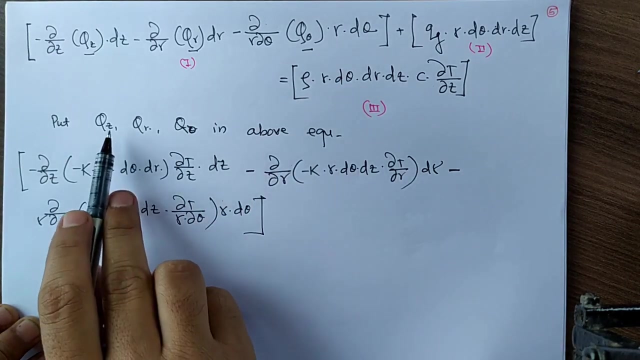 So it says: minus k dr dz. change in temperature: r daba theta. That is what equation we have written for d theta, r d theta. Okay, So we have put all Qz, Qr, Q theta which we have written above, plus. 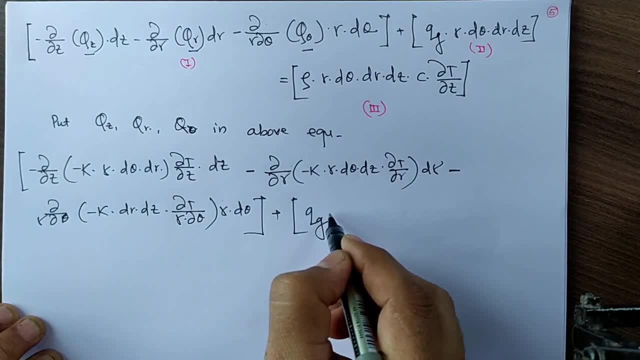 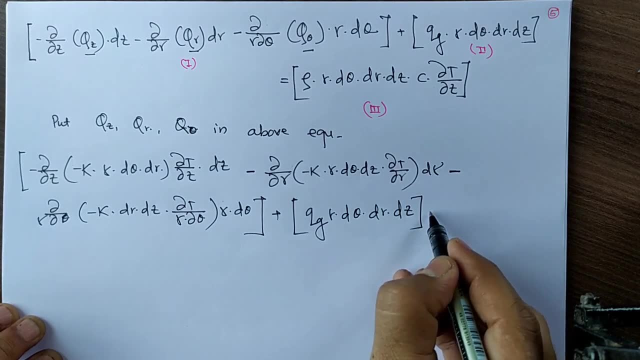 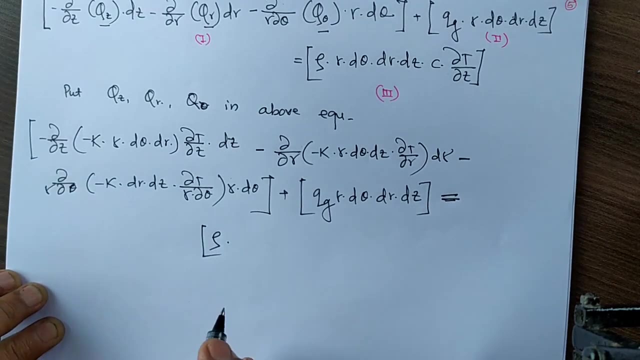 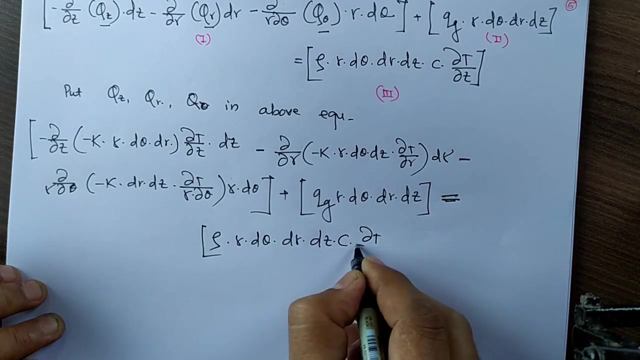 This term will remain as it is, That is, Qg r d theta dr dz. Okay, That is what we have written, And further things also remain same, Equal to Equal to what this term, This term is what Rho r d theta dr dz. c dou t upon dou z. 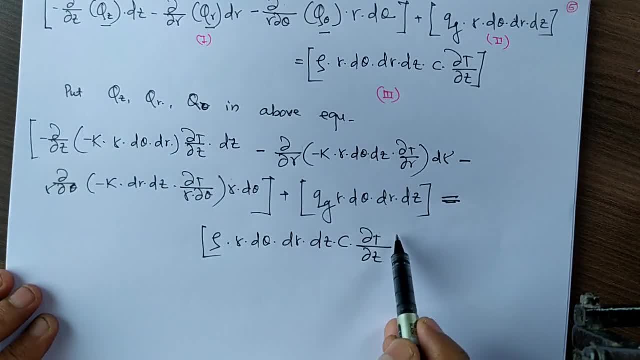 Okay, So this is part number 1. up to this one, This is part number 2 and this is part number 3.. Okay, So once again I can write over here. This is part number 1.. This is part number 2 and this is part number 3.. 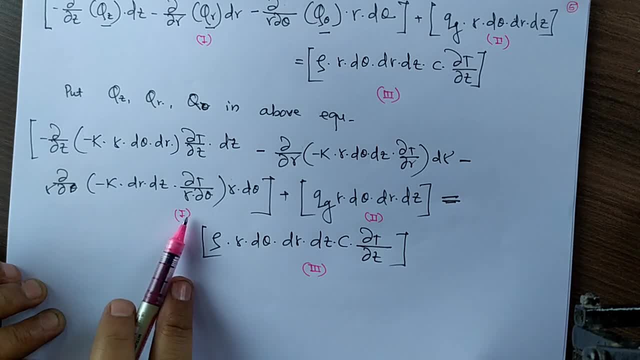 Just what we have done in this particular step is we have written Ah, Qz, Qr, Q, theta. Now, simplifying this: How we can simplify this particular term, How we can simplify this particular term Here. this I will simplify. 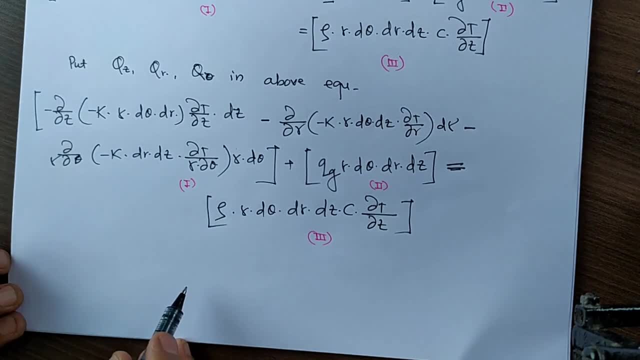 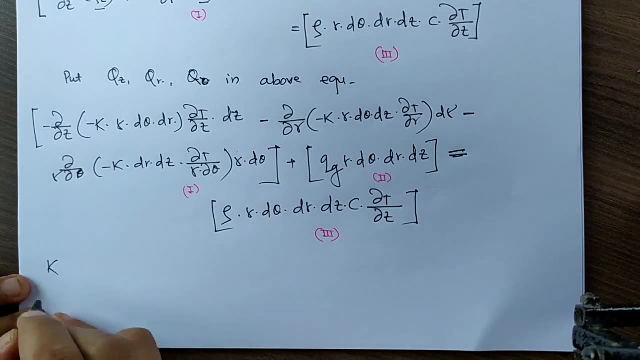 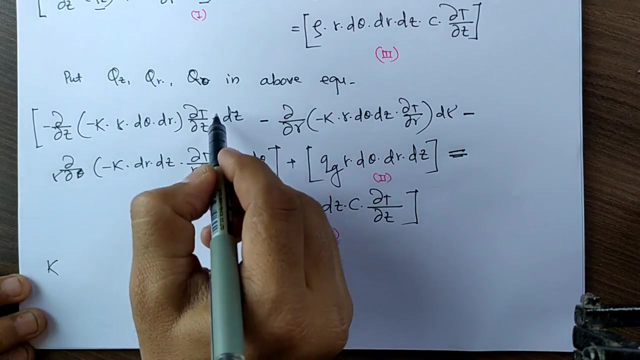 This k, I will take an outside. So let me write over here, So I will write over here that minus, minus it will become a plus k, plus k. This is derivative with respect to z, of all the term which is inside, All the term which is inside. 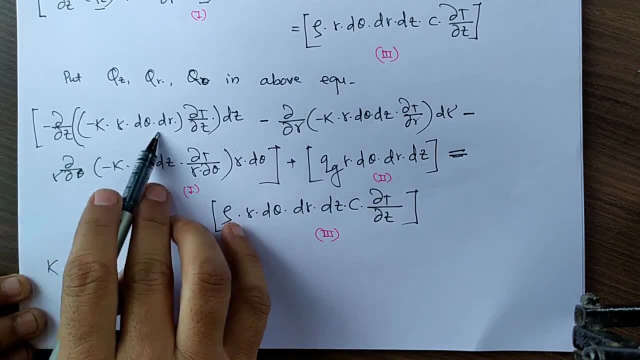 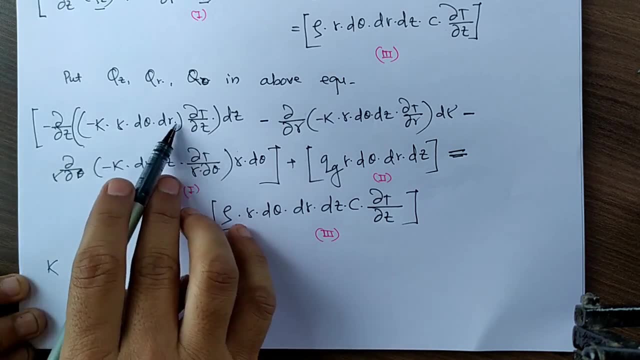 Actually bracket should be like this: Okay, So this is derivative with respect to z, all the term. So z is only variable. All other terms are constant. So in this particular bracket, wherever z is there, that I will keep and others are constant. 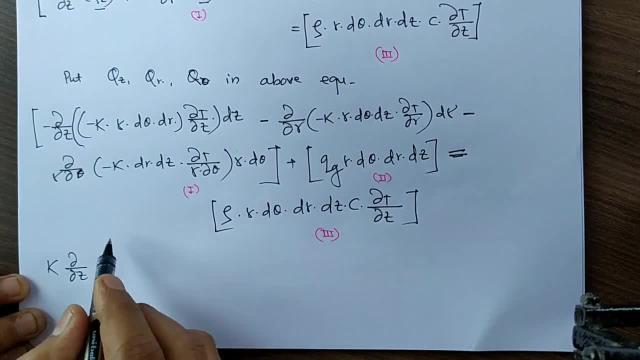 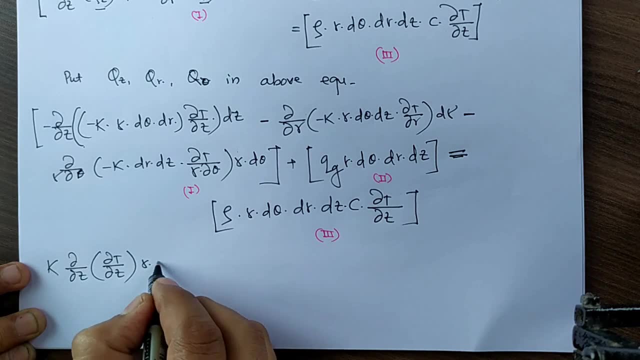 So k I have taken outside Dabba upon dabba z. So what is the term? only dou t by dou z, Dou t by dou z. that is the variable. all other term like r, d, theta, d, r, these are constant. 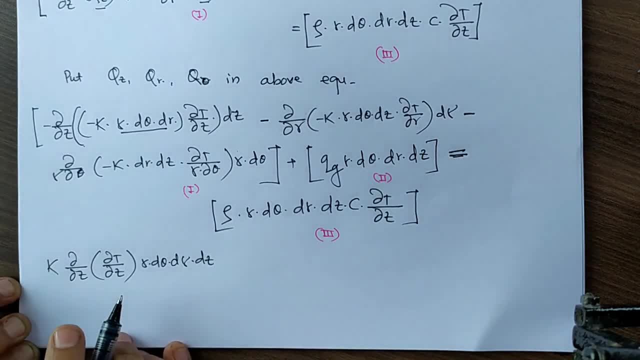 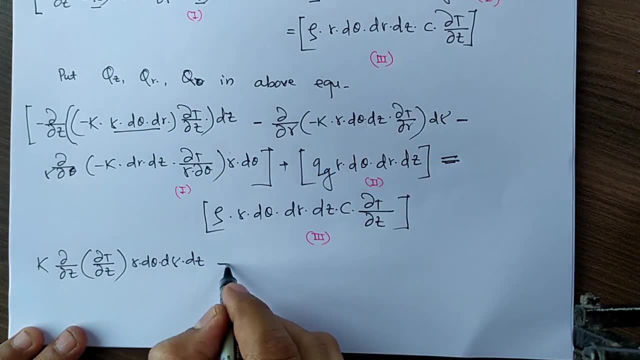 So that I have taken outside into dz is as it is, into dz is as it is. that is what we have done, a simplification for this bracket: minus here, minus, minus. once again it will become a plus. So I will write a plus k in this also. in this also r is variable. 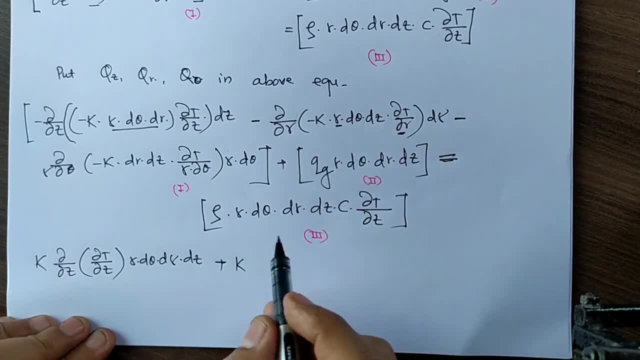 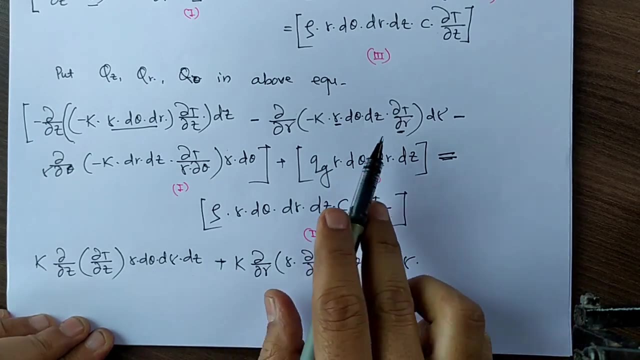 So here is r and here is r. These two terms are variable. all other are constant. So what I will write is dabba upon dabba r. variable is r dou t by dou r. other term, what is other term? d theta dz dr. d theta dz dr is constant. that has gone outside. 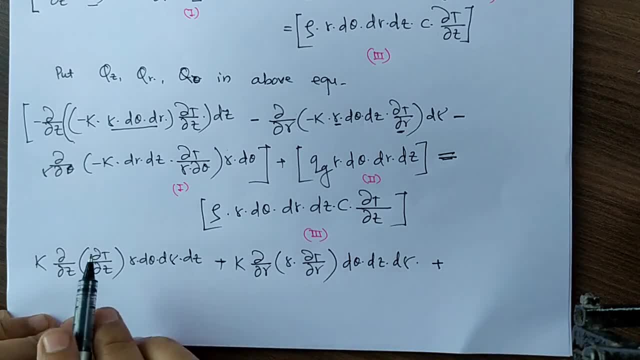 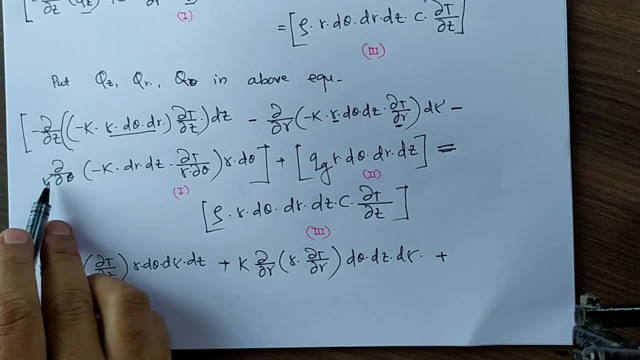 So minus and minus k, once again it will become a plus. it will become a plus into bracket. I will write on a downside over here. I will write a downside over here, In the brackets it is dou by r, dou theta. So what is the variable? 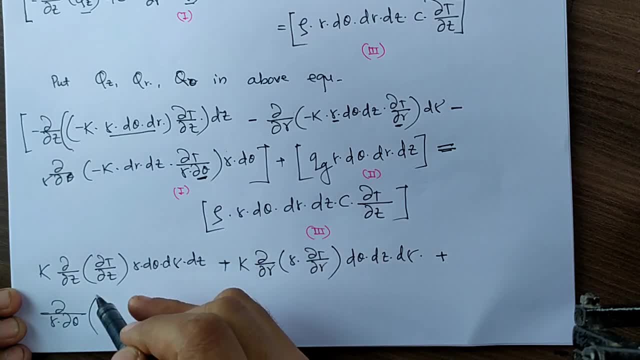 Only theta is variable. So here variable, here is a variable. all other terms are constant. So let me write: the k came outside, this k has gone outside. this dr dz will go outside on this side. So it will become dou t upon other term. I will write as r d theta. dou t upon r d theta. 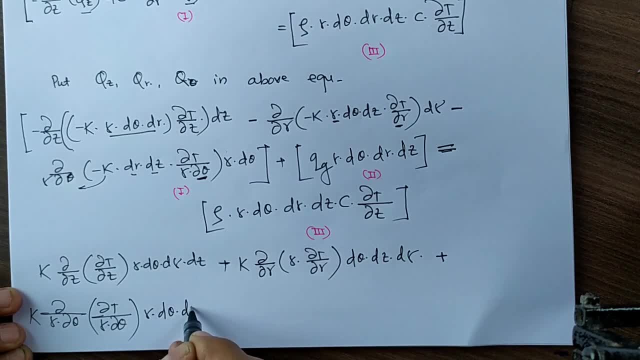 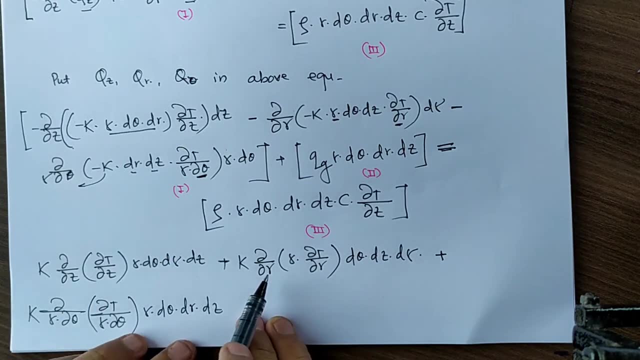 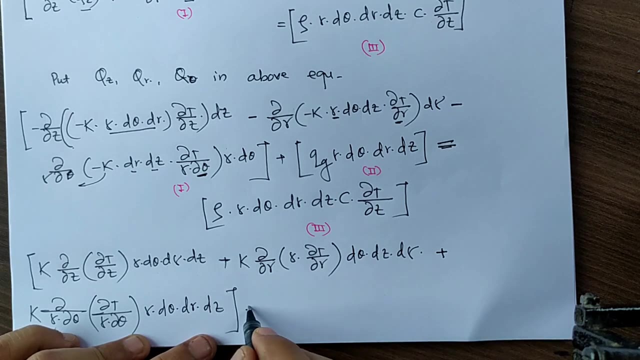 outside bracket: r d theta dr dz. So what we have done is just what we have done. we have taken outside of the bracket. those are constant, those we have taken outside of the bracket. Then this was a part number one. this was a part number one. part number two, I will write as as it is: qg: r d theta dr dz. that's the. 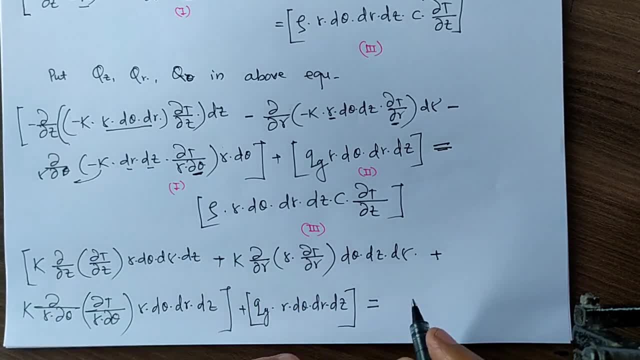 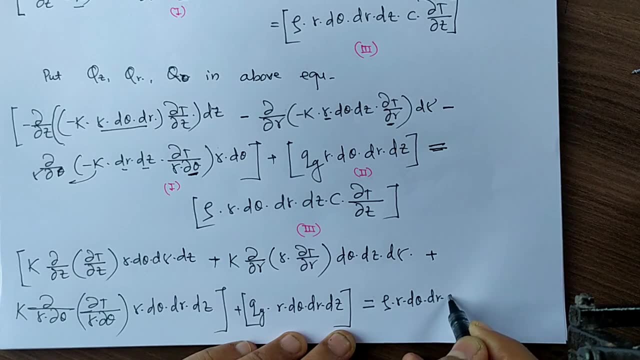 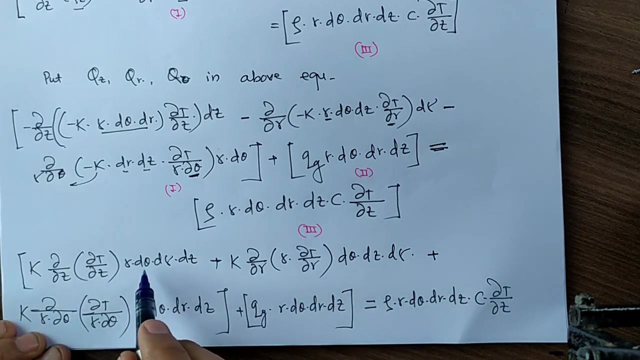 part number two is equal to part number three. part number three says part number three says this: one rho r d theta dr dz, c, dot upon dot. Now what we have to do is we have to, we have to cancel the menu of things from these. all r d theta dr dz is available in the part. 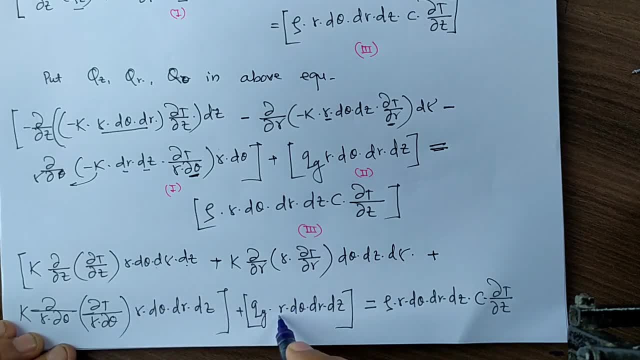 number one, part number two and part number three. Okay so, r d theta dz, r d theta dr dz. we have taken outside of the bracket. We have taken outside of the bracket. We have taken get cancelled. r d theta dr dz. here the r is not available, so i will multiply above and downside. 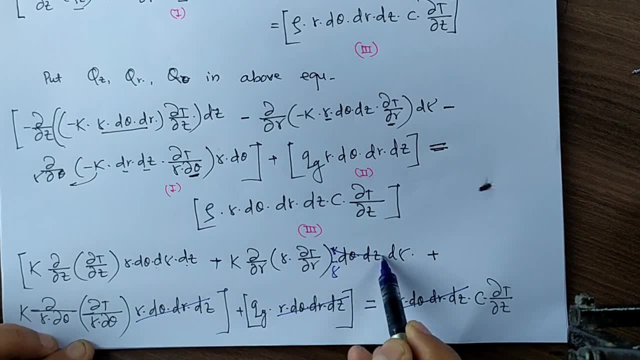 above and downside r, and then this multiply r d theta dz will get cancelled. r d theta dz will cancel. 1 upon r will be added here. 1 upon r will be because here r was not available and that i have to make it cancelled, so that what we have done is r by r, we have multiplied, so r d theta. 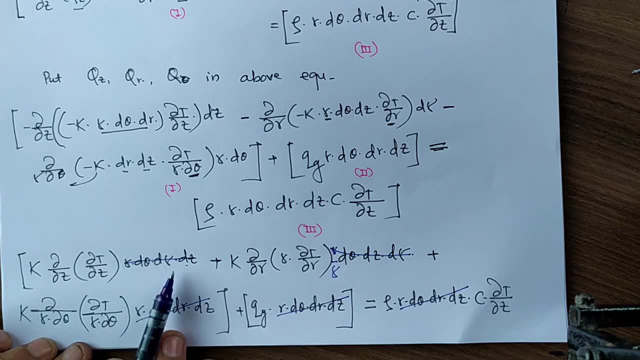 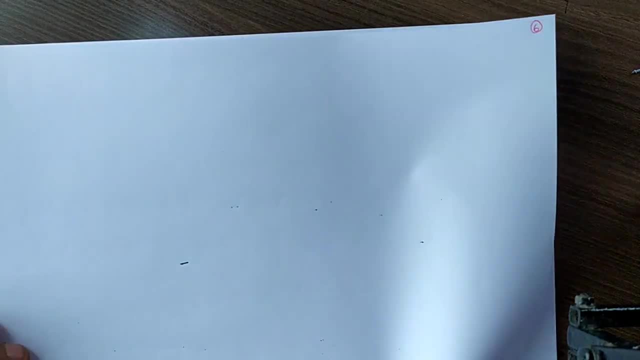 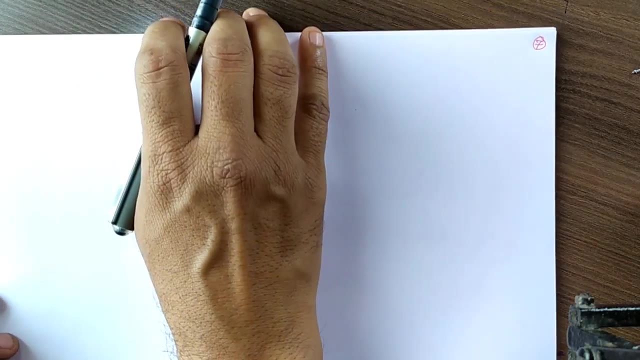 dz is get cancelled. so, from all over r d r d theta dr dz is get cancelled. now let's say further simplification. let's say this: further simplification. okay, so what says further simplification? i will write the above equation. let me show you this equation for your reference. 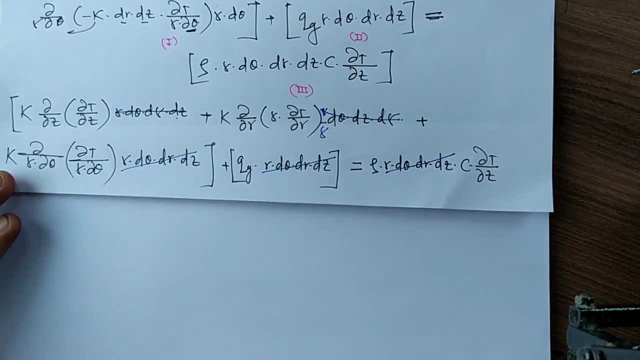 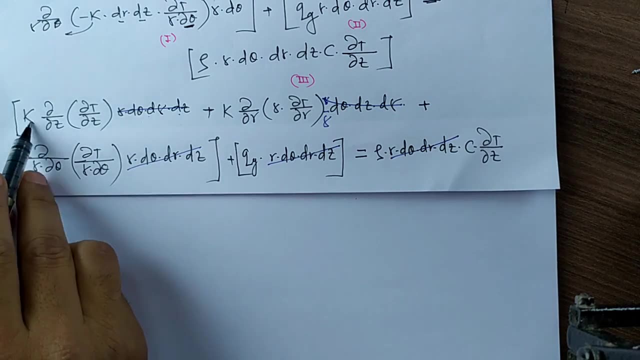 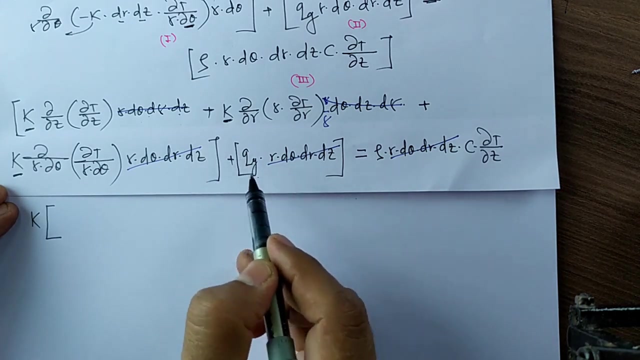 okay, this is the equation. this is the equation now, k, k and k. i will take k outside, this k, this k and this k. from this also, i will take k outside. if 1 k goes outside, k will be denominator added. okay, so then this daba by daba z and this multiplication, i will do it, so it will. 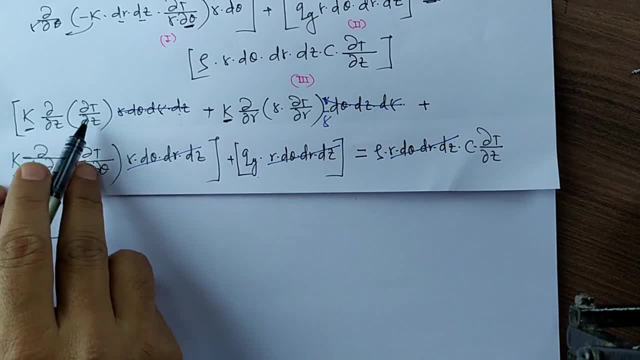 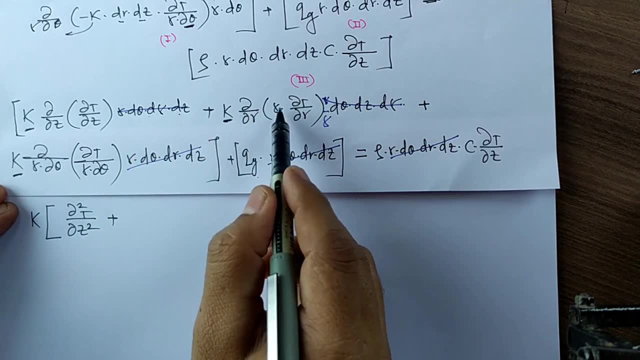 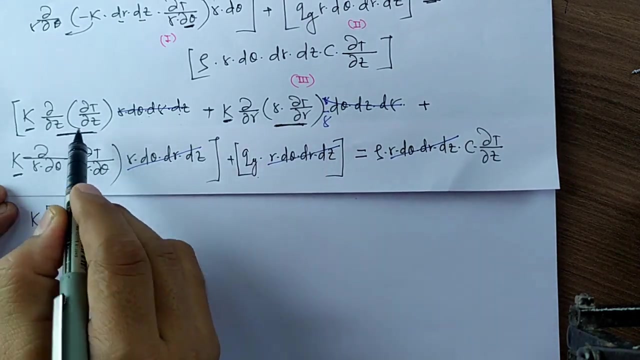 become daba square t, daba z square, daba square t, daba z square plus k has already gone outside. this daba upon daba r r, daba t by daba r this. here we have to use uv rule here. Here we have done direct multiplication, but here we cannot use it, so I have to go with. 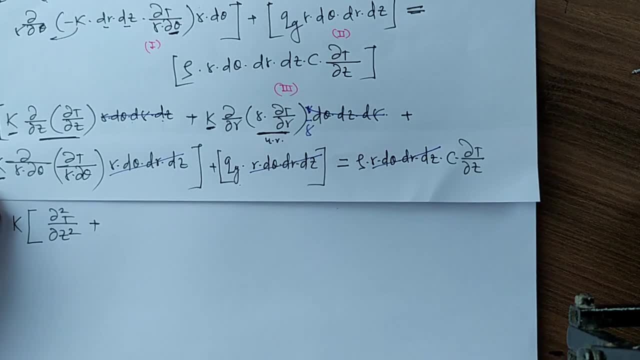 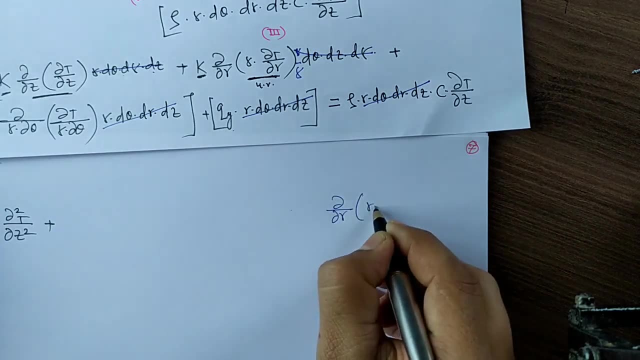 uv rule. So what says uv rule? Let me show you on the side, I will show you here that daba upon daba r r, daba t by daba. That's the equation. So this is u and this is v. 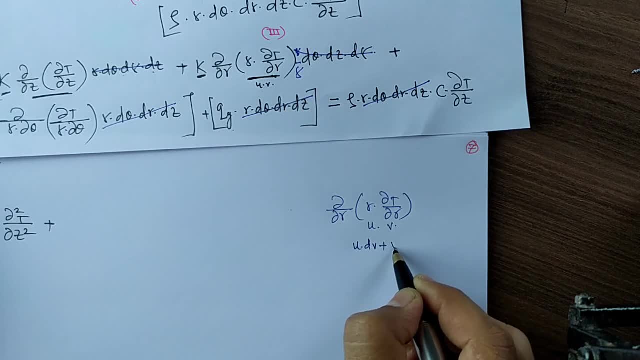 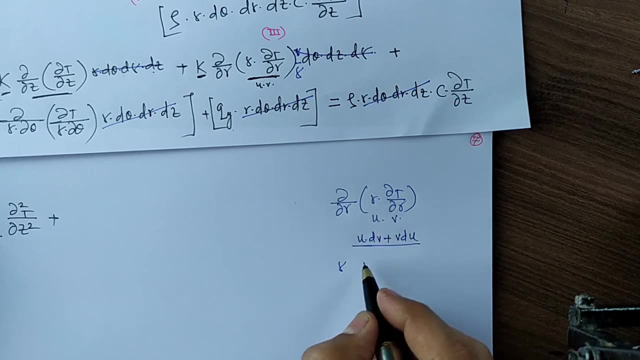 So general derivative is u dv plus v du. That's the equation. We have got it. So now, what is u? u is r, u is r dv. dv is what daba square, t daba r square. So derivative of this, with respect. 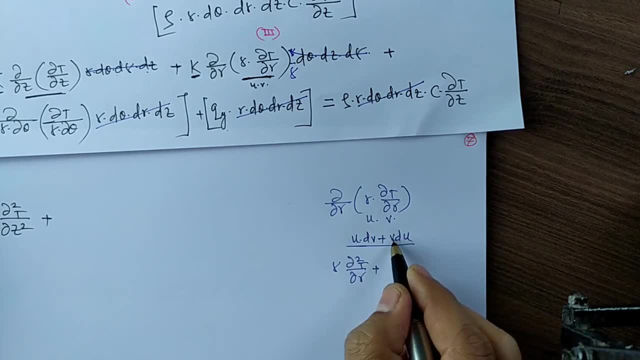 to r, it will become daba square t, daba r square plus v. What is v? v is daba t by daba r as it is, and du Derivative of r with respect to r will become 1.. So what we have got. equation: r daba. 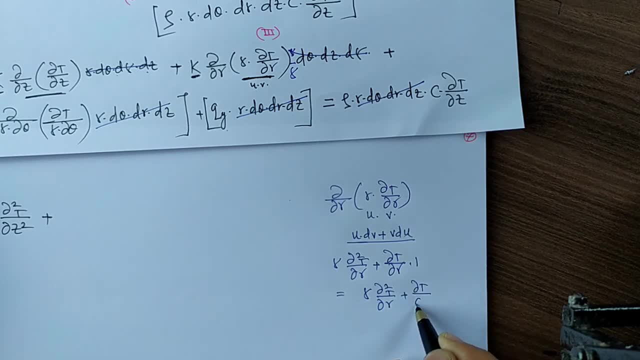 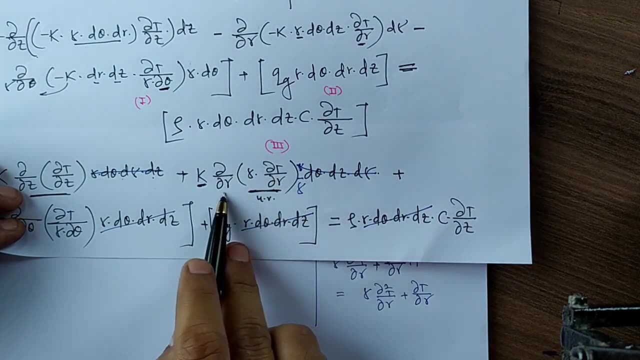 square t upon daba r plus daba t by daba r. That's the equation we have got. For what? For this one, daba by daba r, daba t by daba r. For, instead of this, what I am going to write, I am going to write this one. 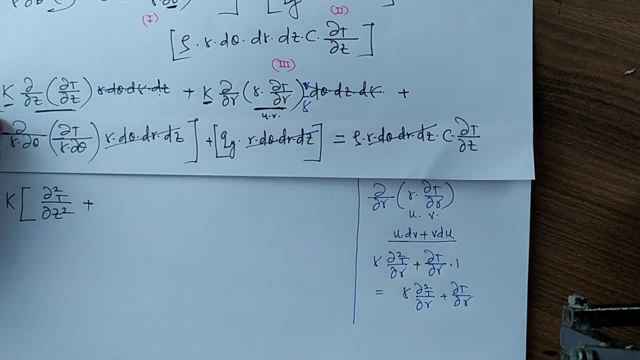 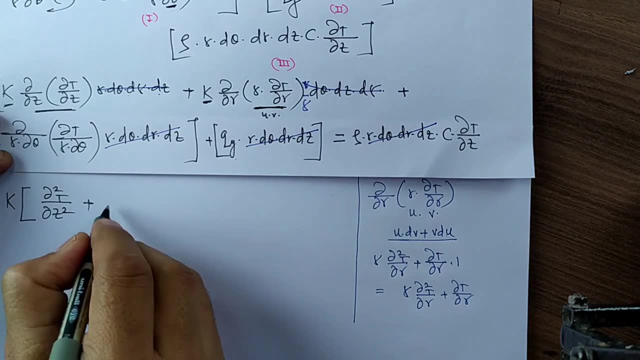 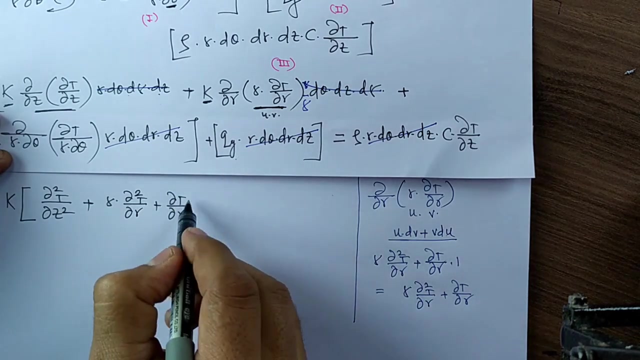 Okay, So we have done it Derivative, So let me put over here. Let me put over here- I hope you are getting. So k is already gone outside- and derivative of this. what we have written is r daba square t daba r plus daba t by daba r. This whole multiplied by r is present. 1 upon r is. 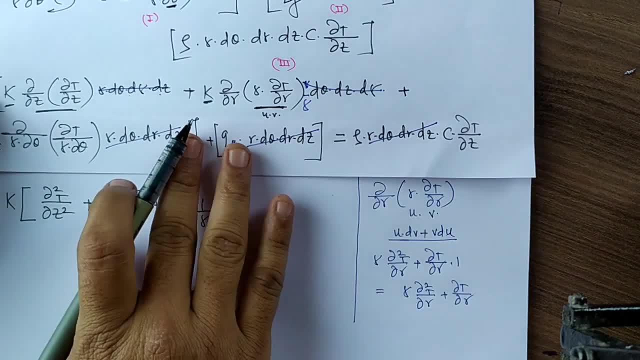 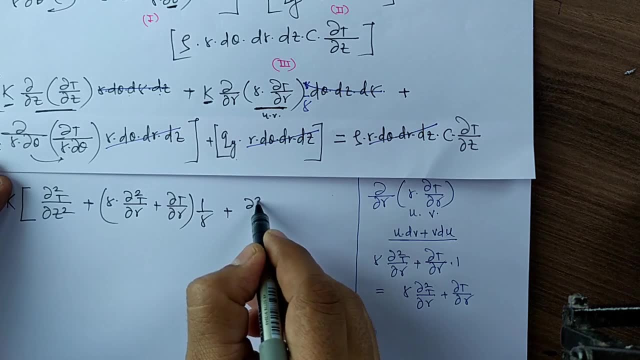 present over here. Right, That you have to remember. Plus Plus this. What is this? k has already gone outside. This multiply inside, So it will become daba square t? r? r will become r? square, Daba square, theta. Okay, That's what, we have got it. Okay, And that's what. 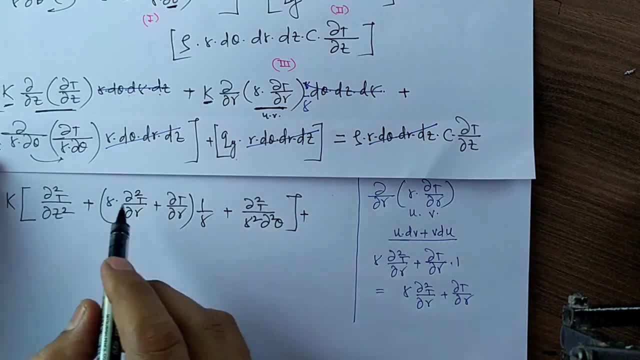 part number 1.. For part number 2, it will become q g by k. Why it will become q g by k? Because this consider that the k is taken outside from all left side. This k is taken outside from all left side. 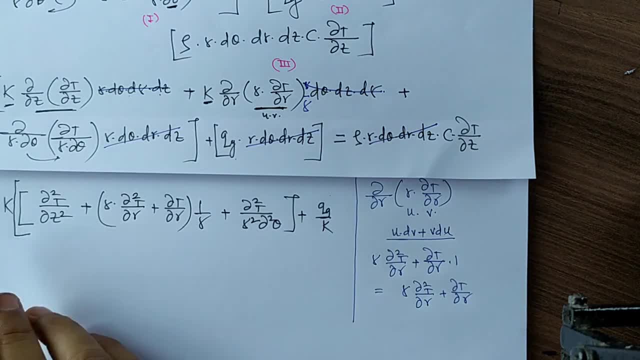 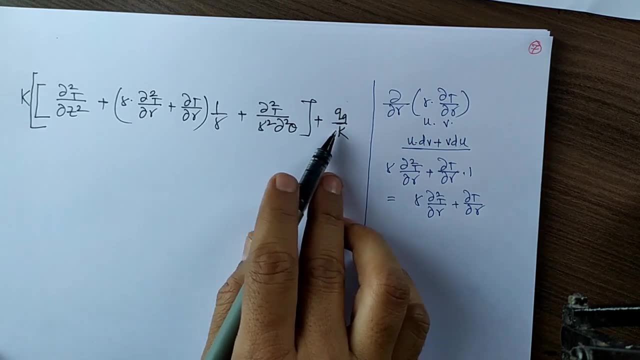 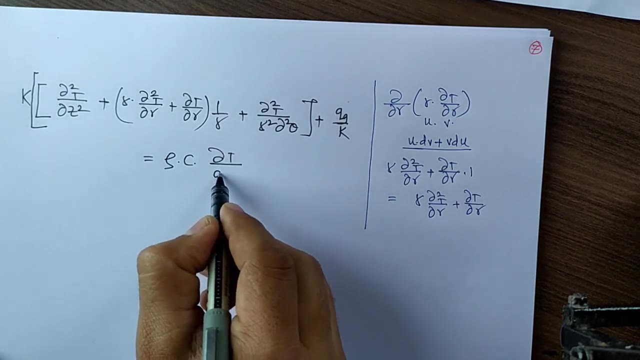 k is taken outside. So here, as on the left side, we are not having, We are not having the k, So it will be added on the denominator Is equal to. Is equal to what The right side term Here Rho c dou t by dou t. 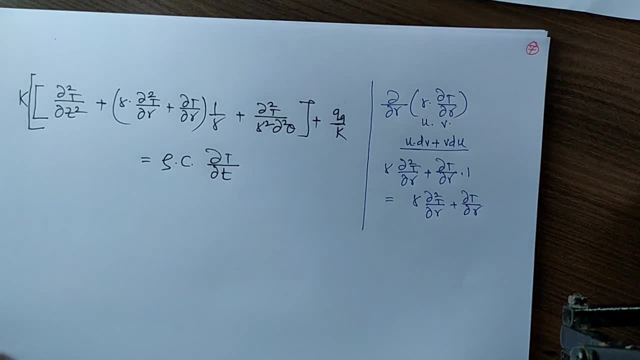 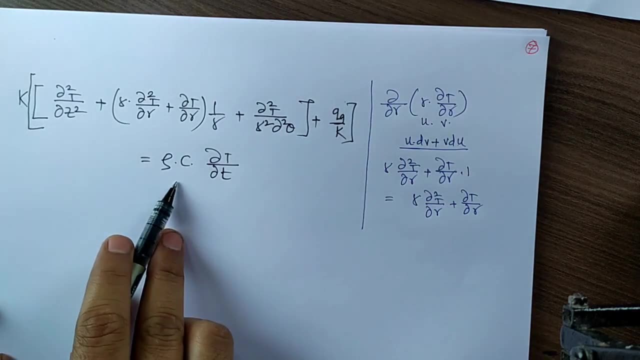 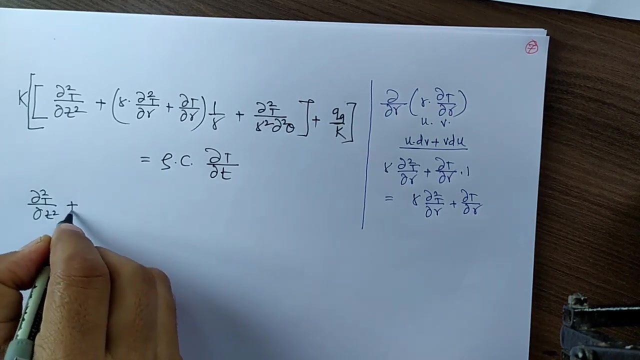 That's the equation, We have got it. That's the equation, We have got it now. Now, this k, This k which we have taken, that we will divide on downsides, so the equation will become equation will get: daba square t, daba z square, plus here r is. 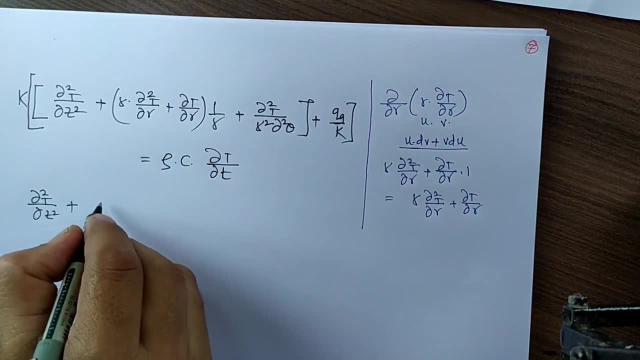 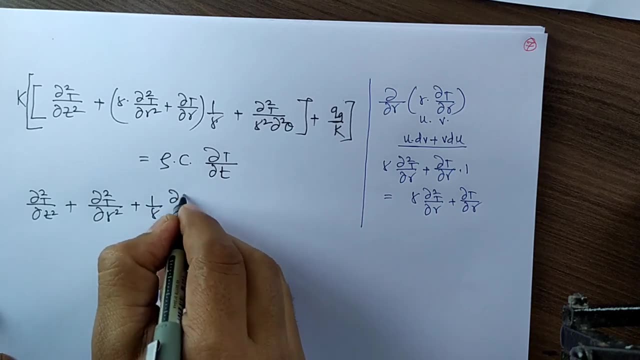 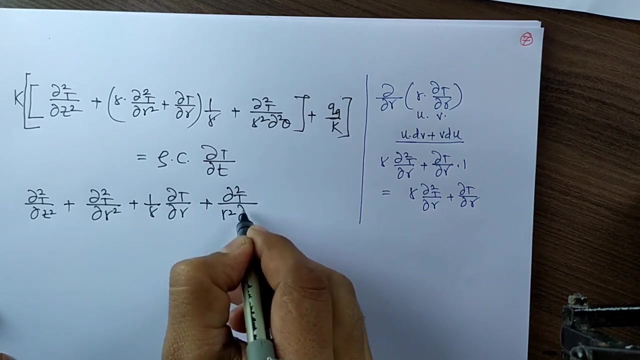 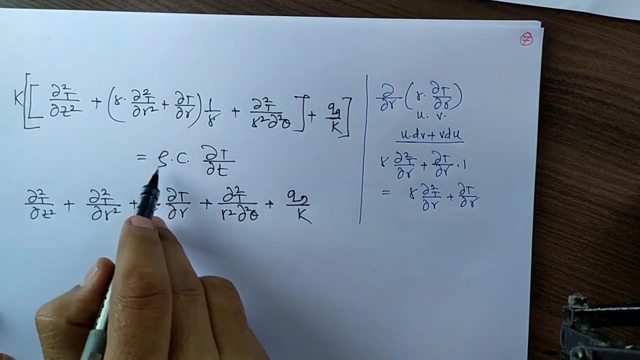 multiplied inside. so if r is multiplied inside r and r will get cancelled. so dou square t, dou r square plus 1 r will be added here. so 1 upon r, dou t by dou r plus daba square t, r square, daba square theta, plus q, g by k. this k comes on this side, so equal to rho c by k. this has came on right. 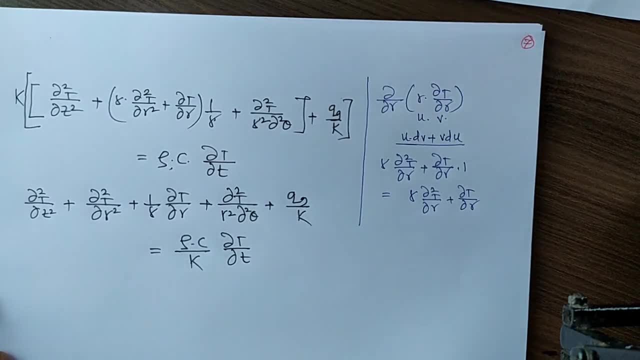 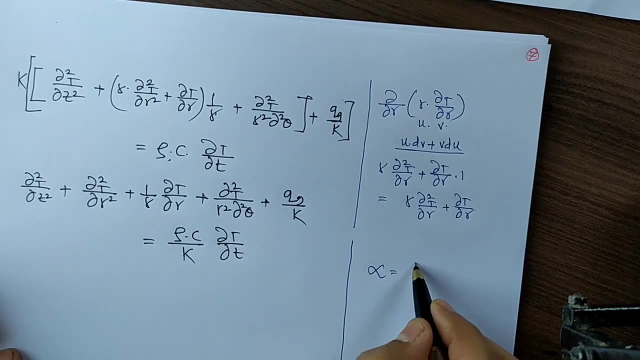 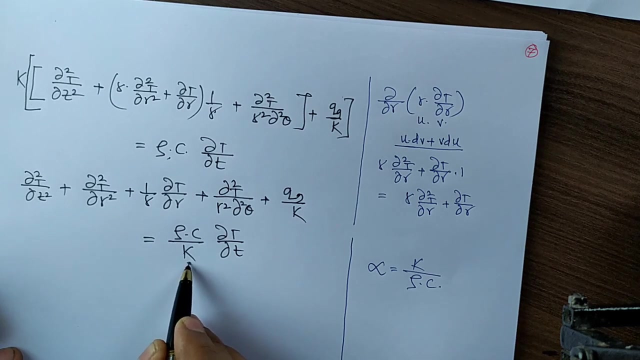 side, dou t by dou t. that's what equation we have got now here. one more simplification is required. we know that thermal diffusivity alpha, thermal diffusivity alpha, is k by rho c. thermal diffusivity alpha is k by rho c. so here rho c by k, so i can put 1 upon alpha. 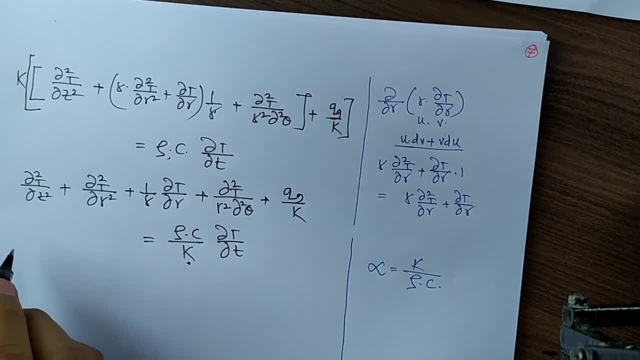 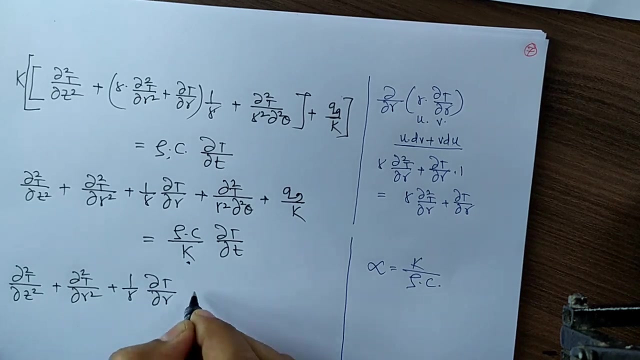 you, i can put 1 upon alpha and i will get a final equation. so the final equation will become daba square t, daba z square, plus other term i am putting as it is: daba square t daba r square plus 1 upon r daba t upon daba r plus daba square t r square daba. 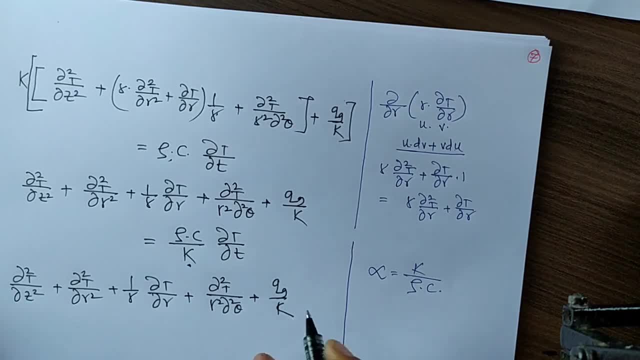 square theta plus q, g by k is equal to. this will become 1 upon alpha into dou t upon dou t. okay, so this is what we have got, a final equation, and is called as what heat conduction equation for cylindrical coordinates. thank you very much.